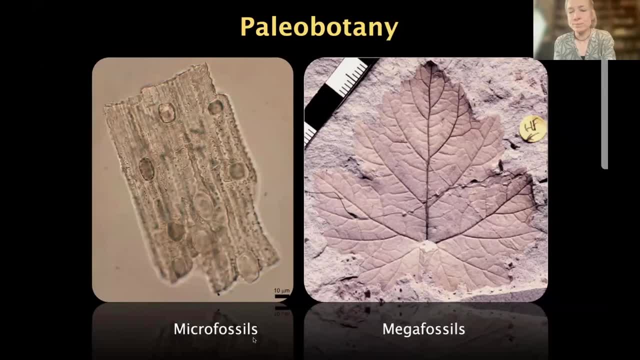 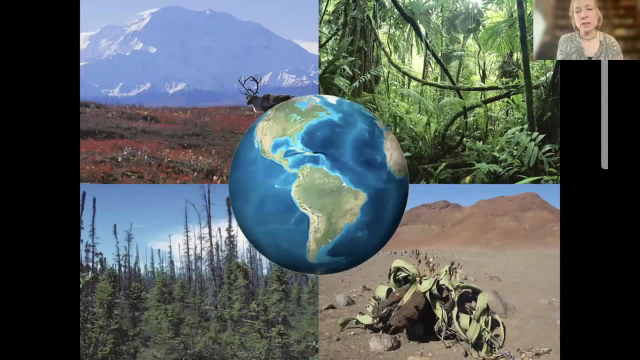 mainly going to be focusing on work using these microfossils. So, as again was said in my lab, we're broadly interested in the role that plants have played in the evolution of terrestrial ecosystems through geologic time, so through the皆-philosophical. 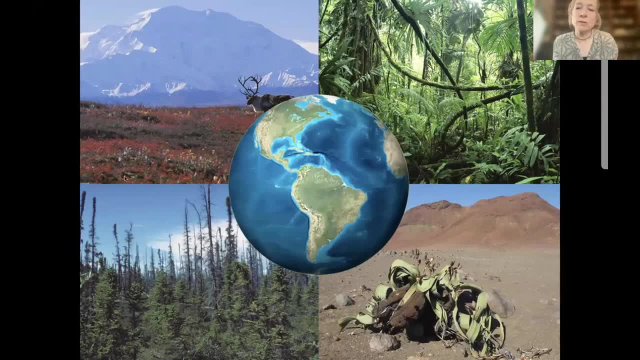 yeah, millions of years. and how we arrived at these all this diversity of ecosystems that we see around us today, how that was driven by changes in the abiotic environment, So climate, the atmosphere, how continents have moved and also how that influences and turn other organisms on Earth. 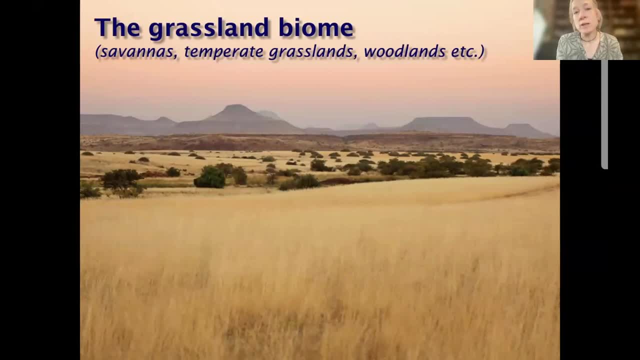 We have focused a lot on the evolution of a particular set of ecosystems in the so-called grassland biome. So this is savannas, temperate grasslands, woodlands and so on. So when I talk about grassy environments, I mean all of those things, unless I specify something more detailed. 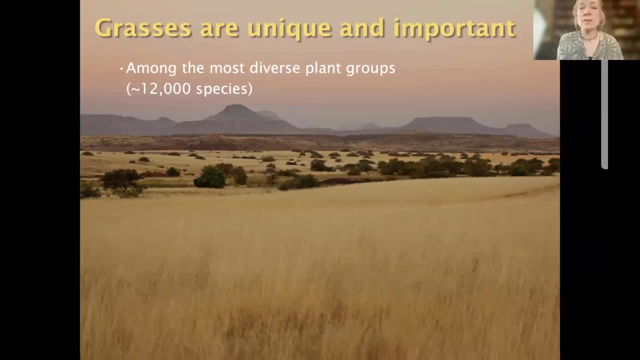 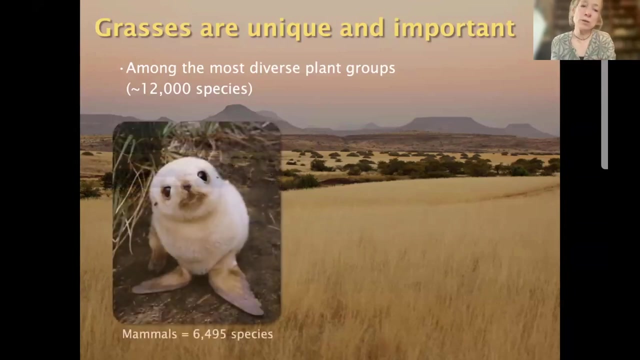 And why are we so interested in grasses and grasslands? Well, it is because grasses are unique and important. They are the fourth most speciose plant group on earth today, or plant family, I should say, with about 12,000 species, And just to put that in context, 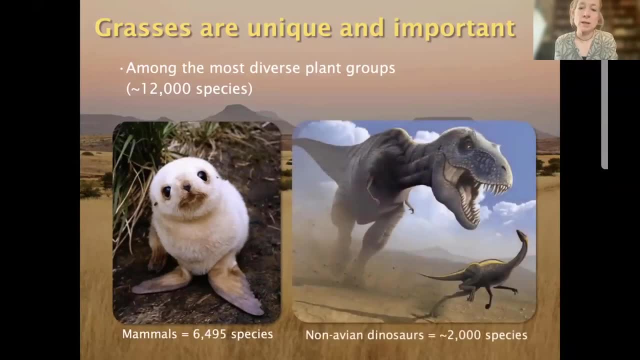 living mammals today are about 6,500 species, And I don't know if this has been updated, but the number of non-avian dinosaurs recognized in the fossil record is about 2,000.. So a lot more of grasses than any of these charismatic organisms, And they also have very diverse. 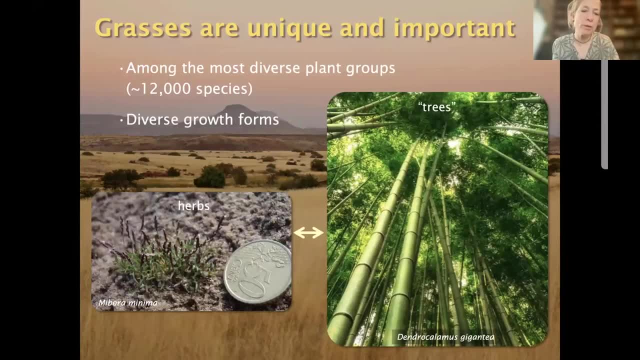 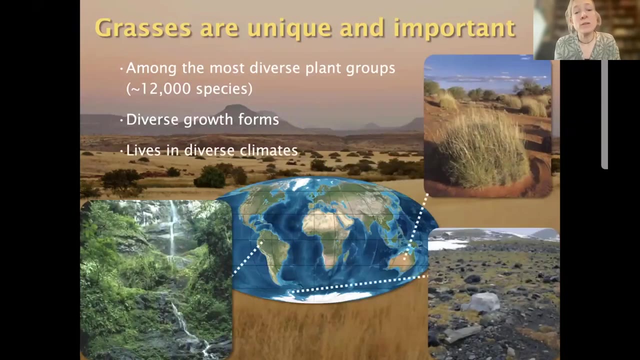 growth forms. So everything from a minute herb here, mybora on the left, to giant tree-like bamboos that can be up to 100 feet sometimes, So very large Grasses also live in very diverse climates, So everywhere, from the tropical rainforest to hot. 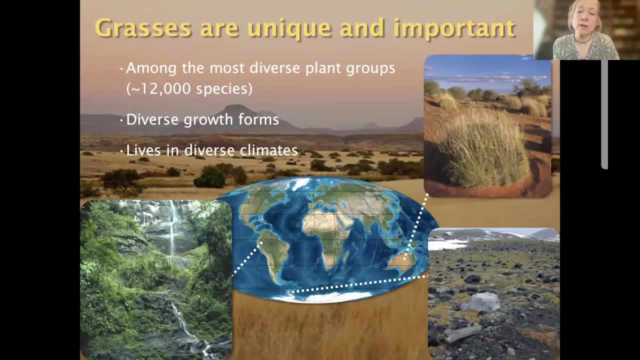 and cold deserts And, in fact, a grass. that's one of the few vascular plants that are now permanently living on Antarctica, which, of course, is a sign that climate warming is really happening. So not a very fun thing, but it does show. 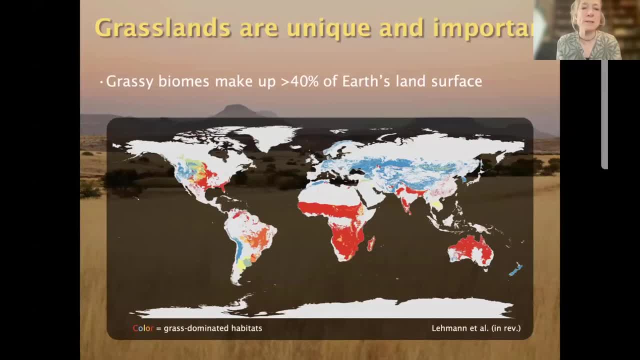 how versatile grasses are in terms of their climate space. Grasslands are also very unique and important, So grassy biomes are incredibly important, making up over 40% of earth's land surface, And you can see grassy biomes here marked in different colors on this map. 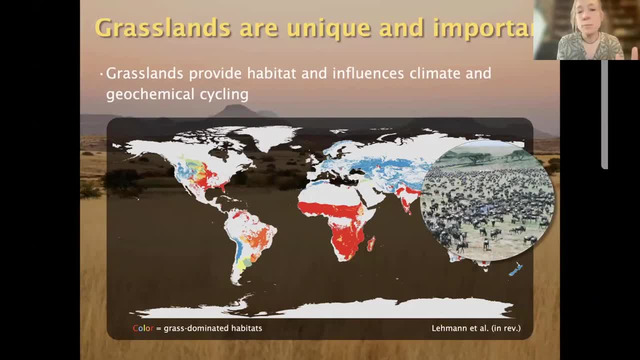 And and they, they provide some really important things for us and other organisms. So over a billion human beings live in grasslands, and many, many millions of other animals as well, And they have an influence on climate because they absorb sunlight in a different way compared to forests or ice. 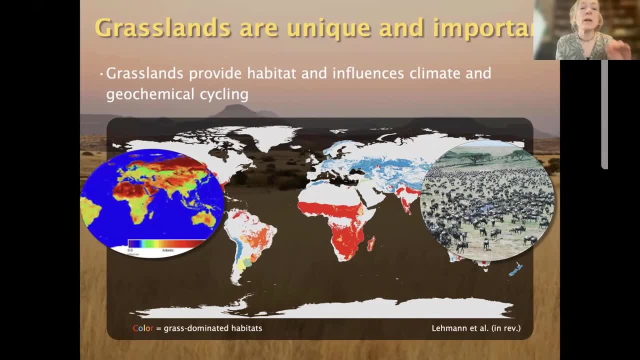 So they influence the distribution of heat that way on earth And they also have a different relationship with water Compared to forests and deserts. So they influence how water is distributed on earth And also they play a big role in geochemical cycling, So how carbon is moving through the. 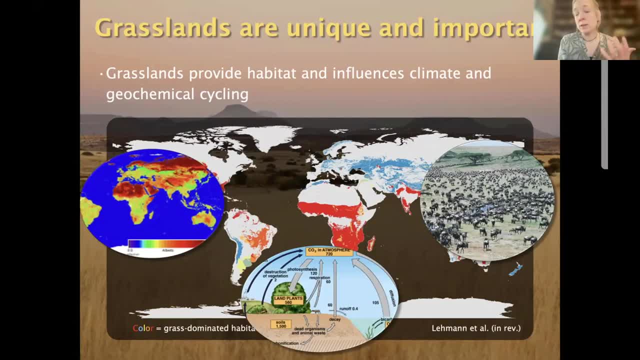 environment, So how it gets fixed, how it gets stored, And this in turn has a feedback and sort of influence on climate as well, because CO2, where the source of carbon, is, of course, a greenhouse gas So important for earth in general. 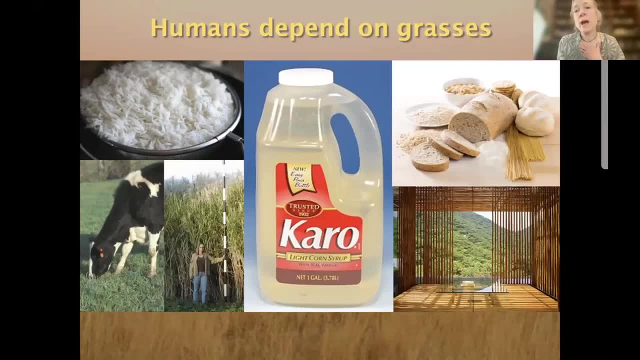 but also important for us humans. specifically, we have grasses were one of the earliest crops to be domesticated, some 10, 12,000 years ago on different continents, And it's still the most that make up the largest part of what we eat today, including corn syrup here in in North America And also 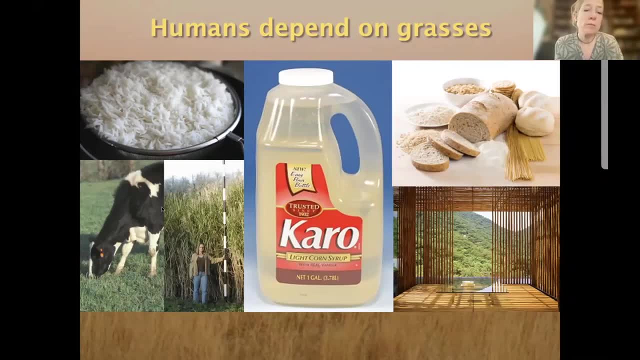 important building material in the form of bamboo, Most of what our domesticated animals eat, but what they don't know. And here's an example of a grass as Biofuel switchgrass. Also, many of our most important weeds are grasses, so it's not all good. 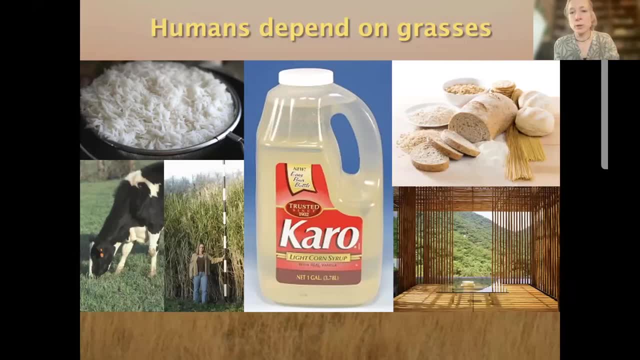 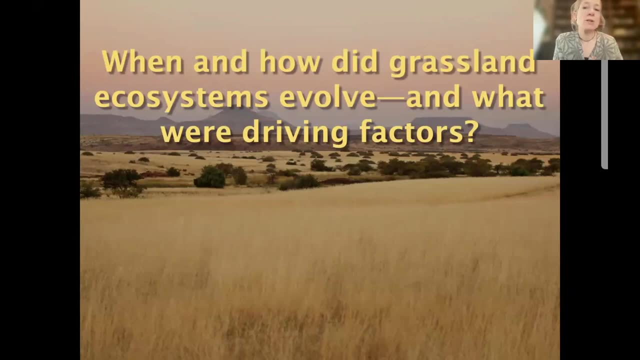 But it does mean that grasses play a really important part in our lives as humans, And so, given their importance today, paleontologists and evolutionary biologists have long been interested in when and how grassland ecosystems evolved. they're so important today. 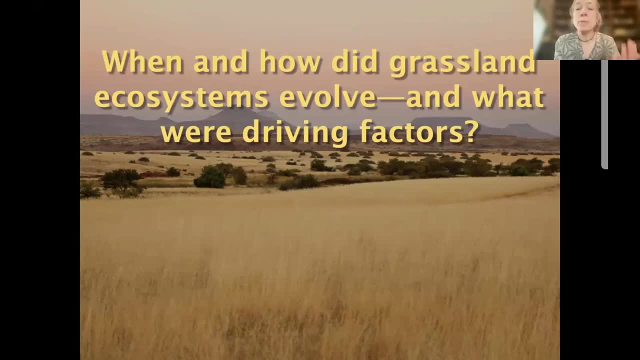 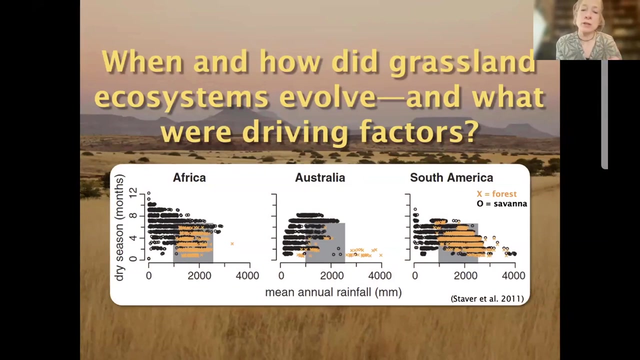 they were not around when the dinosaurs ruled the earth, So it happened very recently. So how and when did it happen and what were the driving factors? And this is not just a sort of a curiosity for knowing earth's history, but it actually plays a fundamental part in understanding how. 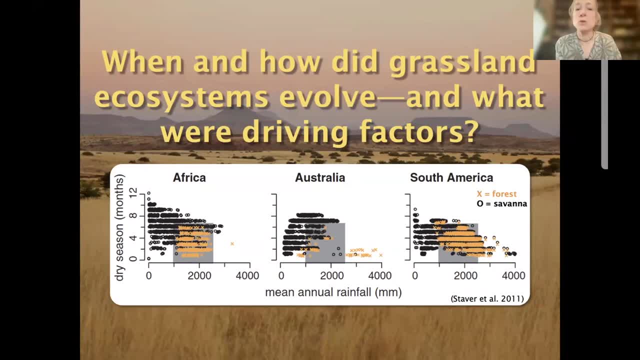 grassland ecosystems function today and how they might change in the future. So to give an example of that, here's the distribution of savannas as black O's here, versus forests as orange X's in climate space across continents. So on the X-axis we have mean annual rainfall on these. 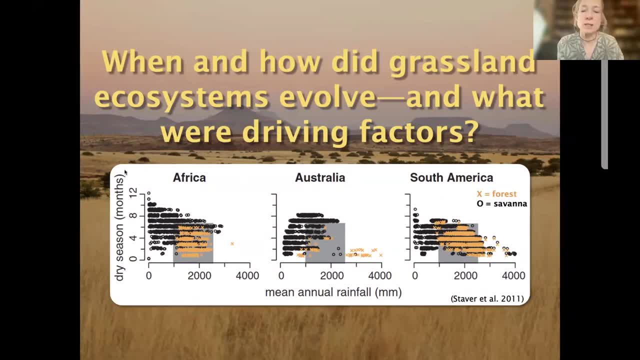 different continents. On the Y-axis we have the length of the dry season And you can see that across continents we see similarities in the distribution of these different vegetation types in climate space, but also some differences. So, generally speaking, forests tend to be at higher rainfall, but there are also some big differences here, And those 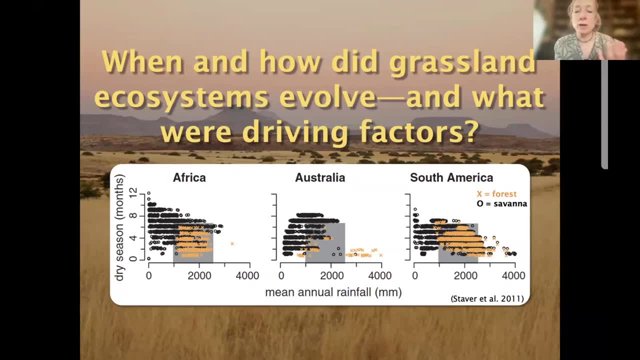 differences have been suggested, or researchers have suggested that that relates to the kind of bedrock that's there, So the types of rocks that form the landscape where these different vegetation types are growing, the kinds of trees that evolved in these different continents, the kinds of animals that occupy these different continents. So in other words, 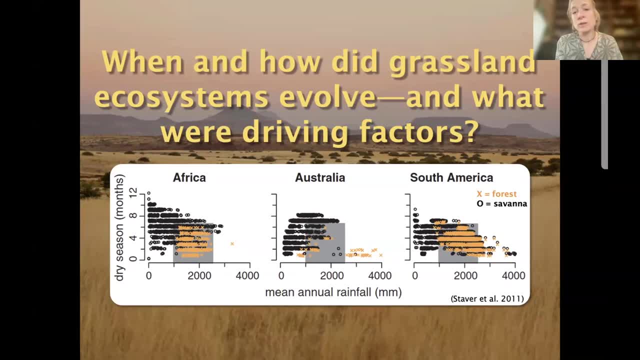 it depends on the history of those biomes on these different continents. History matters, So history matters for how these vegetation types are responding today in climate space and likely also how they will respond in the future. So really important to understand at this point in time when we are 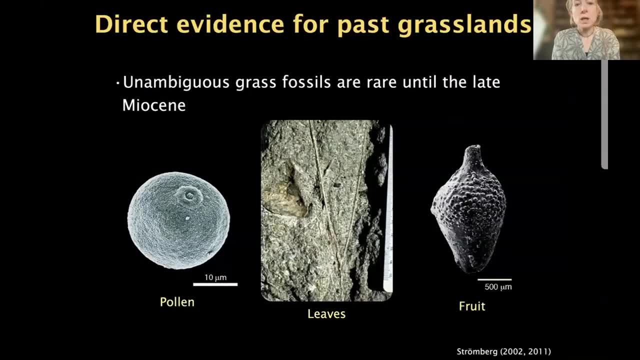 seeing major climate changes happening because of humans. Okay, so we're interested in reconstructing these past grasslands. What kind of evidence, What can we use? So people in the past have looked at, for example, grass pollen, putative grass. 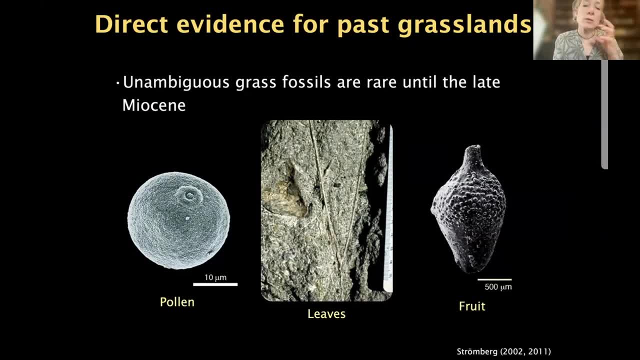 leaves and grass, fruits in the fossil record, And it turns out that those kinds of fossils are rather rare until the late Miocene, And the ones we have are for the most part ambiguous. So leaves are very hard to interpret without preservation of anatomy, so cells And so for the most part we can just say: 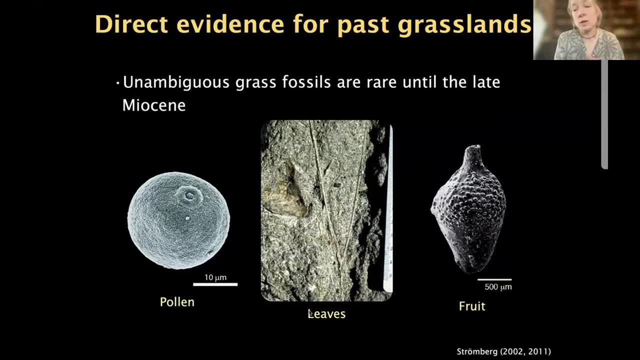 it looks kind of like a grass leaf, but it could also be a sedge or a cattail or some other monocot. And then grass pollen are very similar to pollen of their closest relatives, So we can't know for sure if we're looking at grasses all the time. So instead people, when they want to reconstruct. 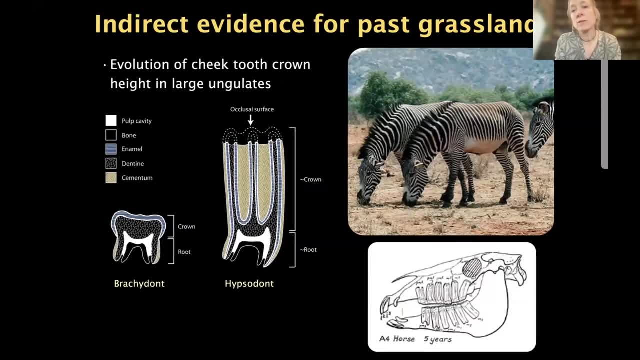 grasslands have looked at indirect lines of evidence, in particular at fossil faunas. So there are animals today, like these zebras that we know live and feed in grasslands and they have particular functional traits, So shapes and morphologies that relate to their function And, in particular, people have. 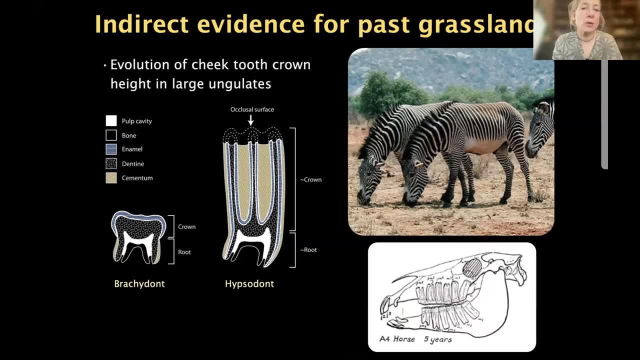 looked at the evolution of cheek teeth, how their crown height has changed, has evolved within large hoof mammals or ungulates. So here we have a human tooth which has a very short crown- That's called Brachydont. And here we have a horse tooth that has a very tall crown, That's called. 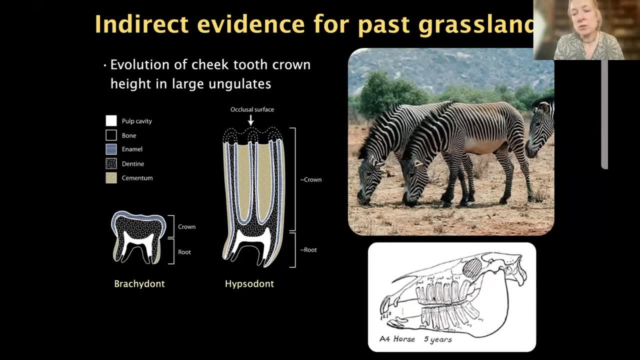 Hypsodont, And we have these Hypsodont cheek teeth shown in the skull of a young horse here on the right. And so what we notice today. when we look at ecosystems, as I alluded to, we tend to see herbivores with these Hypsodont teeth in grasslands and other open habitats. 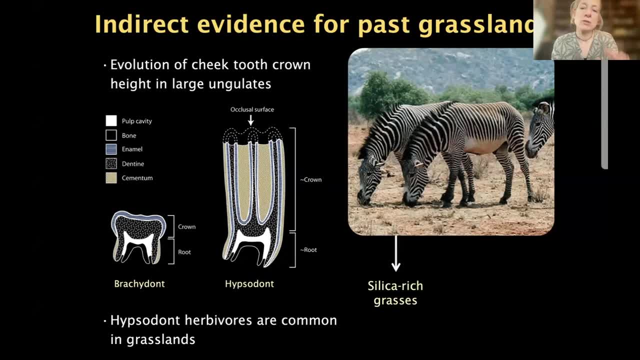 And so the assumption has always been that it is because it's a way to deal with the feeding on very abrasive food materials such as silica rich grasses, because grasses have a lot of silica in their tissues, as we'll talk about, And also because when they're feeding in low to 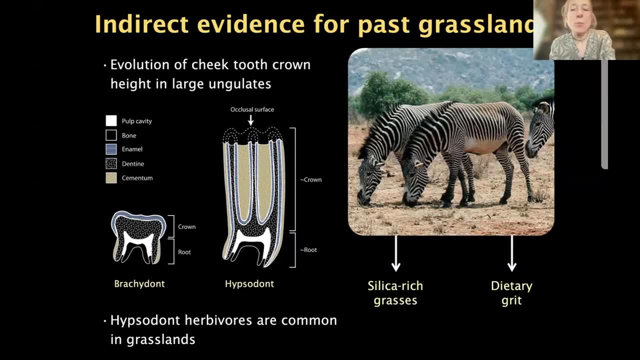 the ground or, you know, in open habitats with a lot of bare soil, they tend to get a lot of dust and soil in their mouth, and that also wears their teeth, And so the significance of this is that these, the silica in the grasses, and this grit wears down the teeth. 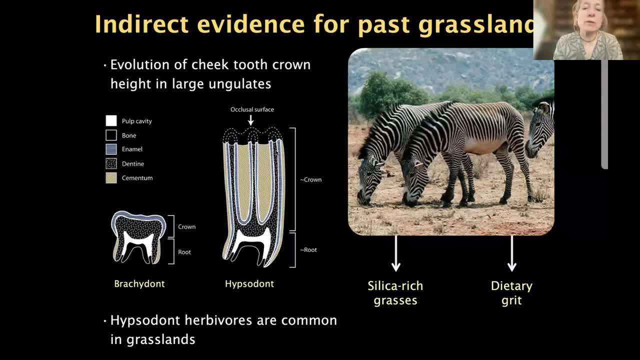 And that means that the more crown you have, the longer you can live, the longer it's a functional life of the tooth. So it is an advantage in those grasslands And the assumption therefore has been made that evolving these tall tooth crowns was an adaptation to feeding in grasslands, either on grasses or grit. 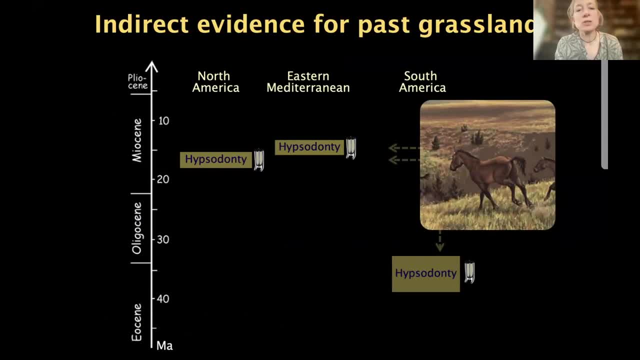 And using this line of evidence, paleontologists have looked at: when did Hypsodontae when in time? when did Hypsodont have the ability to feed on grasslands? When did Hypsodont have the ability to feed on grasslands? When did Hypsodont have the ability to feed on grasslands? When in time? 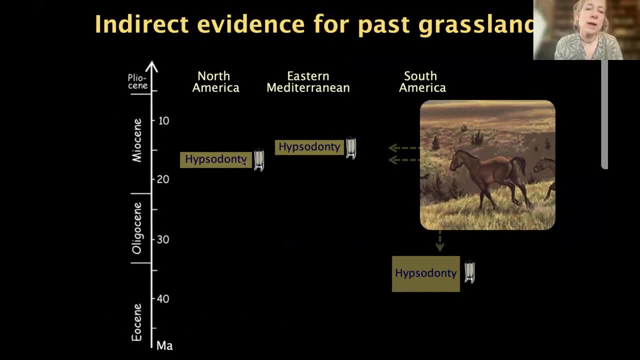 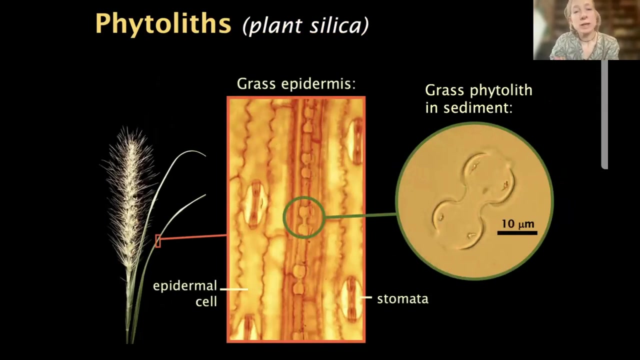 did Hypsodontae show up on different continents And use that as a mark, as a signal that at that time is when we must have started to see grasslands spreading and that those animals evolved Hypsodont teeth in response to that? In my lab we wanted to test this by looking at plant fossils. 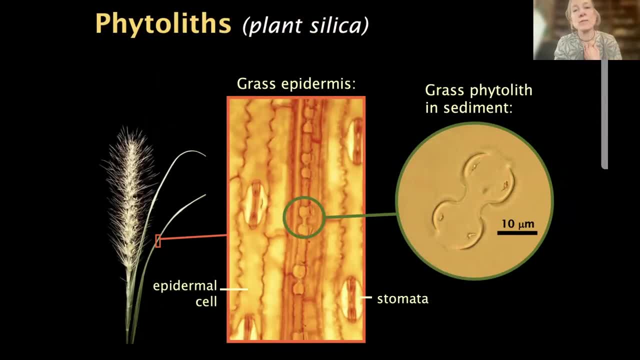 because here we have so far, we have no plant fossil evidence, And that can be easily compared to the animal evidence for the animal, indirect evidence for grasslands. So what we're using is plant silica, fossils, microscopic or phytoliths, And so what? 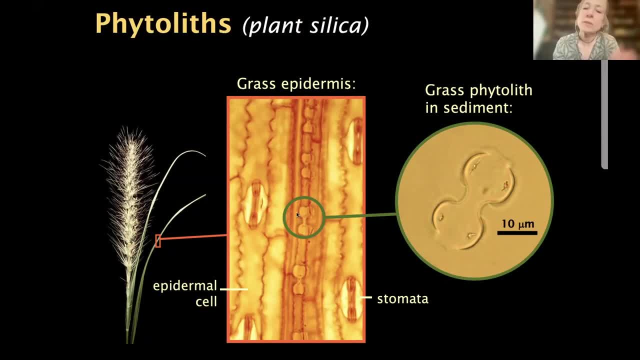 are phytoliths. They are tiny, tiny, microscopic silica bodies that form inside and around cells in living tissue. This is the outermost layer of a grass, the so-called grass epidermis, a leaf, And inside some of these cells we see these silica bodies forming. And then, when that leaf is dying or 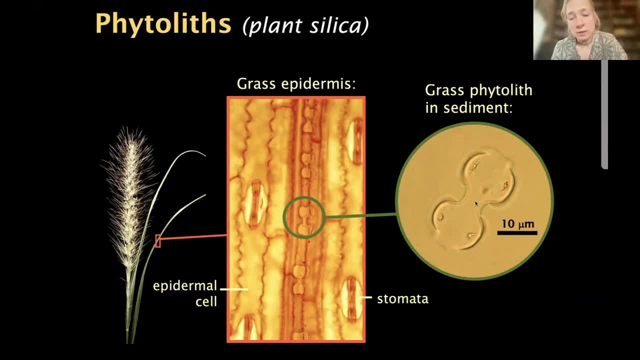 decaying. those silica bodies are left in the soil or the sediment and can stay there for a long time because it's chemically much more sort of. It's not as reactive as organic material, So it can stay there for a long time. It's also very hard. 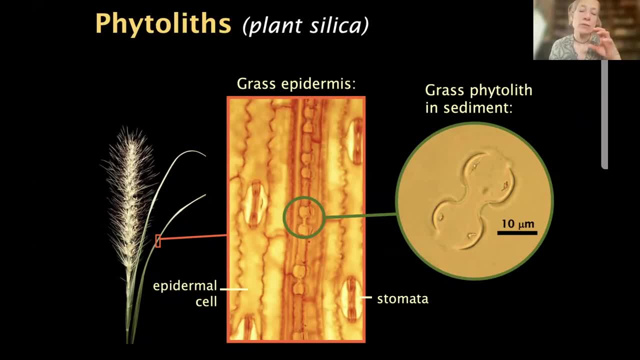 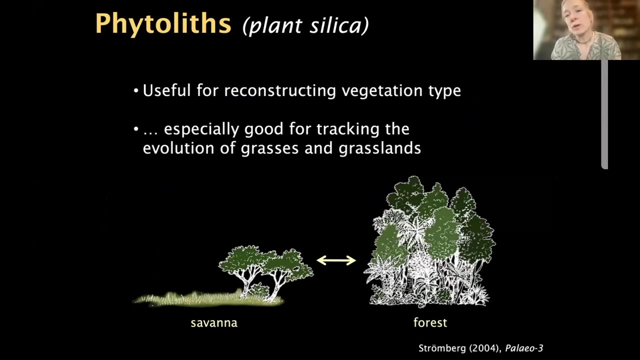 It's hard and durable. So we can use then these phytoliths that are staying in the sediment or the soil to say something about what plants were growing at that particular site. And so, if we compare phytoliths to other types of paleobotanical data, 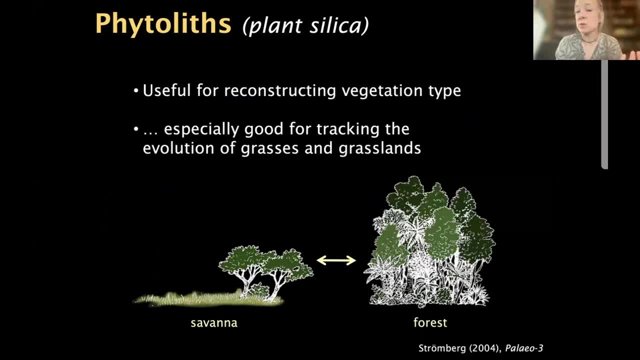 you can't get very specific information about, for example, the types of trees that were in a particular place, But we can say something about the broad vegetation types. So, whether we're looking at a Savannah or a forest- And this is of course- 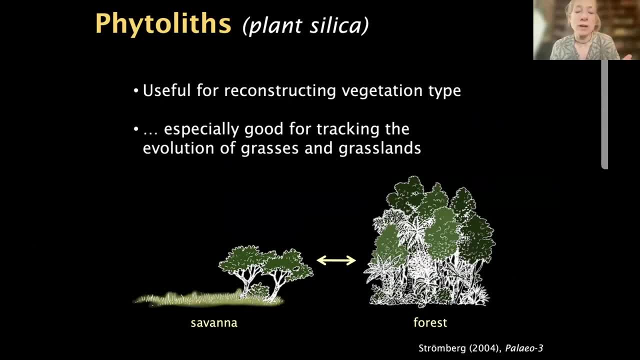 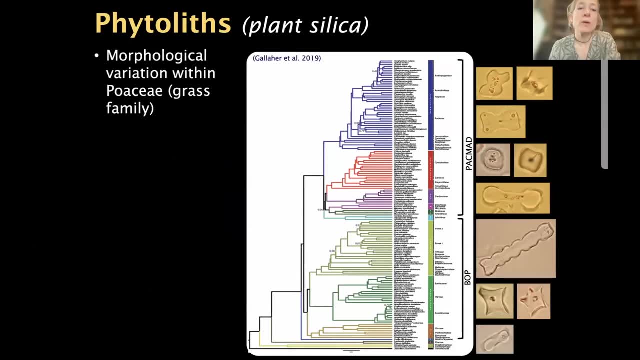 what we want to know when we're trying to reconstruct how grasses are becoming more abundant in the environment, So they're very good for that, Also within the grasses. So this is a picture here of a grass family tree, or a phylogeny as it's called, And so showing 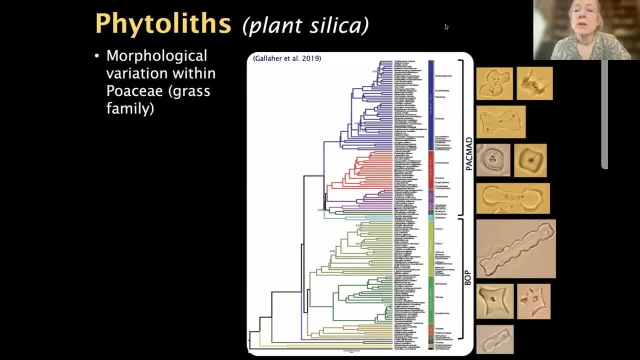 different grasses are related. We also know that there is variation in the the shape among phytoliths across the grasses And that means that we can say something. we can look at phytoliths in the fossil record grass phytoliths and say which kind of grass it came. 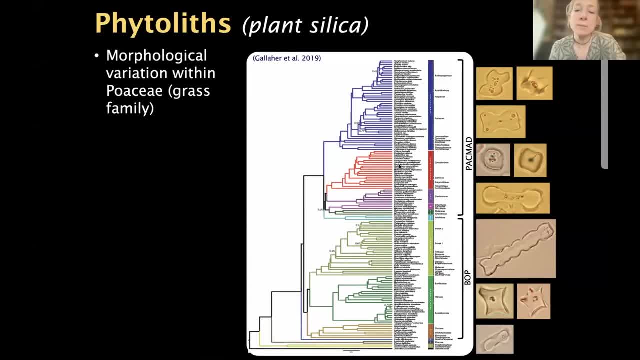 from which subgroup of grasses it came from. And this is important because, as I'll show you in a second here, different grass subgroups have different ecologies, So they can say something about ancient grass communities. what kind of grass community, what was the ecology of that? 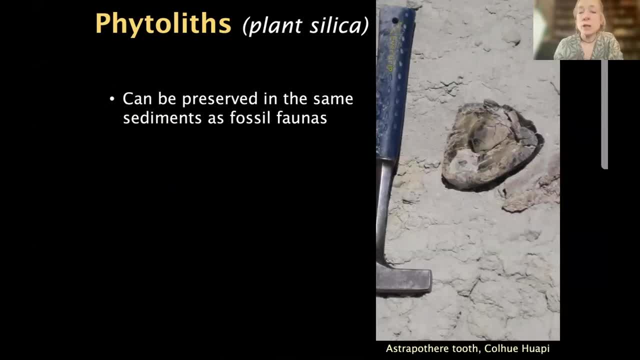 grass community. Another really cool thing about phytoliths is that they can be preserved in the same sediments as fossil faunas. And this is unique, I would say, to phytoliths, because in many of the sites where you find faunas, you don't find other types of fossil plants such as leaves. 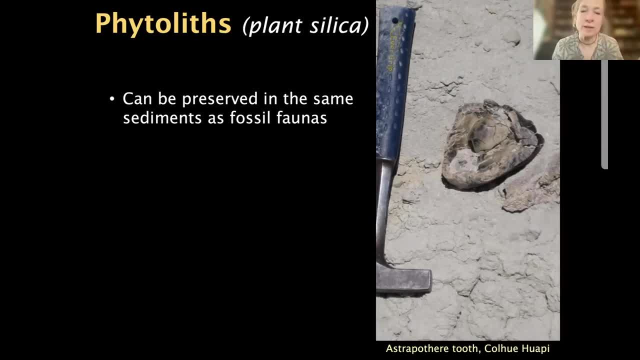 or pollen. They're often been oxidized away. So this is good because we can get a direct ecological link between floras and faunas using phytoliths for that reason, And we can capture some part of the environment that we don't see when we look at other types of fossils. potentially Okay. so 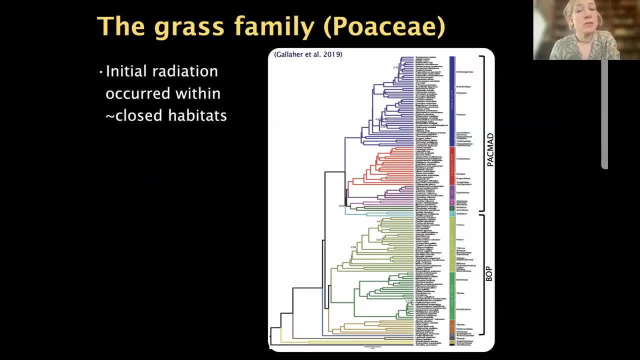 before we dive into the research, let's just familiarize. So we're all on the same page when it comes to grasses. What are they So, or what can we say about different kinds of grasses? So we know that the initial radiation 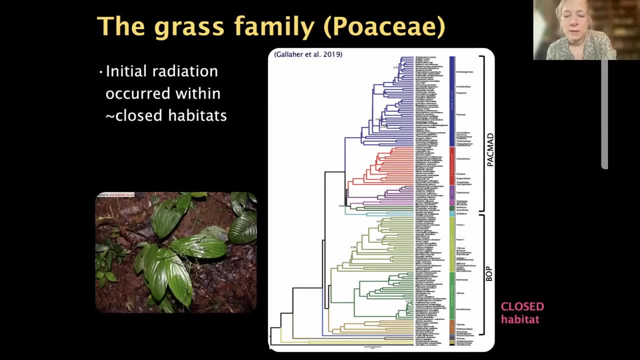 It occurred either of grasses. So if we Look down here at the bottom, the most early diverging grasses, we know that those today live in relatively close habitats, So either in the forest understory or in forest margins, And so we know that this, that they probably sort of initially 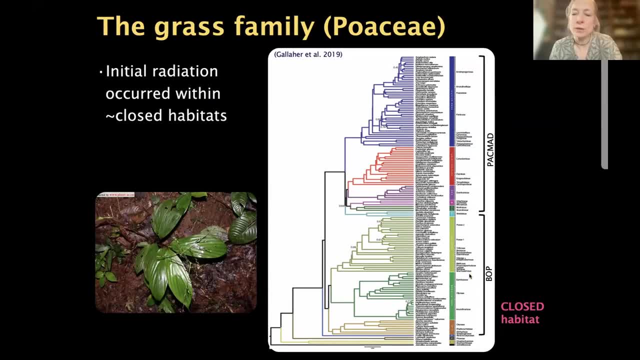 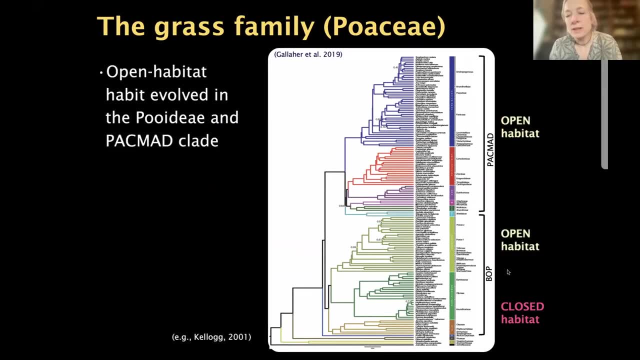 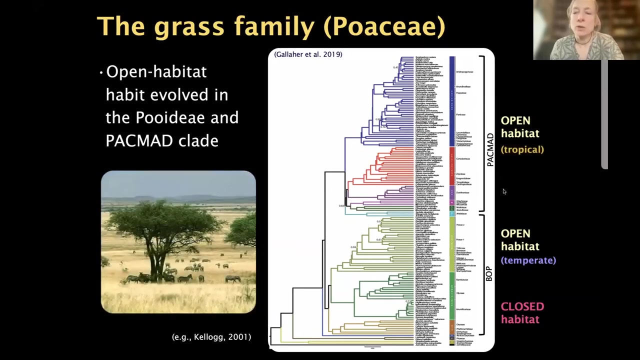 lived in in close habitats. Also, there are some groups, like bamboos, for example, that still live in close habitats. And then there two groups that independently evolved the ability to thrive in open, drier habitats. One was the cool-tempered poids here, the poidae, and one was the tropical pack mats. 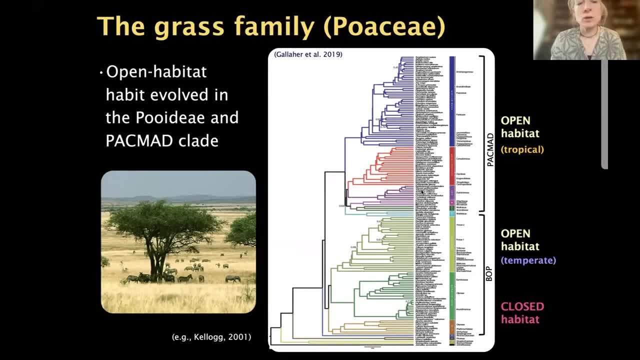 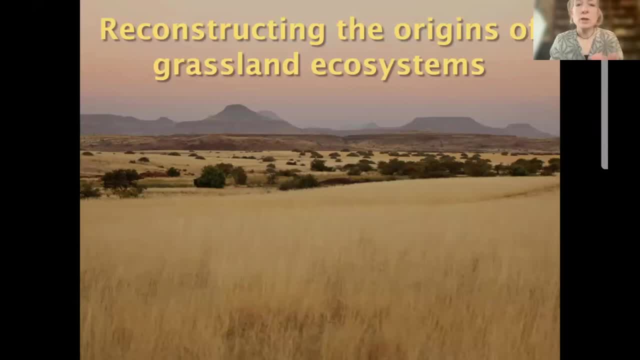 And within this pack, mats, is where we find some of our most common savanna grasses, for example, tropical grassland grasses And, okay, so using phytoliths we have. I'm going to talk about three different questions that we've been able to address in the lab. 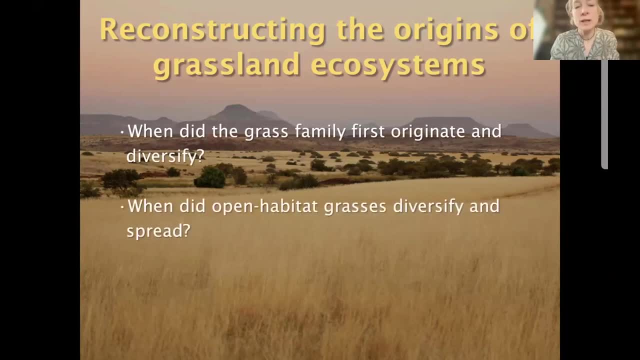 And one is: when did the grass family first originate and diversify? When did open habitat grasses diversify and spread, And how did the evolution of grasslands relate to the evolution of grass-eating herbivores, those hypsodont herbivores? 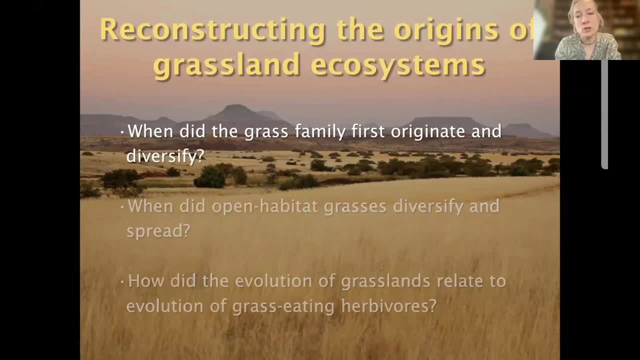 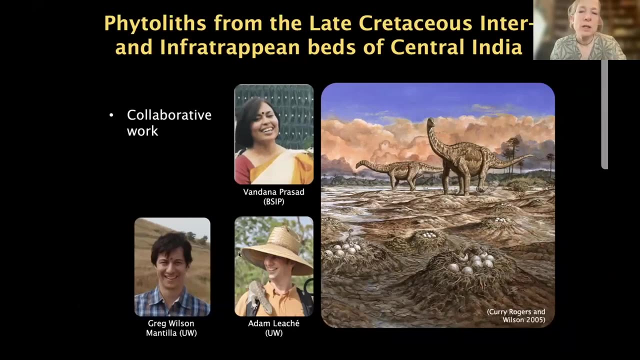 Okay, so first I'm going to talk about some work. looking at this first question, This is collaborative work with colleagues from India and elsewhere, And it's looking at phytoliths from late Cretaceous sediments in central India. So what we did was we went to some sites in central India that have been dated to 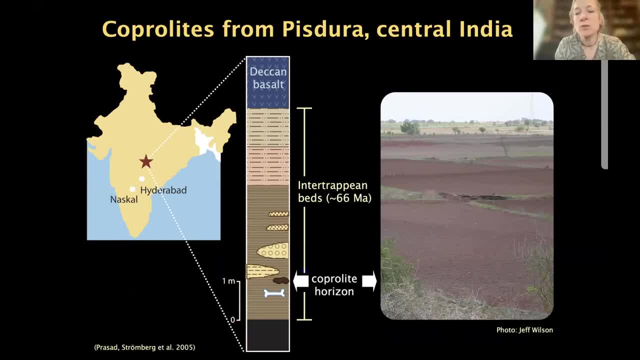 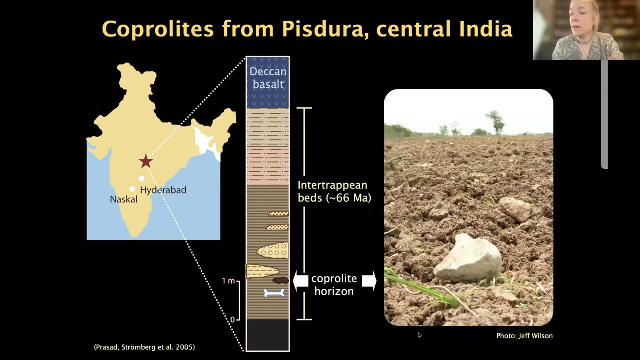 just before the extinction of the non-avian dinosaurs- about 66 to 68 million years, perhaps something like that- And in those sediments we have certain horizons And that weather out in the form of agricultural fields and where you can find dinosaur bones. 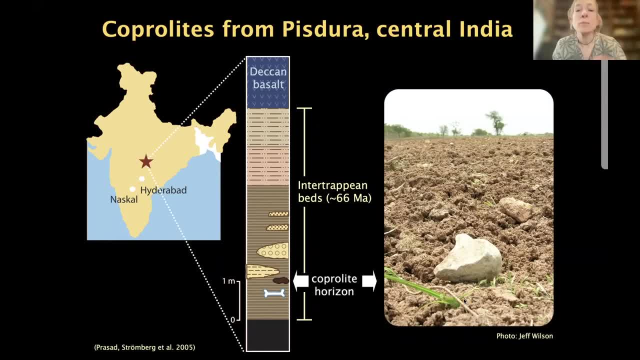 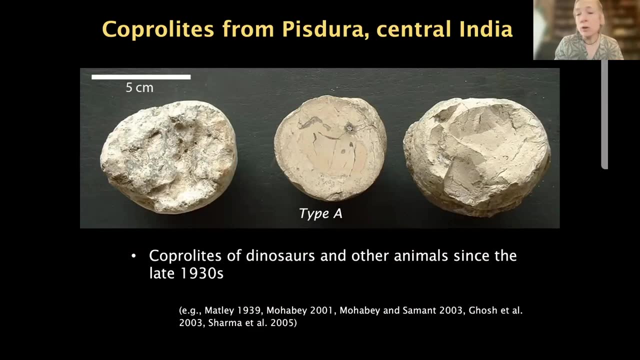 such as this one: turtle bones, all kinds of bone scraps, but also a bunch of fossilized poop, so-called coprolites, And here are some examples. Some are five to 10 centimeters in diameter, sort of blobby things, but there are all kinds. 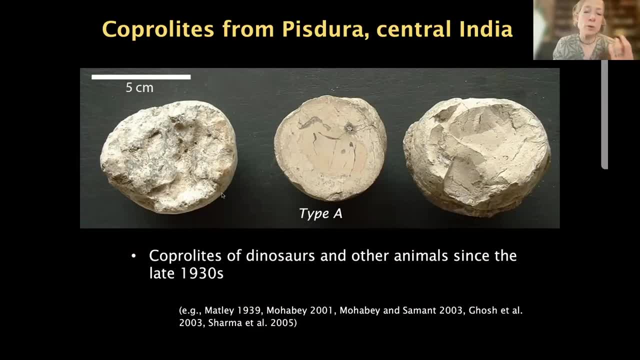 of other kinds as well. These larger ones have been most- I'm not saying they're most reasonably linked to dinosaurs or diverse dinosaurs, but these coprolites, the whole assemblage of coprolites, have been studied since the late 1930s by 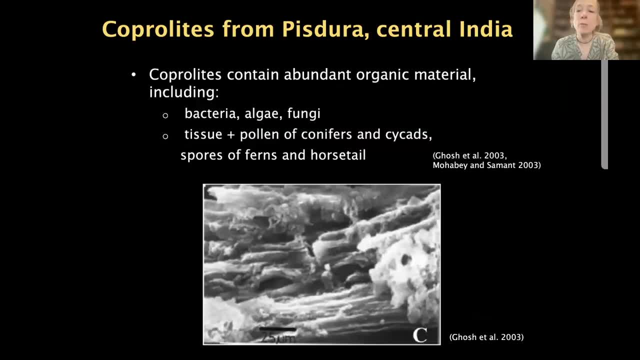 primarily Indian researchers, And what they found inside them is that they contain abundant organic material, including from bacteria, algae and fungi, but they've also found a lot of tissues and also pollen or spores from conifers. So, in particular, the most common ones are made out of coir and the most common are 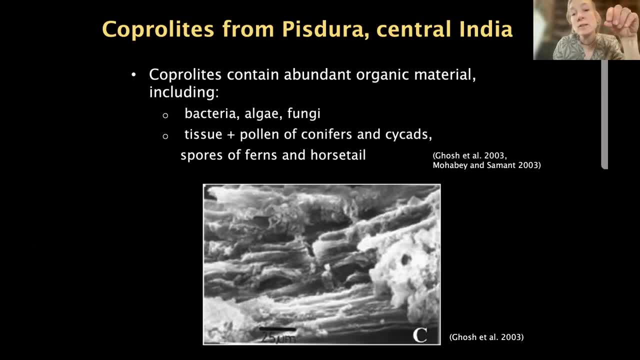 from the. So, again, the most common ones are made out of coir and the most common ones are made out of coir, and the most common ones are made out of coir and the most common ones are from the. So we took these coprolites into the lab and macerated them, basically broke them down. 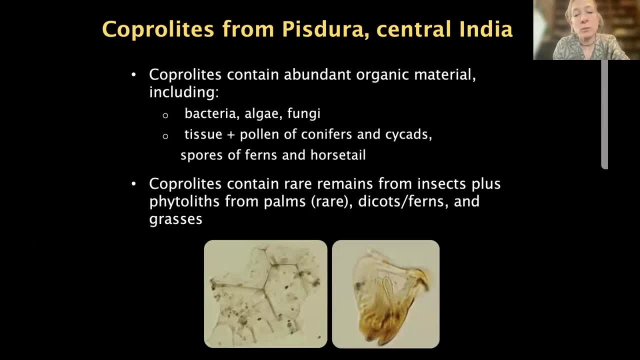 with chemicals and then we saw what we found, And what we found was rare remains from insects. So this is a jaw element here of an insect, plus some phytoliths both from ponds and also from the vegetation. So we got a lot of information. 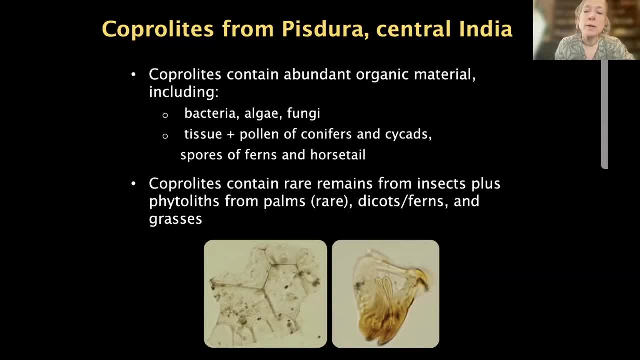 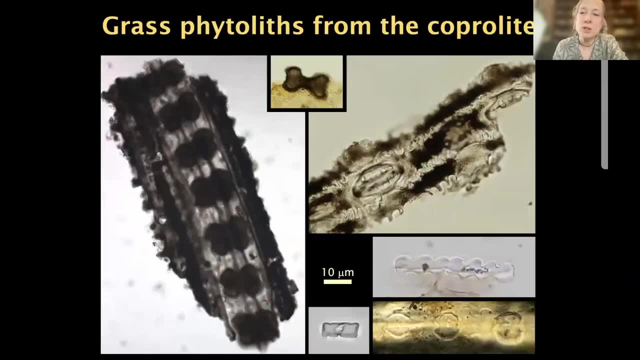 both from palms, dicots and ferns, but also from grasses. And this is the most important and exciting thing Here is showing some images of these lovely phytoliths. So, just to orient you here, here are some typical grass phytoliths. 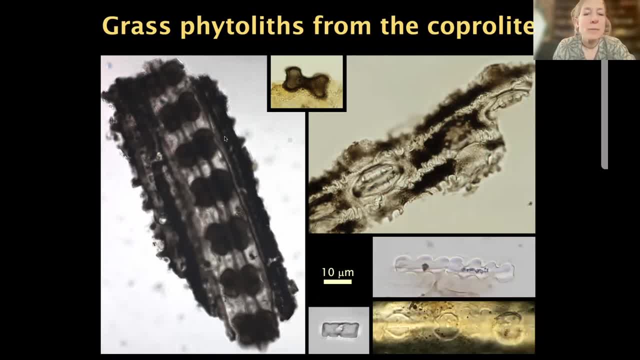 We call these short cell silica phytoliths. And then here are some silicified, basically epidermal cells around that And also in some cases, some cuticle, And cuticle is the waxy outer layer of a plant. 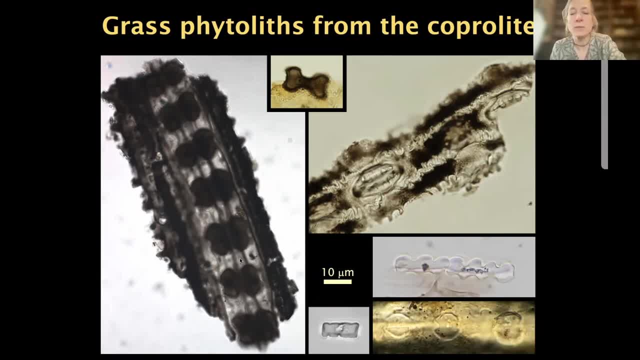 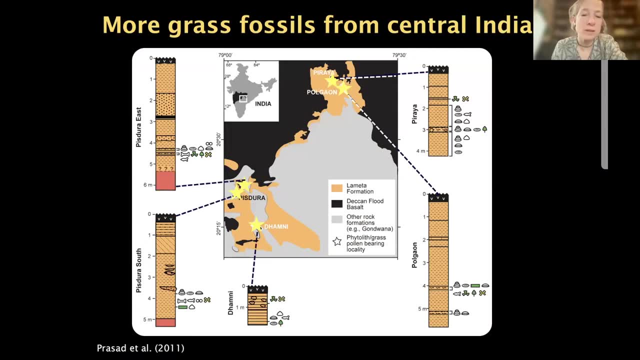 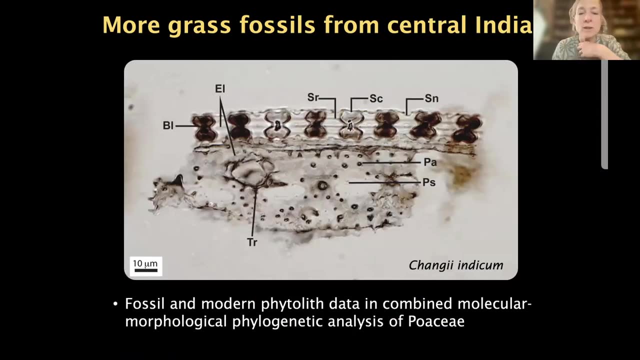 But we found a whole range of these different types of grass phytoliths. We've continued to work in India looking not just at coprolites but also at different sediments from the same time period in central India, And there we continue to find phytoliths and whole silicified pieces of epidermis. 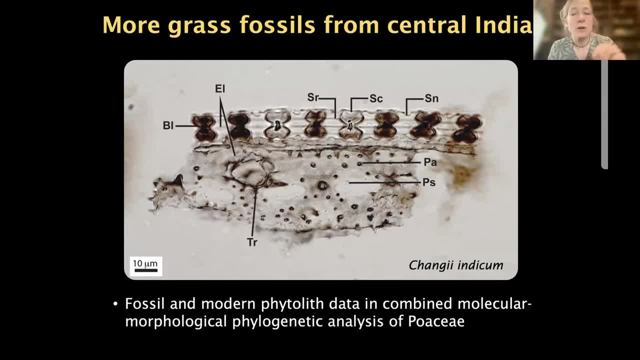 where we could get a lot of sort of you know characters, a lot of information from those. And so what we did was we looked at a whole bunch of modern grass, phytoliths and epidermal features And then we compare that to our fossil ones. 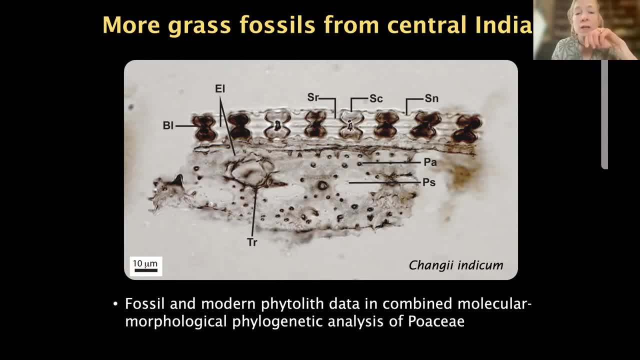 And then we use that in combination with DNA molecules to try to figure out where in the grass- phylogeny, so where in the family tree of grasses- these fossils fit. And so we did a phylogenetic, so-called phylogenetic analysis. 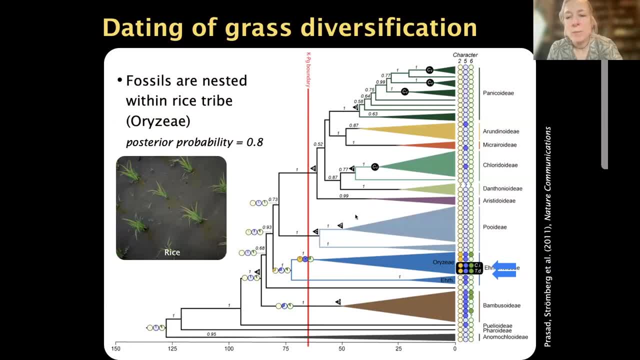 And we found, so this is the family tree that we came up with. We found that these fossils from India fit in the orise, which is the rice tribe within the grasses, And so that then allowed us to say that this tribe must have arisen by 66 million years ago. 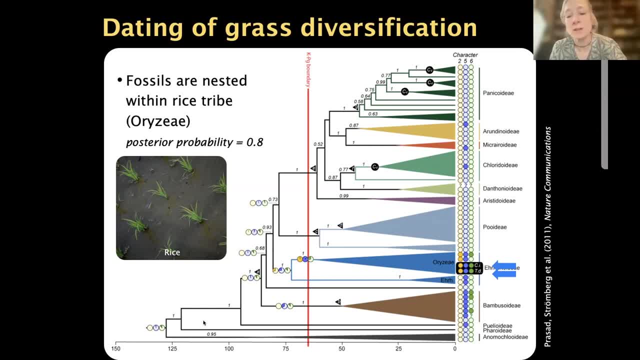 because that's the age of the fossil, And that then allowed us to date the entire tree, the entire family of grasses, And what we found was that grasses evolved much earlier than previously thought, in the early Cretaceous, maybe some 100, 125 million years ago. 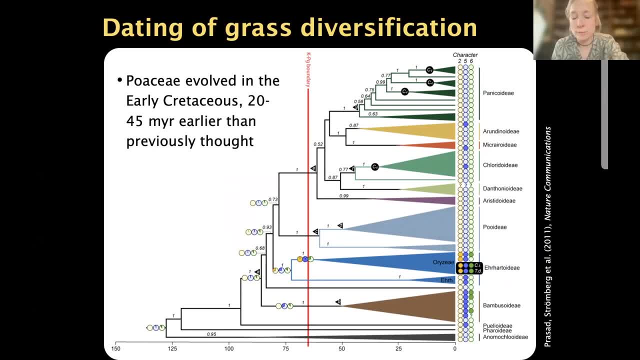 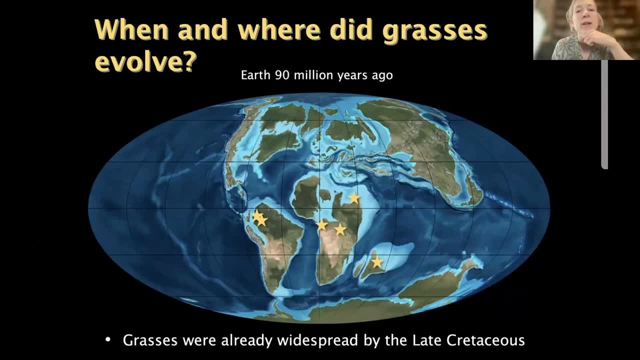 And that was up to 45 million years earlier than previously thought. So that was exciting And it also well so. it also has led us to think a little bit about where grasses evolved. So our fossils are from India, But there's also some pollen, grass pollen found in northern South America and in Africa. 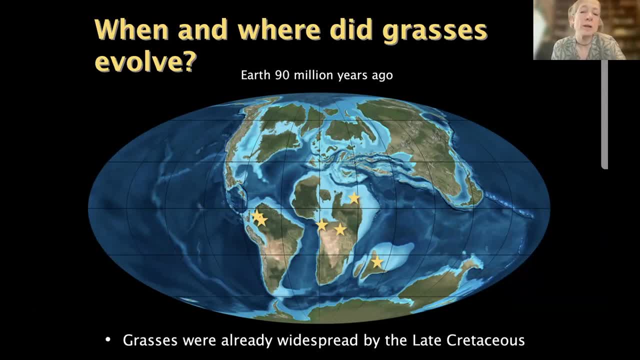 And so that led people for a long time to say that grasses probably evolved in the southern continent, so-called Gondwana land, and that they had done so before the late Cretaceous, because at that point they were already widespread across these continents. 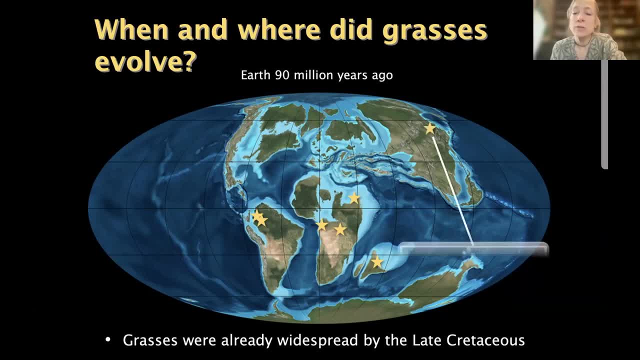 Now, just a few years ago. there's some fossil phytoliths described from China, And those fossil grass phytoliths were 100 million years old, so significantly older than the previously studied grass fossils, both the phytoliths and the pollen. 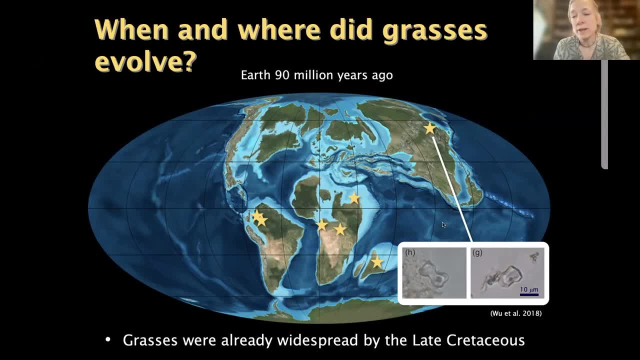 And they were actually found in the teeth of a hadrosaur, so definitely associated with dinosaurs. So this then calls into question whether grasses actually evolved on the southern continent. So now we really have to intensify the study and try to find fossil. 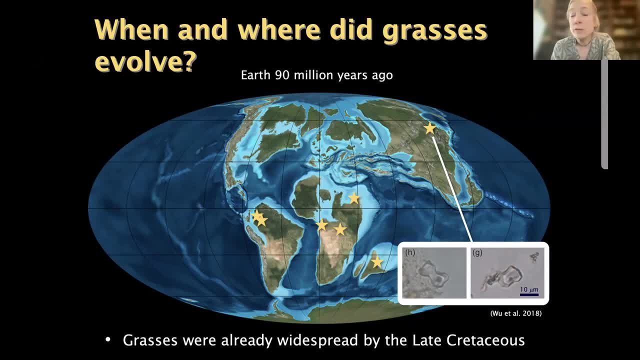 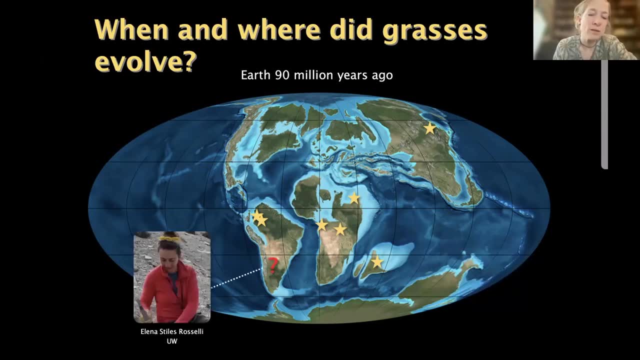 grass phytoliths and other grass fossils on different continents. to try to figure it out In the meantime, one of my grad students, Elena Stiles Rosselli, is looking at early grass phytoliths from southern South America, from Patagonia. 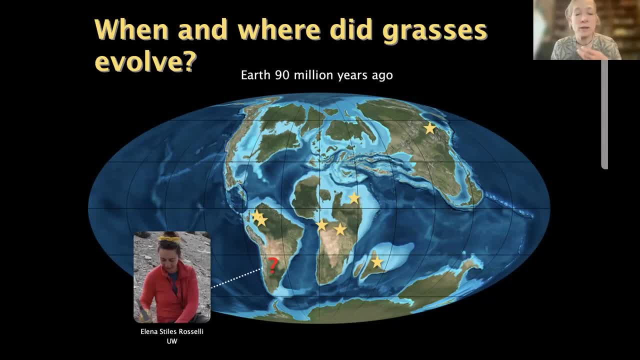 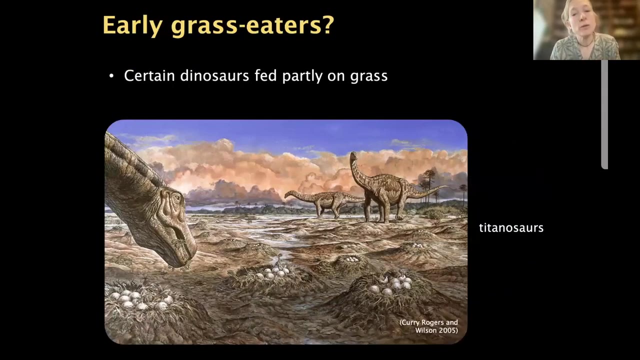 and tried to figure out what grasses were around there and in what habitats did they live, And, based on that, what can we say about how grasses diversified and spread across continents during the early days? The other thing that we could conclude based on our study is that certain dinosaurs fed partly on grass. 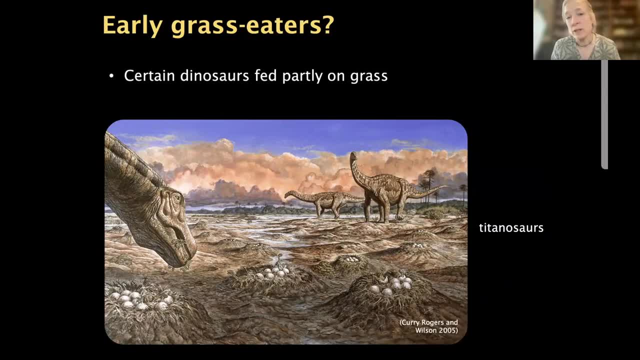 but that grasses were only a small component of a very varied diet And the herbivorous dinosaurs that were around at that time were titanosaurs, rather small sauropod dinosaurs, but potentially they were feeding on a very broad set of vegetation. 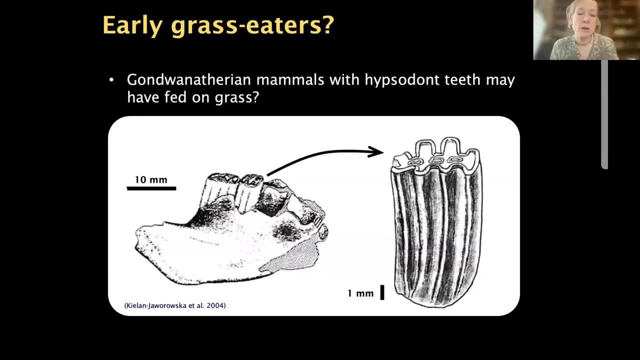 Another cool thing is that in India and other southern continents there's this marmot-sized mammal called Gundwan Aetherian mammal, and they have very hips, that on teeth, And previously the idea that they may have fed on grasses had been discounted. 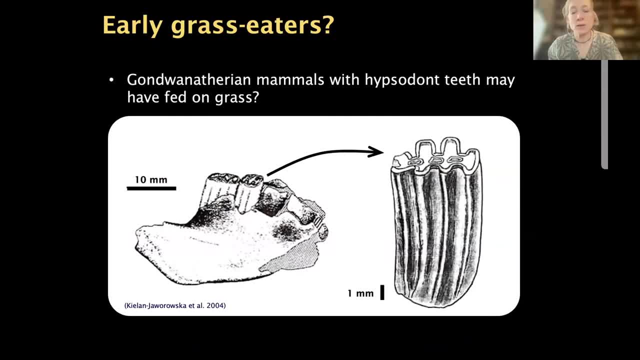 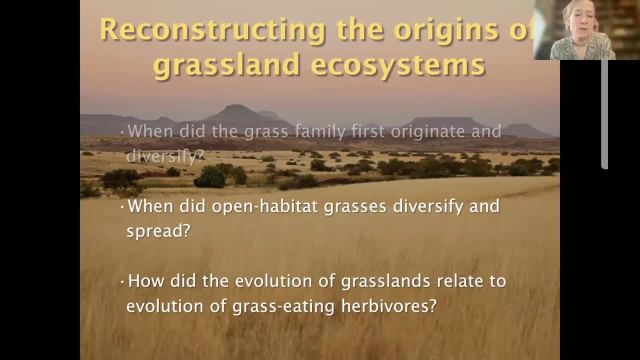 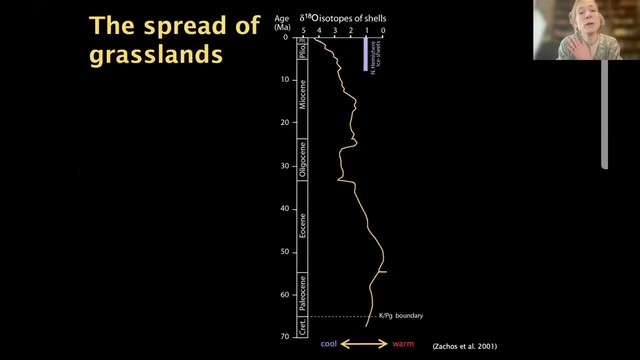 but now again, that is a hypothesis that we have to consider. Okay, so now let's switch gears to looking at when open habitat grass is diversified and spread, and how did that relate to the evolution of grass-eating herbivores? So the spread of grasslands has long been a challenge. 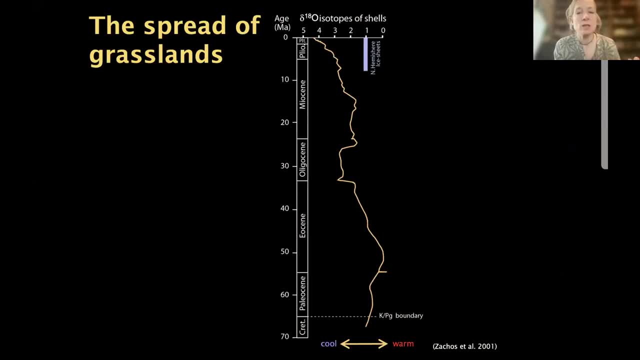 long been thought of as a response to changes in climate during the the last 66 million years. so to orient you here we have time moving forward on the y-axis as we go up, and then on the x-axis we have a global climate reconstructed using oxygen isotopes from shells of marine microorganisms. 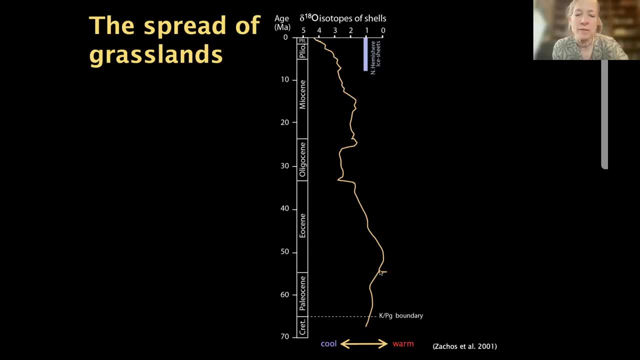 so-called foraminifera, and basically what we see here is that we have very high temperatures in the early eocene here around 50 million years ago, and then we see a decline and with some bumps in it, and so we have increasingly cool climates on earth, also on mid to high latitudes. we see 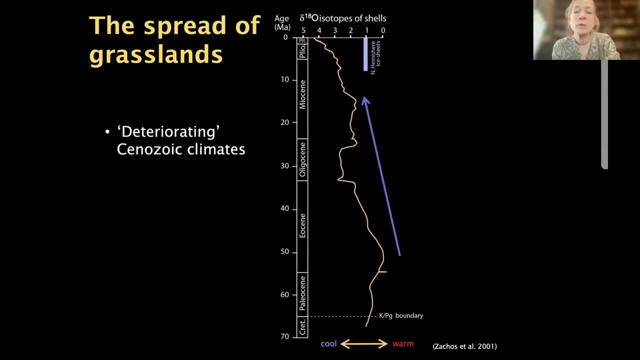 increasingly dry climates and for various reasons, and so the idea was always that grasses diversified and became abundant, as this was happening and that happened in co-evolution with herbivores that grew larger, grew hypsodont teeth and diversified and and became abundant. so there was this idea of 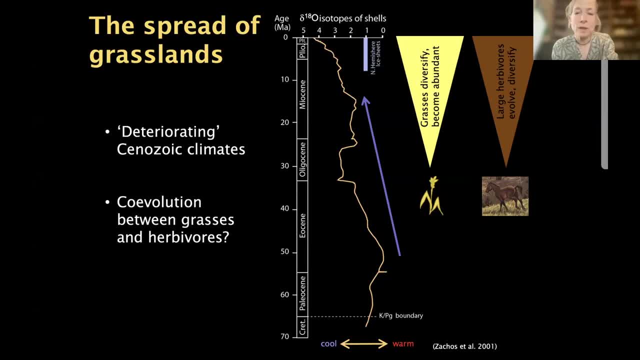 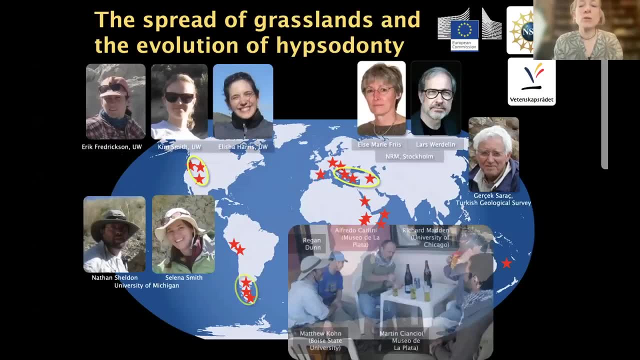 the co-evolution between grasses and herbivores during this time, and so this is something that we've wanted to work on and address, and this is just showing some of my many collaborators on these projects trying to reconstruct the spread of grasslands and the evolution of hypsodonti. 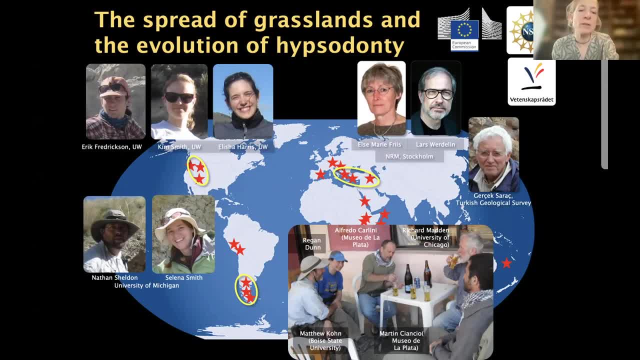 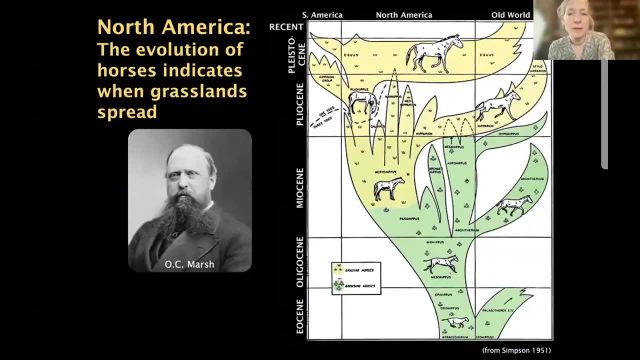 i'll be talking a little bit about these three areas in north america, eastern and eastern america, eastern mediterranean and patagonia as we go here. first, let's talk about north america. this is where, um classically, the evolution of horses happened after horses or the earliest. 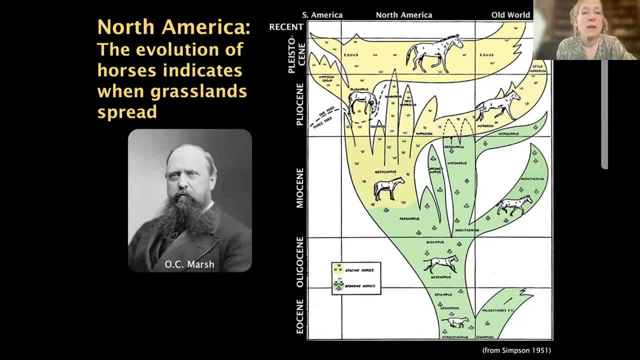 horses immigrated from from asia around 50, 50, 55 million years ago. north america has just a tremendous fossil record of this evolution of horses and in part because of the evolution of horses and the evolution of horses because of the many collecting uh trips that oc marsh and others. 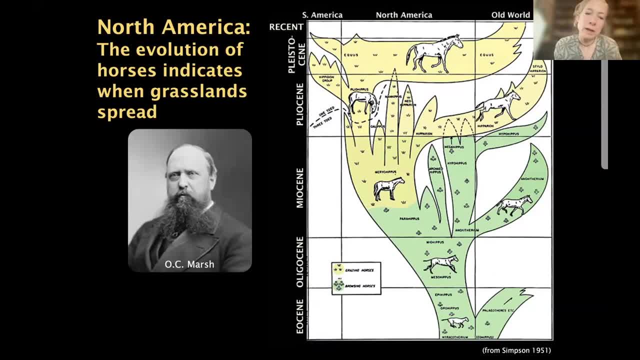 took and during that time, and i don't want to get into um the the horrible atrocities that happened against native americans as as a result of that- but one positive thing is that we we know a lot about horse evolution as a result and what we know here. 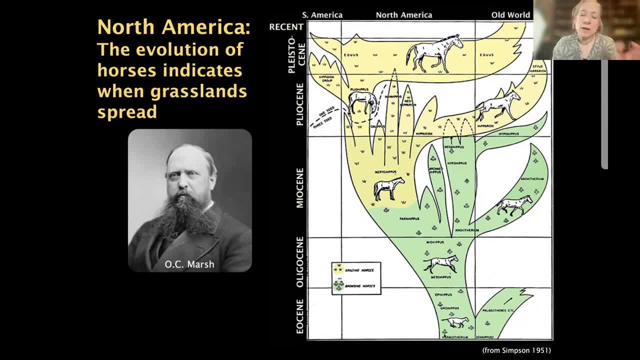 is that we see the evolution from these tiny early Eohippus that were capsized and have very low crown teeth, all the way to our large, long-legged and very hypsodont Equus, today the only living genus, and we see this diversification, And this was then thought. 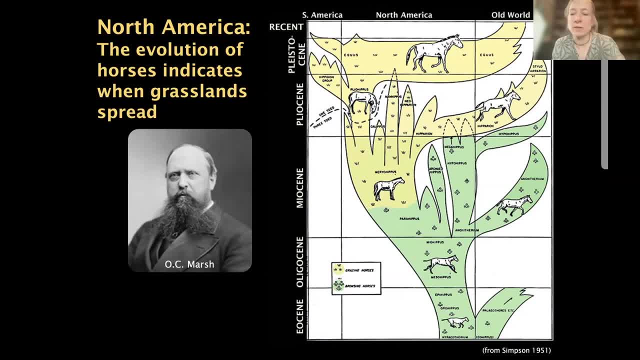 of as a response to the spread of grasslands, and this is shown here in this image from Simpson's book on horses And based on it, researchers pinpointed that sometime between 18 and 50 million years ago is likely when grassland spread, because that's when we start seeing the 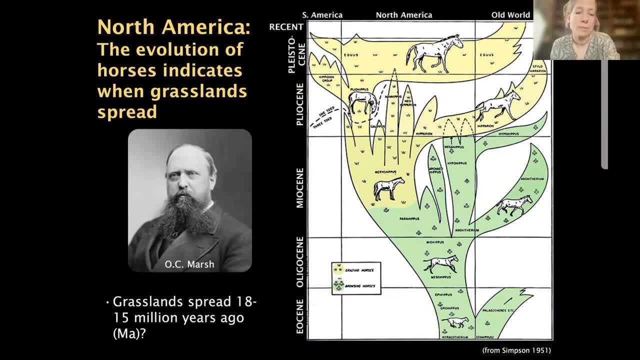 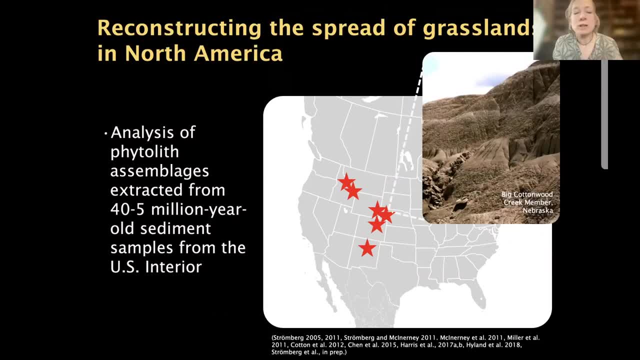 evolution of hypsodont really taking off within horses. This is something that we wanted to test, so I analyzed phytolith assemblages extracted from Eocene through Miocene into Pliocene sediments, so 40 to 5 million year old sediments from the US interior- and not just me, but me and my students and colleagues. 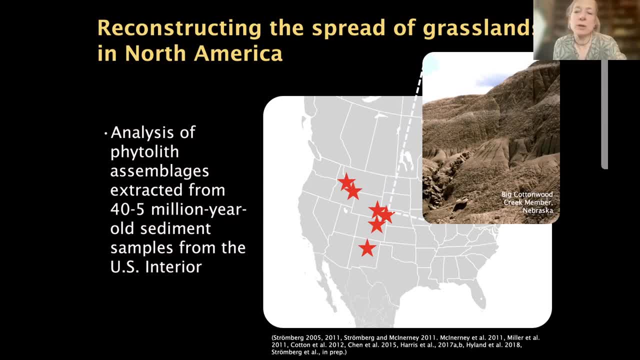 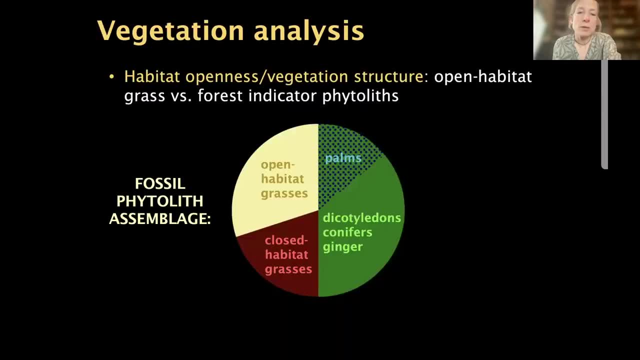 as well. This is showing one example of the kinds of areas, so we've tried to focus on areas where animal fossils have been found as well and that were well dated. So before we dive into the data, I just want to talk a little bit about how we analyze vegetation based on phytolith assemblages. 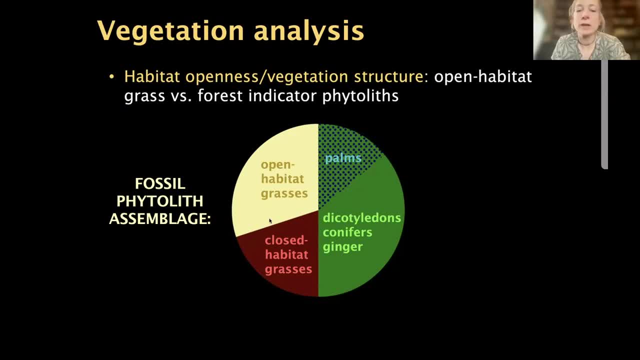 So this is showing this pie chart here is showing a fossil phytolith assemblage, and what we do is basically to reconstruct vegetation structure or habitat openness is that we compare the amount and types of open habitat grass phytoliths compared to phytoliths indicative of plants that tend to grow in. 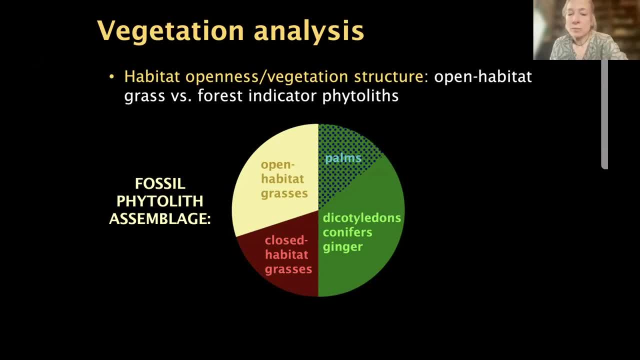 association with or in forests. Okay, so that's the simple way of saying it. and we also look inside the grass communities to look at closed habitat grasses and those also help us indicate that we're looking at a forest habitat. So the very coarse rule of thumb is that in grasslands we tend to see 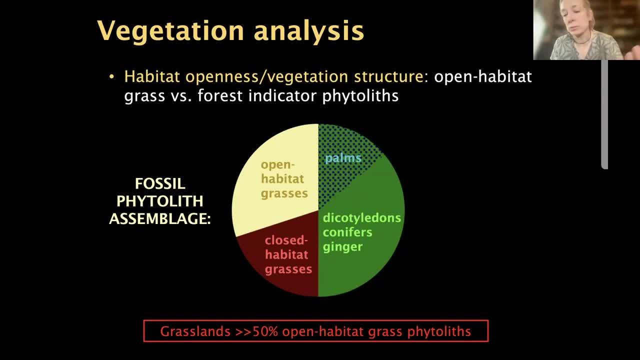 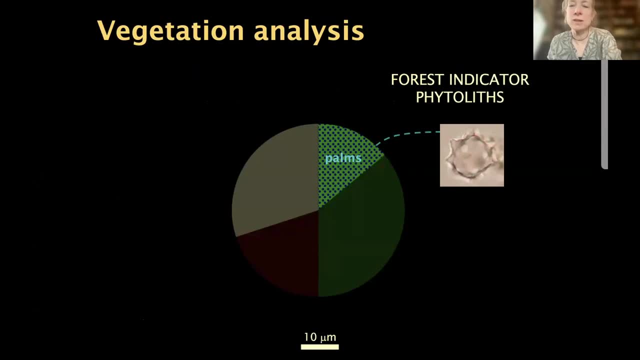 well over 50 percent open habitat grass phytoliths, and this will become important later on. This is just showing some of the pretty phytoliths that we have, so this is phytoliths indicative of palms- a range of phytoliths indicative. 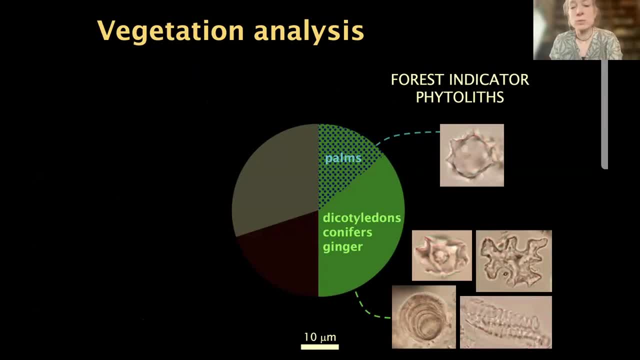 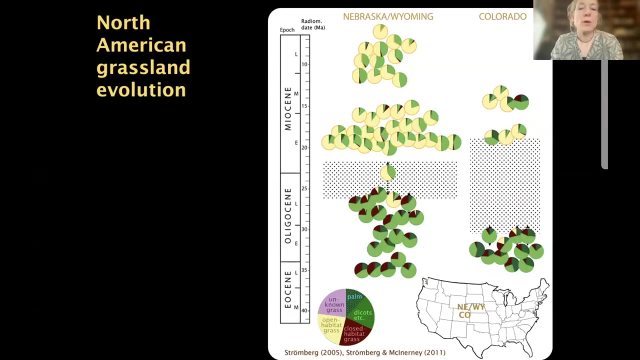 woody and herbaceous dicots, so angiosperms, conifers and gingers, And then we have our bamboos and other types of closed habitats, so forest grasses, and that's compared to, then the open habitat grass phytoliths. Okay, so let's dive straight into looking at North American. 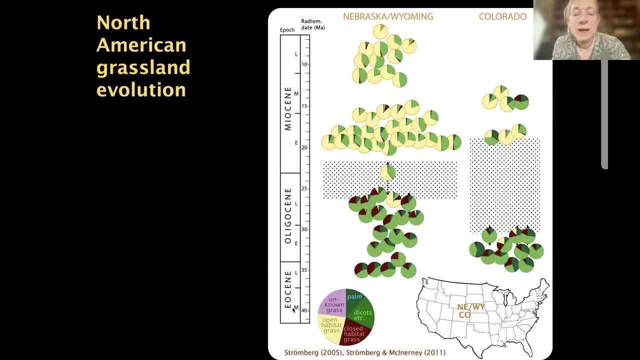 grassland evolution using phytoliths. Here we have again time on the y-axis moving forward as we go up, and then we have data from Nebraska-Wyoming and from Colorado, so the central Great Plains, if you will. What we see here is some clear patterns. First, I just want to point out that there's some 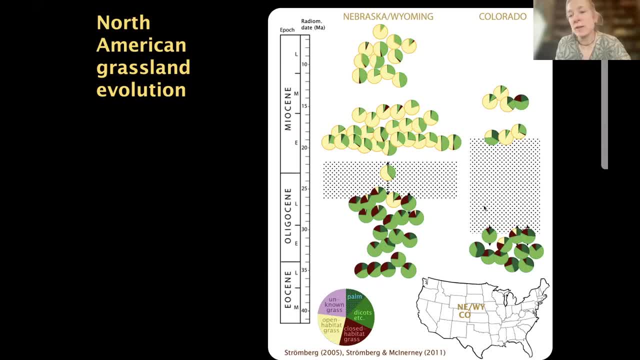 uncertainty in timing and some lack of data from some of these time periods and regions, but basically, what we think we're seeing is that the Eocene-Oligocene was dominated by forests. so these pie charts, or these assemblages, are dominated by forest indicators. Grass communities are, by and large, dominated by 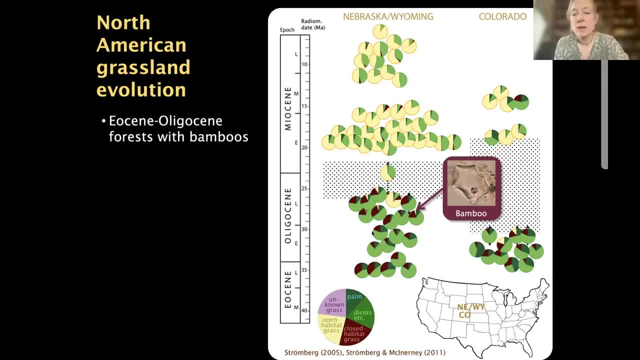 bamboo phytoliths, or what we interpreted as bamboo phytoliths. And then we still, during this time, we still see minor abundancies and in some cases, more higher abundancies of typical looking open habitat grass phytoliths- This is a Poide phytolith, for example- and this is happening in the late. 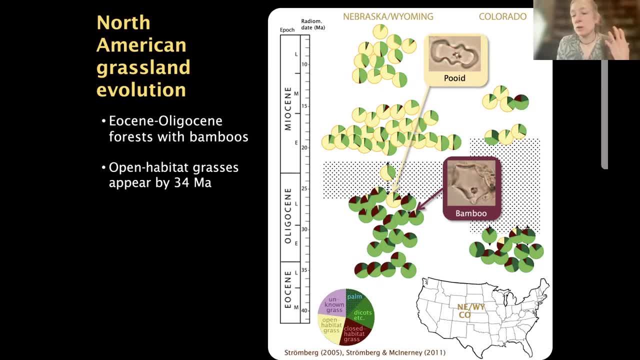 Eocene. So this indicates to us that, even though these are primarily forest habitats, we have open habitat grasses present either in the understory or in gaps or at the margins of forests. And then we see sometime during the late Oligocene or early Miocene, depending on the 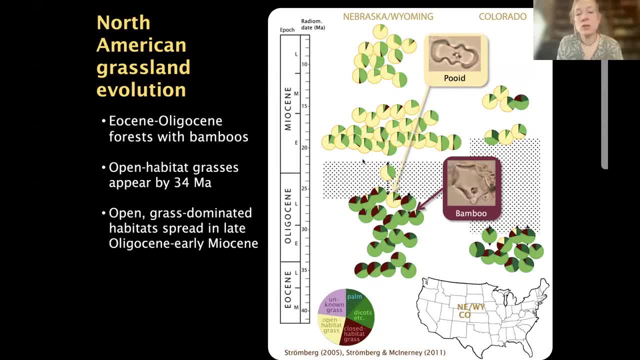 dating of some of these assemblages, we see an expansion of these open habitat grasses into open grass-dominated habitats, maybe woodlands, maybe savannas, most likely some kind of mosaic of these, Of more forested patches and more open patches. And this is happening, like I said, in the late. 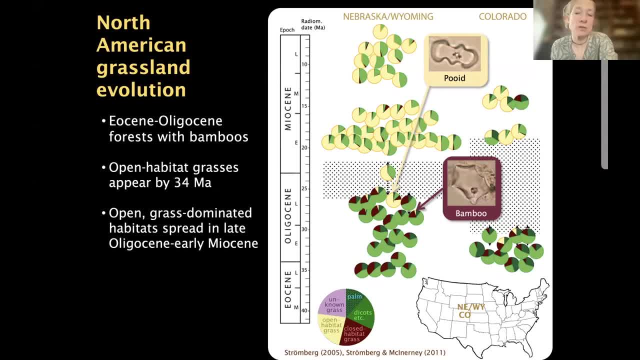 Oligocene or early Miocene, maybe 25 to 22 million years ago. And, importantly, these earliest grasslands were dominated by cool, temperate Poide grasses. These are grasses with the ancestral photosynthetic pathway C3, but we're not going to talk very much. 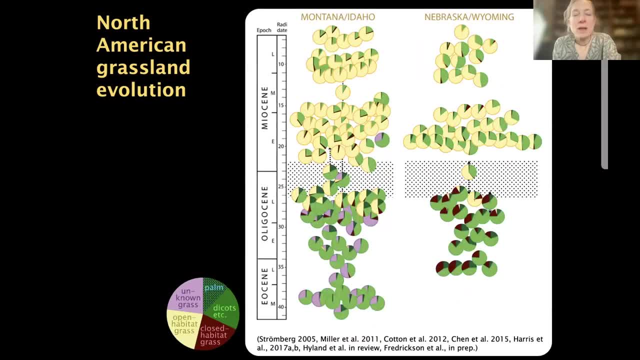 about that, so you can ignore that. We also have looked. So now we have some poppy, we also have some magma, we also have communean tree, we have some bumblebees, we have some dendritic tree, we also have some bonyerer, We also have some. 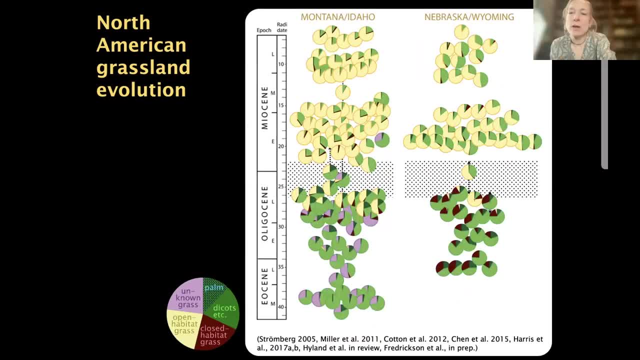 small trees and we are also talking about the more open patch of woodland. This is happening from the. We also have looked, so now I removed Colorado. we've also looked at Montana, Idaho, so this is a little bit further north, and we see there a similar pattern actually, where we 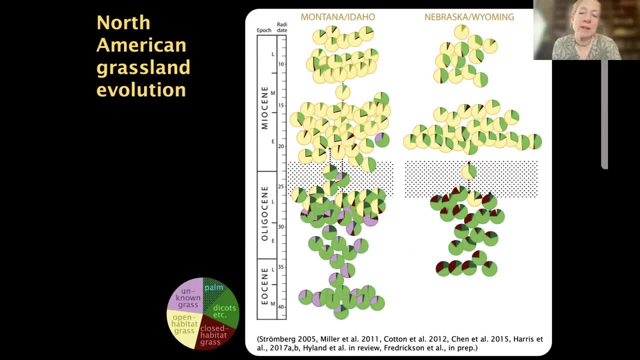 see forests, more closed habitats in the Eocene and Ligocene. The difference here is that we have a different set of grasses. We're not entirely sure if they are closed habitat or open habitat, but primarily we see closed habitats here, maybe with some more local, more grassy habitats and then 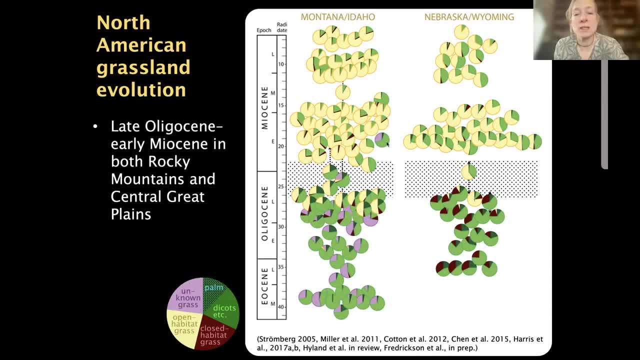 sometime in the late Ligocene or early Miocene, we see the expansion of typical open habitat grasses, forming some kind of open grass-dominated habitats, also in the northern Rockies, so the Montana and Idaho, And so this indicates to us that this shift it's actually 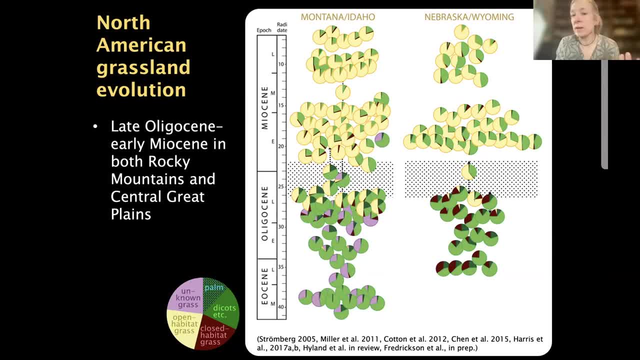 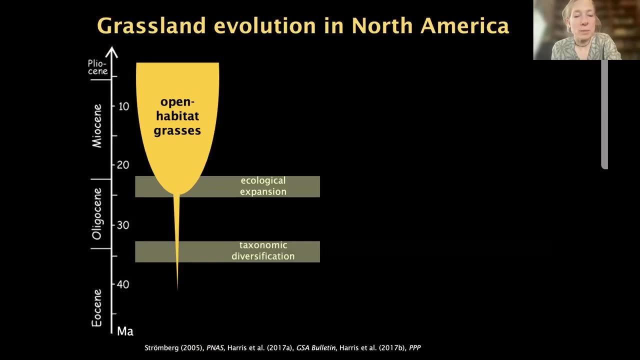 seems to be fairly synchronous between these regions, indicating that some large-scale change must have happened to allow these open habitat grasses to expand, and we'll get back to that. So what are these data showing? They're showing that the taxonomic diversification of grasses, of these open habitat grasses, 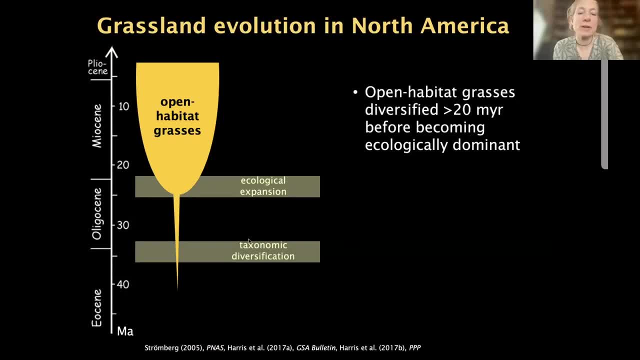 is happening down here when we see our earliest open habitat grasses, but it's not until some 20 million years later- Actually, here In North America it's more like 11 million years later, at least- that we see the expansion. 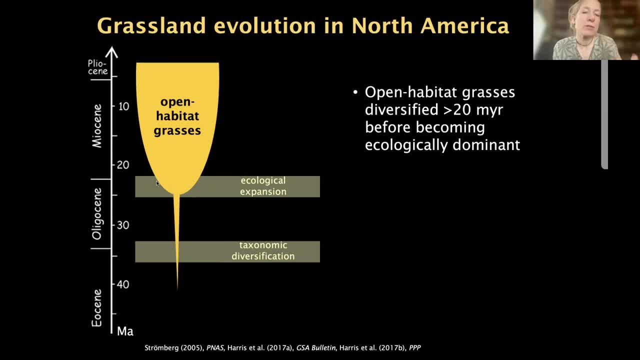 the ecological expansion of open habitat grasses, So when they become ecologically dominant. and this indicates then that there were different drivers between the taxonomic diversification and the ecological expansion, And what were some of these drivers then? We have collaborated with some geochemists. 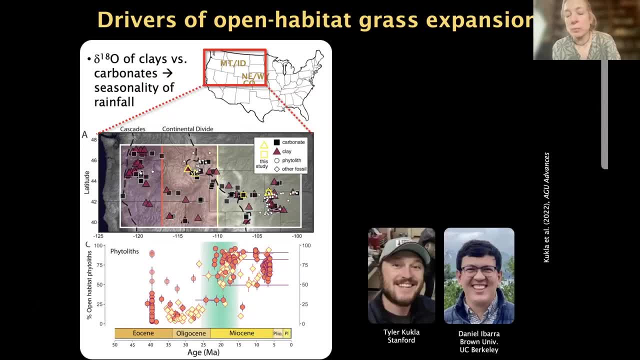 Tyler Kukla, who used to be at Stanford but is now actually doing a postdoc at University of Washington, and some other folks. And what they did was they looked at the isotopes, the oxygen isotopes of clays and carbonates. 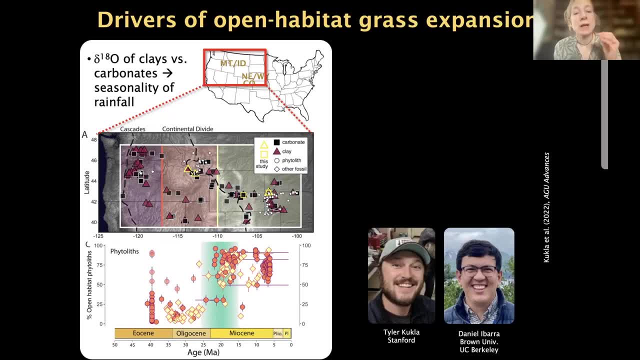 So these are different minerals in the sediment or the soil And this allows us to say something about rainfall, of seasonality. So they looked across this western US, here including the regions that I talked about, and they took samples across those regions. 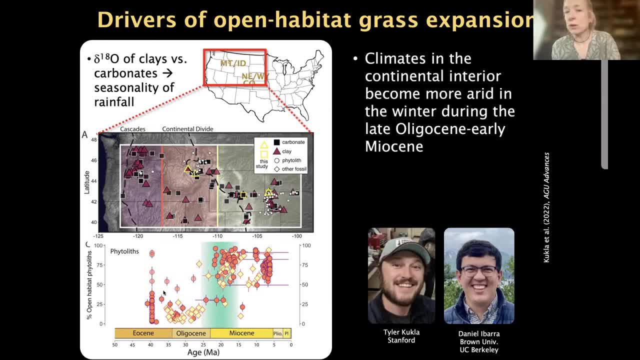 And compared it to the phytolith data down here. And, to make a long story short, they found that climates in the continental interior became more arid in the winter during the late Oligocene to early Miocene, So we see an increase in winter aridity during that time. 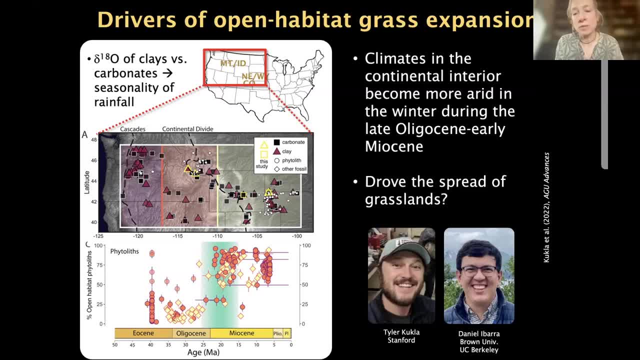 So this seems to coincide with this opening up of landscape and the spread of open grass-dominated habitats. So we are hypothesizing that that change is what drove that And we are further hypothesizing. We are hypothesizing that it may have been the rise of the cascades in the west here. 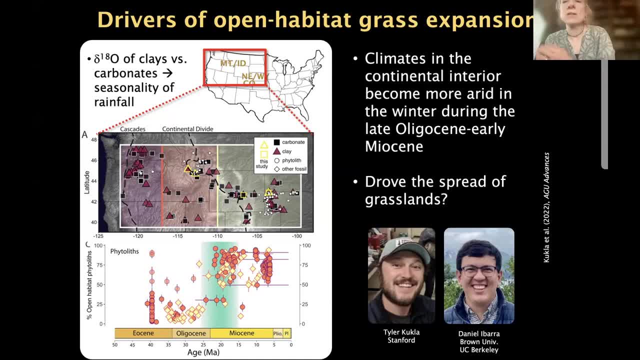 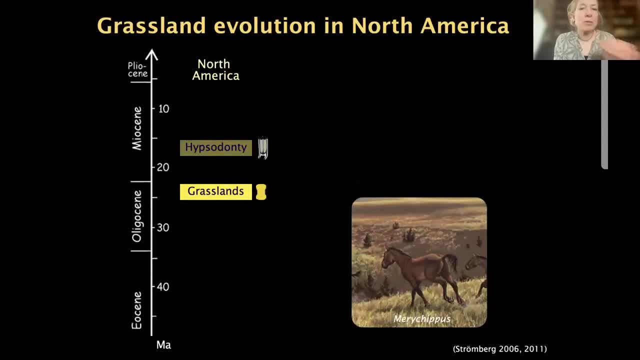 that helped create this gradient of aridity across the western US. Okay, What about the evolution of grasslands in relation to the evolution of hypsodontae in North America? What we see is that hypsodontae evolved at least four million years after the spread. 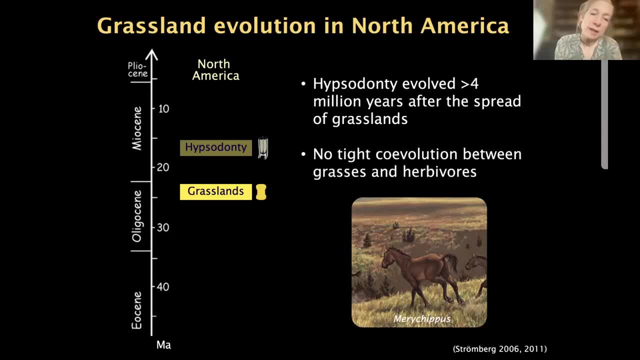 of grasslands, And so, even though We think that hypsodontae could still be an adaptation to these new open habitats, there doesn't seem to be a tight co-evolution between grasses and herbivores. The take-home message, though, is that these herbivores evolved in the context of open 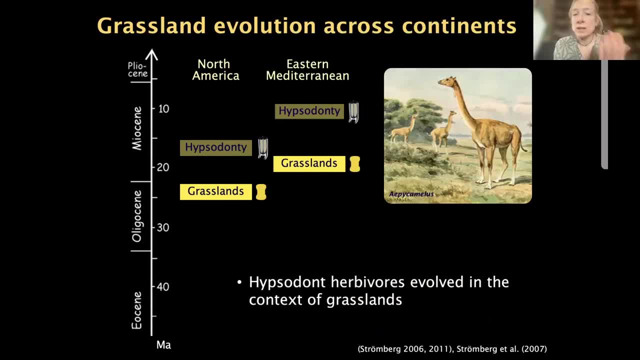 grass-dominated habitats. If we look at the Eastern Mediterranean, we see a similar pattern of a long delay- several million years- between the spread of grasslands and the evolution of hypsodontae. But again, the idea here is that hypsodont herbivores evolved within grasslands. 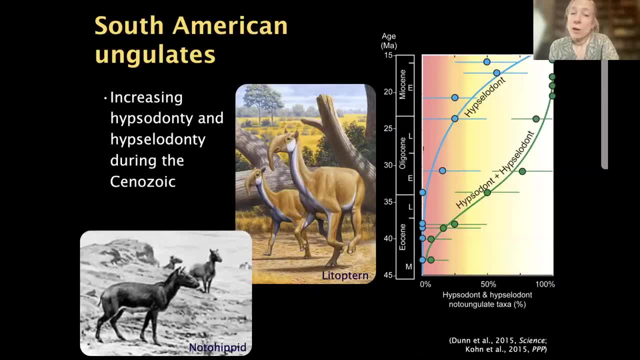 grasslands or grassy habitats. now we were interested in looking at south america as well, because in south america we have an endemic group of hoofed mammals that are now entirely extinct, so-called southern ungulates or meridi ungulates, and they evolved, increasing hypsodonti and 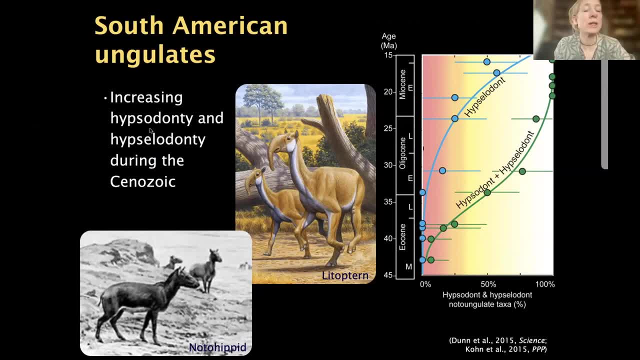 something called hypsilodonti, which is basically ever-growing teeth, so an extreme version of hypsodonti during the xenozoic. so if we look here through time, we see that hypsodont and hypsilodont cheek teeth increase through time and this is looking within the node ungulate. 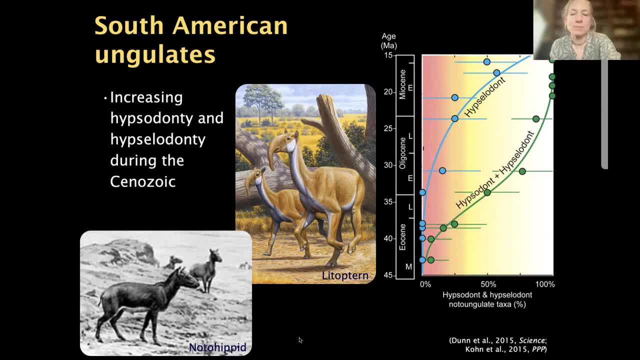 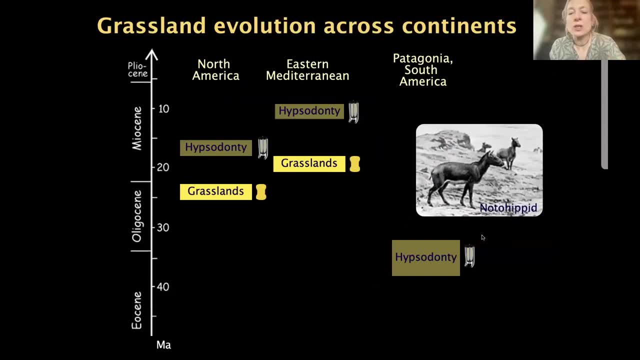 group, which is a subgroup of these southern ungulates. so we were interested in in looking at that and and just to say that we see this change happening very early on the evolution of hypsodonti, so 20 million years earlier than on other climates. so we see this change happening very early on the evolution of hypsodonti, so 20 million years earlier than on other climates. 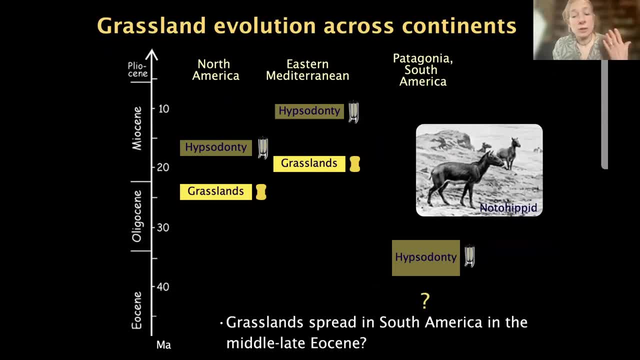 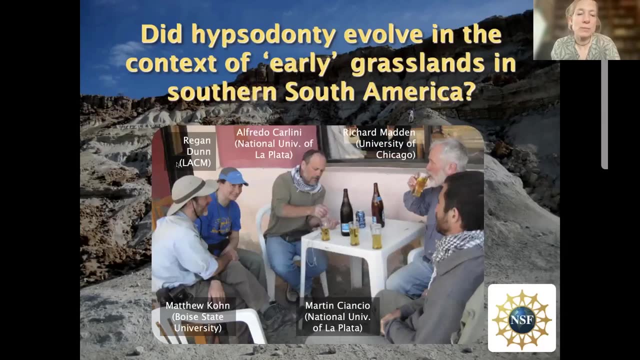 and so the idea had been that the earliest grasslands on earth actually spread in south america in the middle to late eocene, around 40 million years ago. so this is something that we wanted to test, and this is the team that set out to test that, and the most important person here is 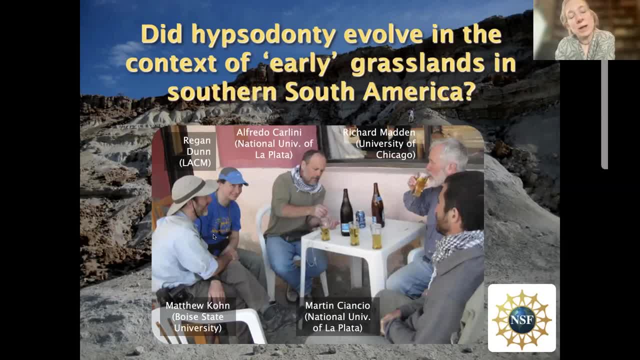 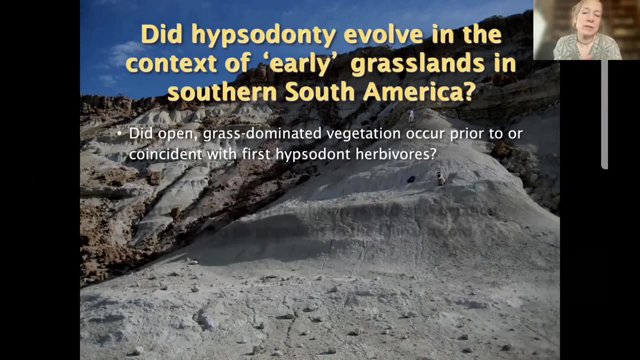 my now former grad student, reagan dunn, who is now at la brea tar pits as a curator of paleobotany there, but also a whole group of vertebrate paleontologists and geochemists here, and so we were interested in looking at whether open grass dominated vegetation occurred prior to. 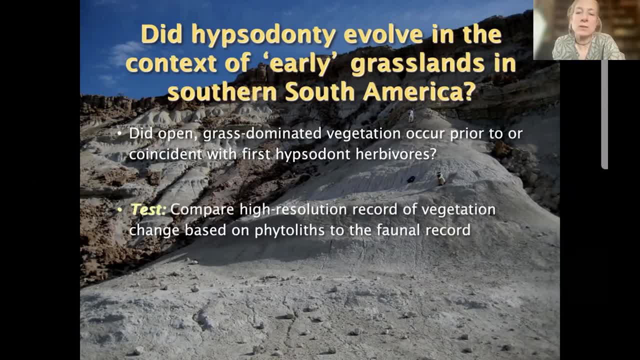 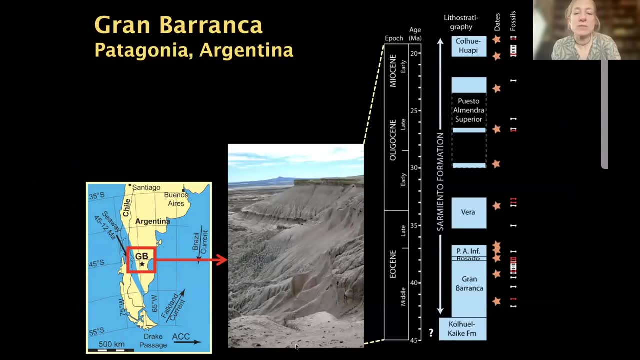 or coincident, with the first hypsodont herbivores in southern south america. and the test then, of course, is to reconstruct vegetation based on phytoliths and compare it to the faunal record. so to do that, we went to a place called gran barranca, in paragonia argentina, which is this: 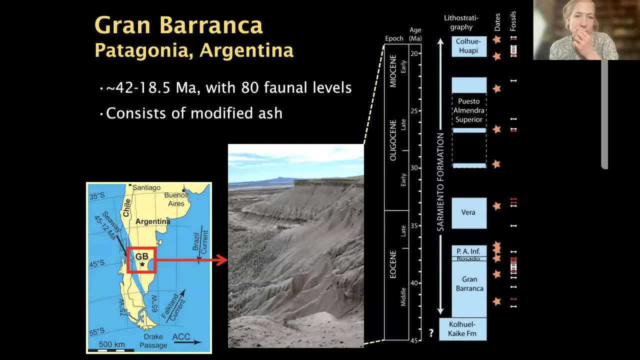 very long section of rocks that spans 42 to 18 and a half million years, so um middle eocene, through um, through the early miocene, and it has 80 faunal levels. so a lot of faunal evolution is recorded in this section and the the sediments here. 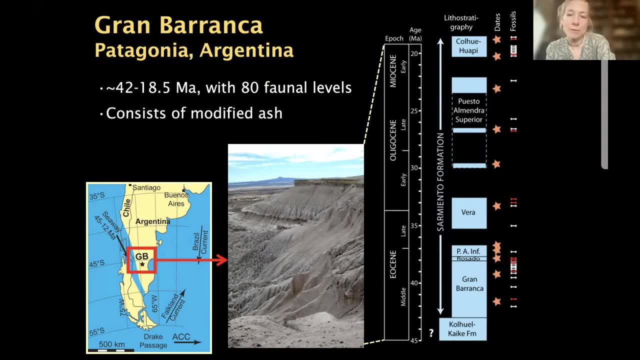 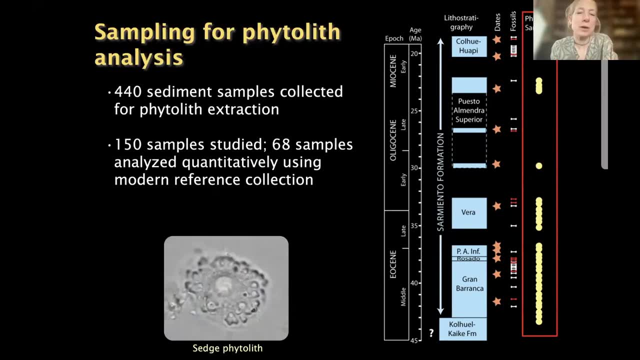 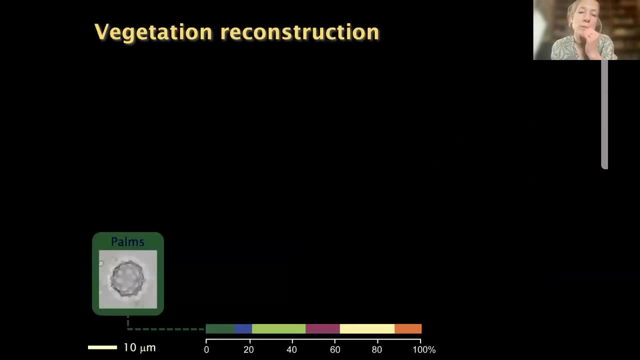 are modified volcanic ash- and this will become important later on- and so we sampled extensively for phytoliths and analyzed a whole bunch of samples from there, and the preservation is primarily quite good. so that's cool, and we used our modern reference collection to classify them, of course, as we do, and just to 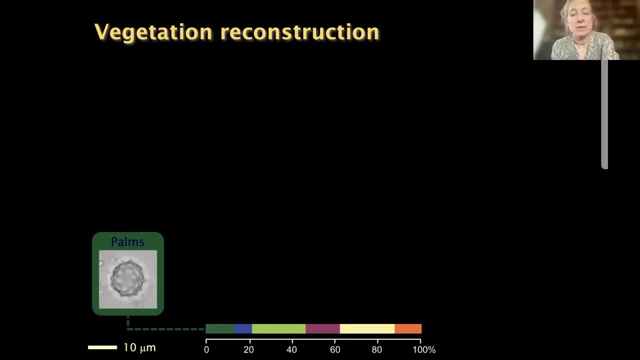 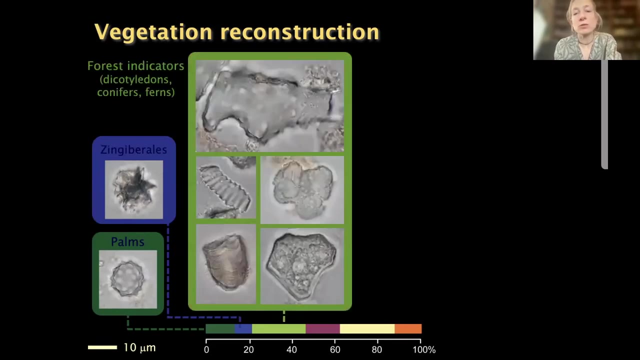 remind you of of these different things, because now we're going to look at a phytolith assemblage as a bar graph graph. we have palms, we have um, ginger spiral, genders and relatives. these are tropical herbs that tend to be associated with forests, and then we have other forest indicators. 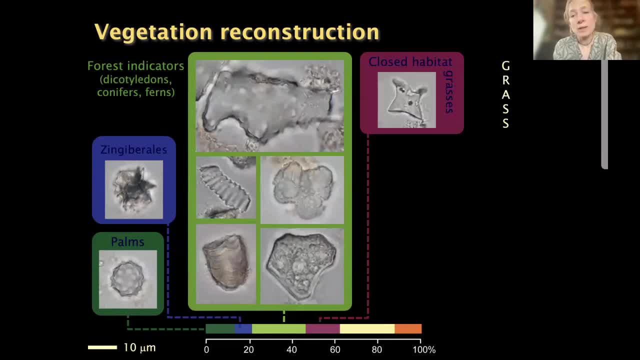 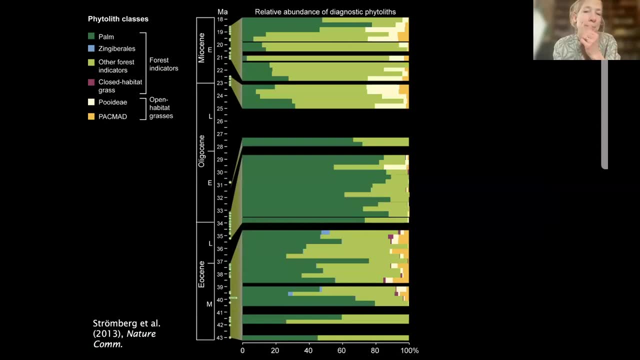 woody and herbaceous dicots and so on, and we have closed habitat grasses and we have our open habitat grass grasses and the poets and pack mats. okay, so, um then, uh, let's look at the data. so here we have time moving forward on the y-axis as we go up and we have our phytolith assemblages as bar charts. 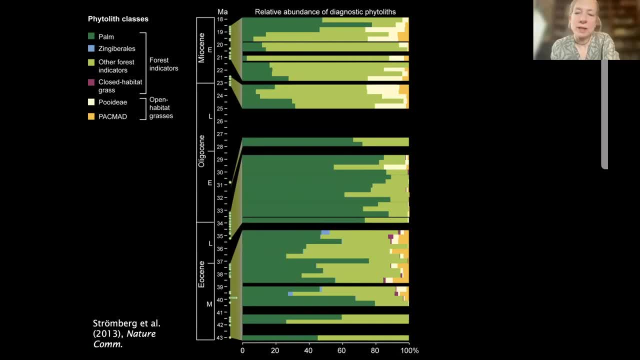 here, and and what we see- a striking pattern here- is that grass phytoliths are less than 25 percent of any given assemblage, even though we see grasses present from about 43 million years ago and by 40 million years we have representatives of modern clades such as bamboos and also open. 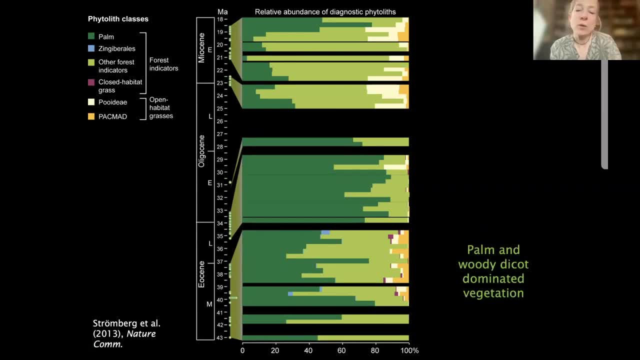 habitat grasses, poets and pack mats and so- but these grasses are are quite, uh, rare, relatively speaking, and we have primarily a lot of palms and a lot of woody and herbaceous dicots, so we interpreted this initially as some kind of forest, and this vegetation type seems to persist through. 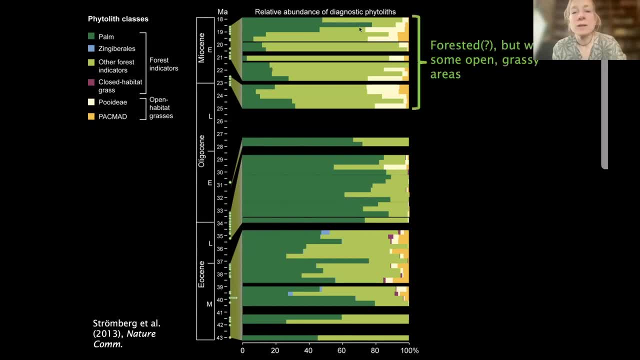 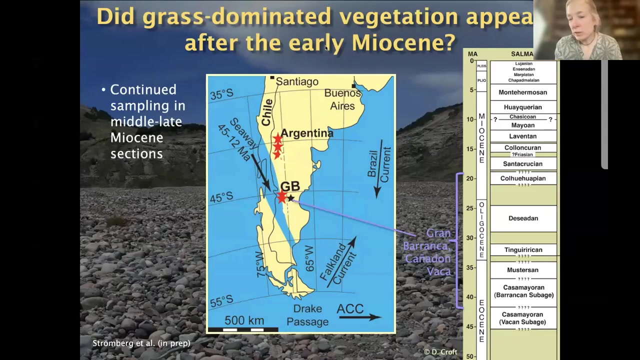 up here through the, the legocene and then in the miocene, we start seeing, uh, more abundant open habitat grasses- up to 25 percent- but uh, still primarily dominated by other plants. so we still interpreted this as forested, but with maybe some open grassy areas. um, yeah, and we looked at at gran barranca. we've also. 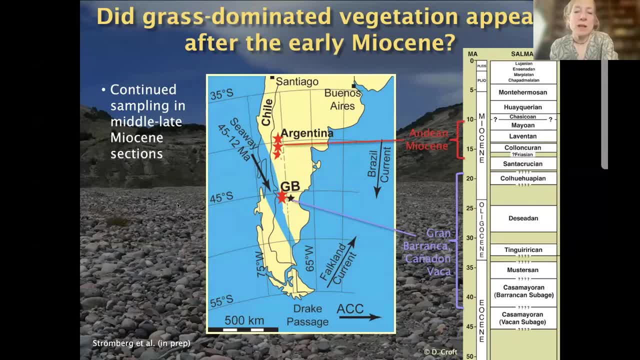 looked a little bit higher up in the section, so at younger sediments and, and we've also looked at a little bit higher up in the section, so at younger sediments and, and we've also looked at a little bit higher up in the section, so at younger sediments. 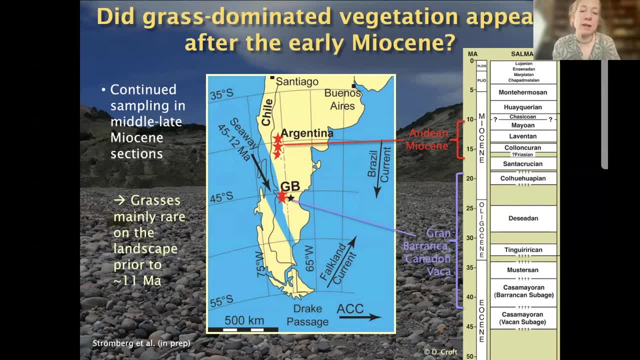 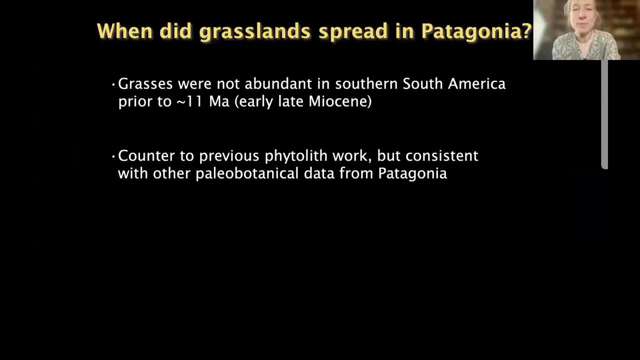 we found a similar thing here, that grasses are mainly rare on the landscape prior to about 11 million years. we haven't we, we haven't- analyzed anything younger than that. so that's what we know, and so we concluded then that grasses were not abundant in southern south america prior to. 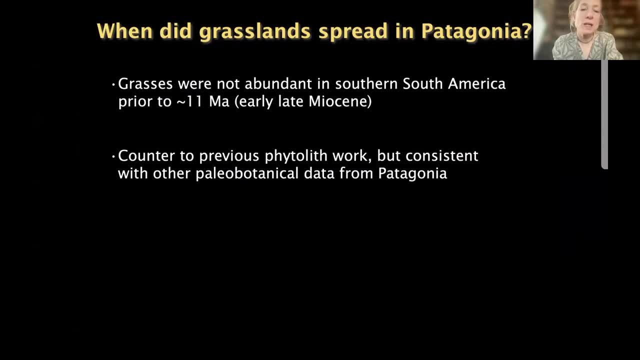 about 11 million years ago, so the early, late miocene, and this is counter to previous phytolith work that had been done in that region, but it is consistent with other paleobotanical data from the same region, uh, in particular the phytolith work that had been done in that region, but it is. 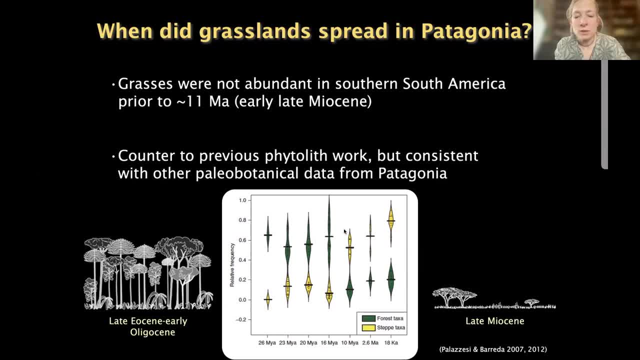 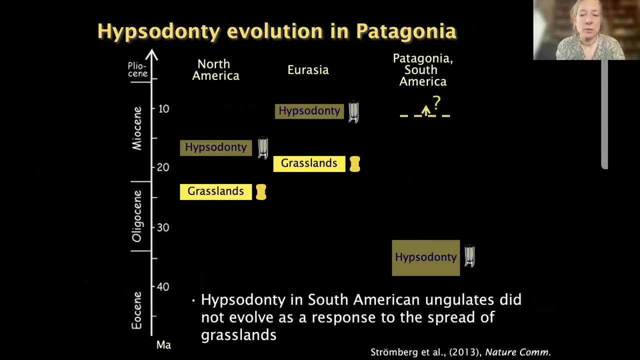 consistent with other paleobotanical data from the same region, but it is consistent with other fossil pollen which indicate that it's not until after about 10 million years that we see step taxa. so grasses and other types of pollen dominate over the forest taxa. okay, so what about hypsodont evolution in patagonia? so we can conclude that 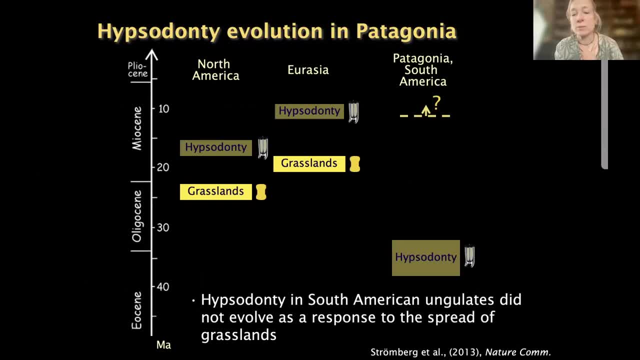 hypsodonti and south american ungulates did not evolve as a response to the spread of grasslands, because there were no grasslands when hypsodonti came around. but what do we know about open grasslands? but what do we know about open grasslands? 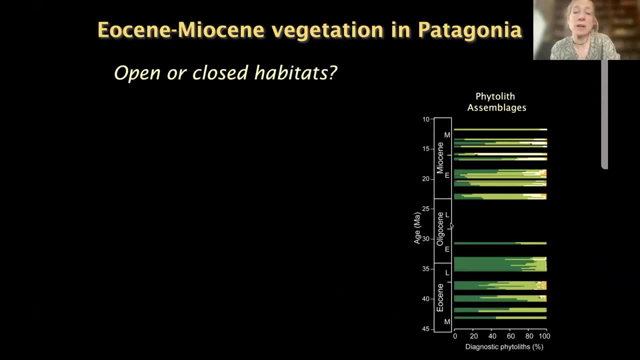 so i told you that we interpreted this primarily as forests and and this is because in traditional and this is because in traditional phytolith analysis, we use the presence and and abundance of open habitat grasses as an indicator for the, the openness, basically. and but what about if you're? 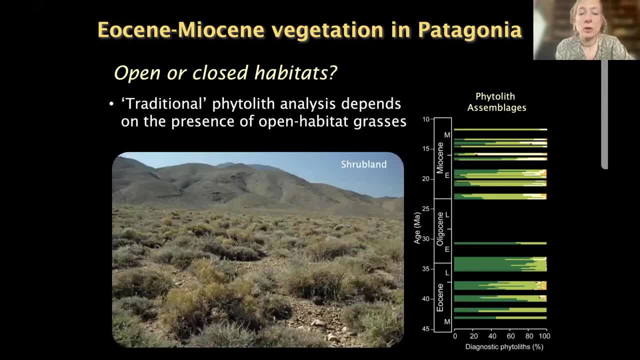 looking at a habitat that is very open but where grasses are not dominant, such as this shrubland. なた는аютiskaighli так etapahgenia ablega harirbað sa Vie consensus. castocku här an tadi bares tak viessel줘. 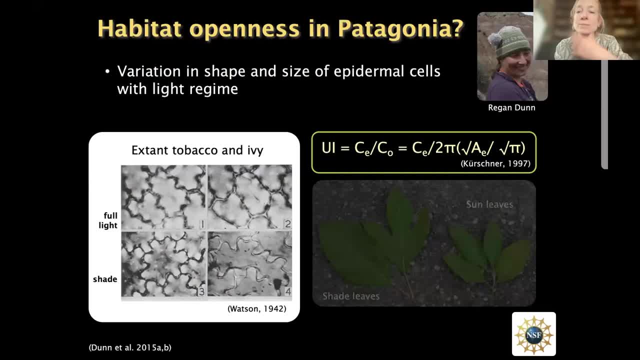 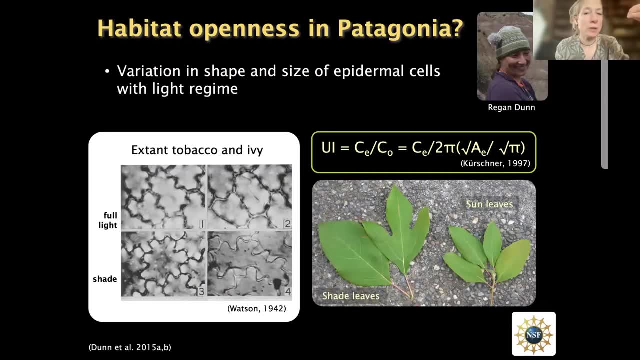 detect that in the fossil record. so reagan, and with reagan we set out to come up with an alternative way of of inferring openness in the fossil record using phytoliths and reagan, came up with this idea that we could use: uh, that there's variation in plant traits with light. so, for example, if you 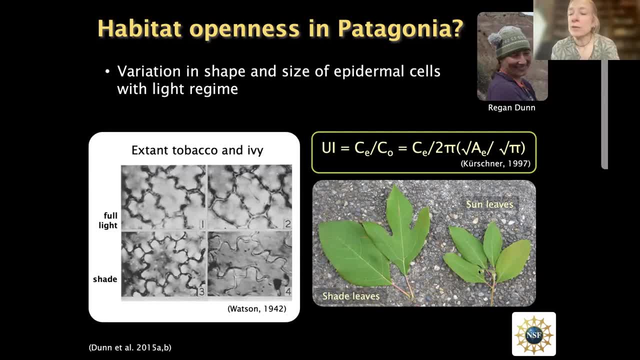 look at at leaves, leaves growing in the sun have a different uh size, they're smaller and they are less lobed than leaves growing in the shade, because that is how they optimize uh, their, their surface area and so on: uh for, for the light, um, and similarly when we look at the, the epidermal. 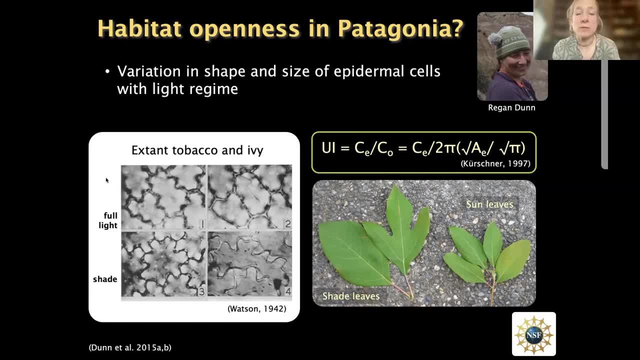 the epidermis of plants growing in full light versus shade, we see differences in the the shape and size of cells. so the cells that grow in full light tend to be smaller and less undulated than cells grown in the shade, and in fact there's even 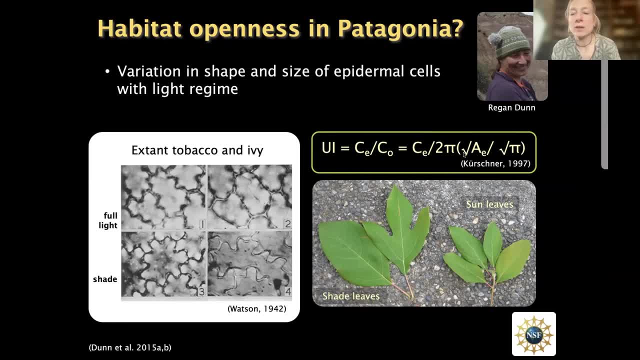 an equation for this, the so-called undulation index, uh, set up by this pelibotanist, wolfram kirschner, to measure the, the degree of undulation, and correlate that with the, the uh, whether it was a sun leaf or a shade leaf. but what we wanted to do was to actually use phytoliths to reconstruct. 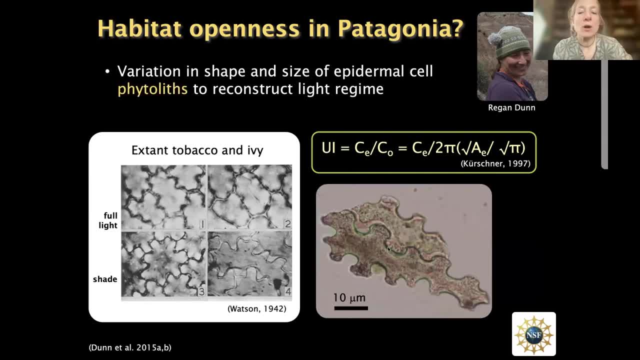 light regime. and we can do that because epidermal phytoliths are often a direct cast, it's just a copy, it's an infilling of an epidermal cell. so the shape of that epidermal cell will be reflected in the phytolith and the size, and we 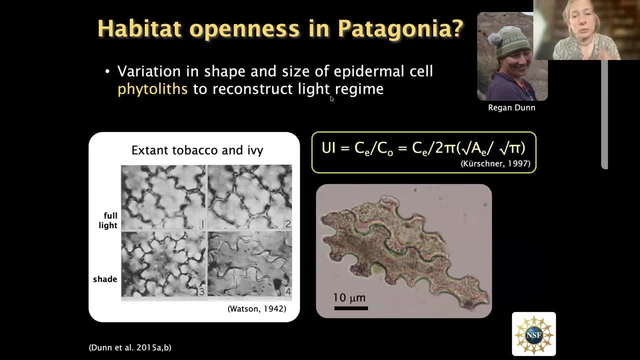 wanted to look at phytoliths that we extracted from a soil sample or a sediment sample and look at the, the distribution of those shapes and sizes, and use the average to say what kind of light regime was present at this site. so, and and i should say that the, the, the, the, the, the, the. 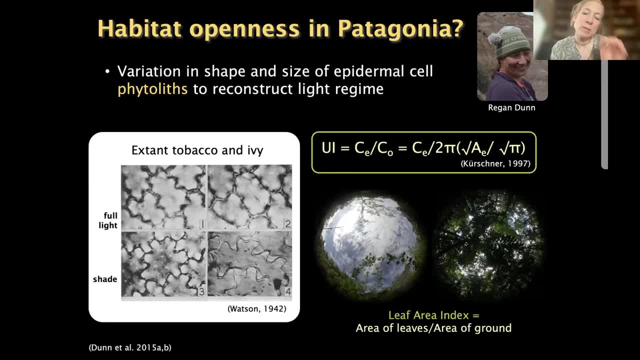 what we wanted to reconstruct is a is a measurement called the leaf area index, which is basically a measurement of openness. it looks at the area of leaves relative to the area of the ground. this is a hemispherical photograph, taking straight up, and you can see here in this habitat, we have very 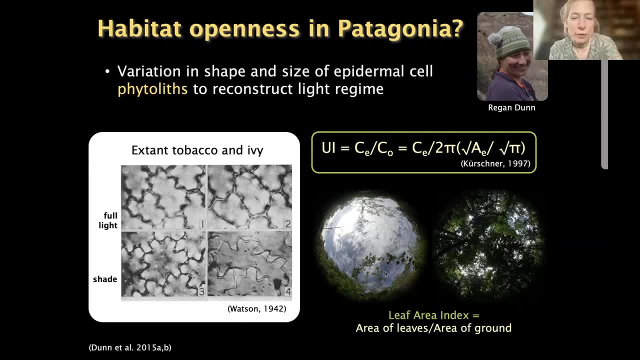 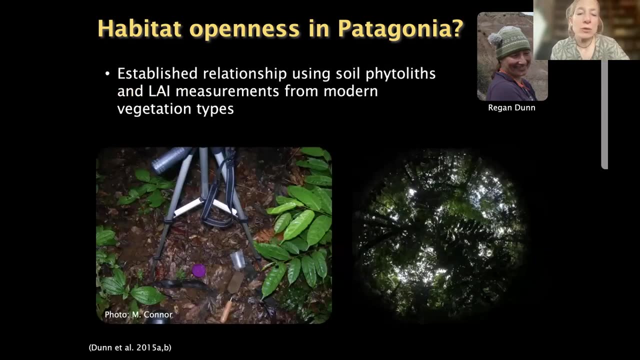 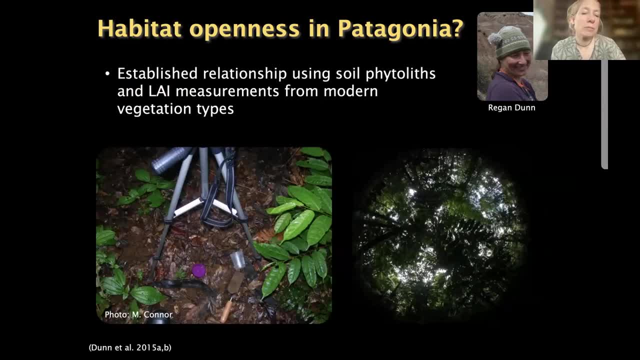 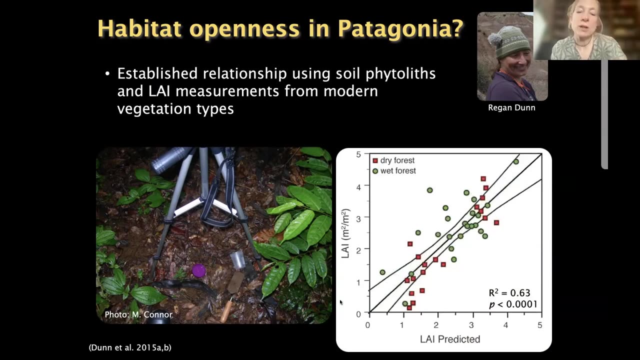 and she looked at soil, phytoliths from different vegetation types there- rainforest and a dry forest- and she also took hemispherical photos so she could measure leaf area index from these photos and then she saw how those things correlated. specifically she saw how the actual leaf area 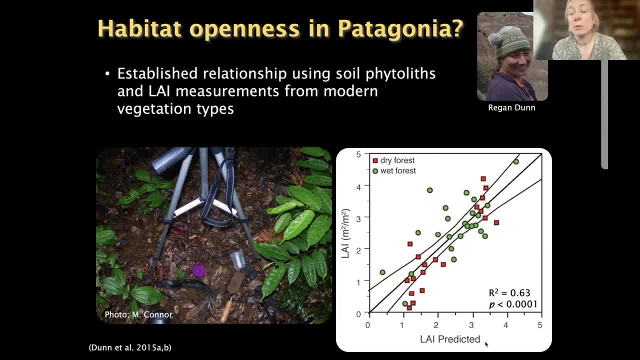 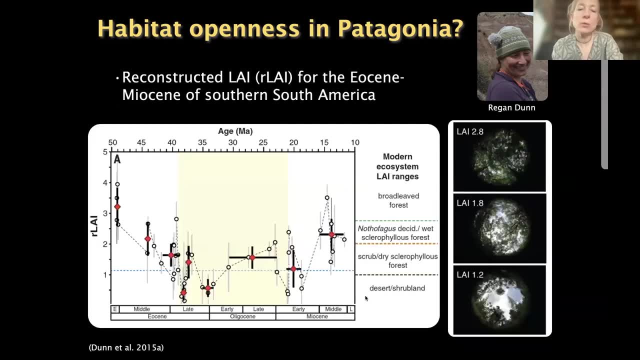 index and correlated with leaf area index, predicted from the shape and size of those soil phytoliths, and she found a pretty good relationship there and so we used that relationship to reconstruct a leaf area index in fossil assemblages from southern south america, so the same ones i've been talking about. 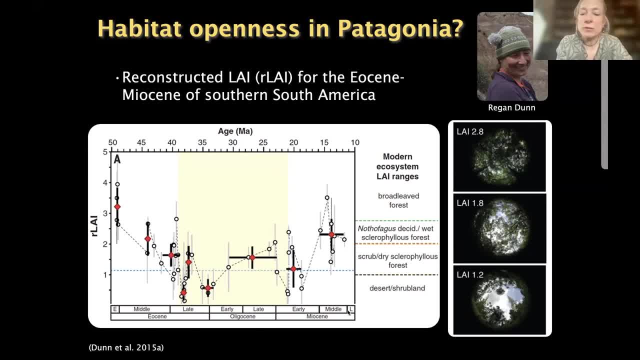 so here we have time on the x-axis, moving forward to the right, and we have reconstructed leaf area index on the y-axis, and here are some examples of typical modern ecosystems that have particular lai ranges, and what we see here is that we, as we go from the early to middle to late. 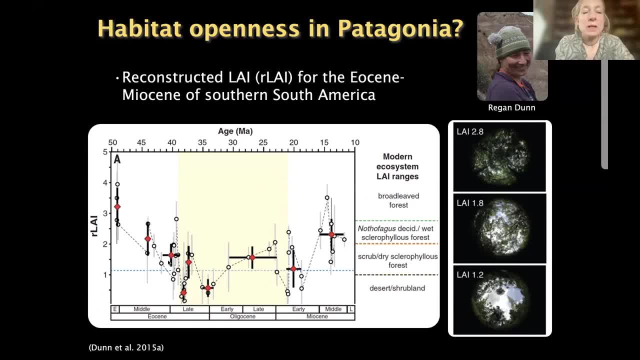 eocene. we see a drop in average lai, so an opening of landscapes down to values that we now associated with desert and shrubland, so very open habitats and for the most part things remain fairly closed until sometime in the middle myosin when we see a regreening, a spread of forest there. 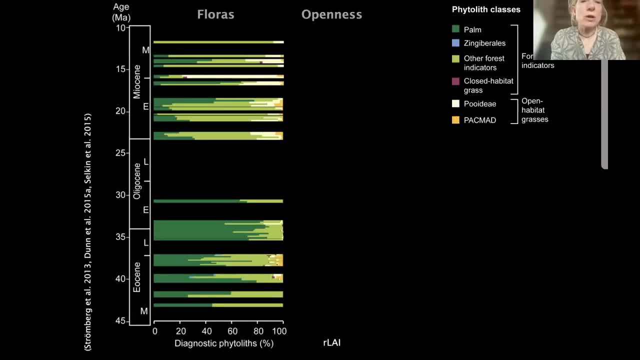 so if we compare the, the floras that i showed you earlier with the measurement of openness, we see that when we reconstructed it, we see that we go from close forest to an open shrubland and because we have a lot of palms here, we reconstructed this as some kind of non-analog palm dominated shrubland. 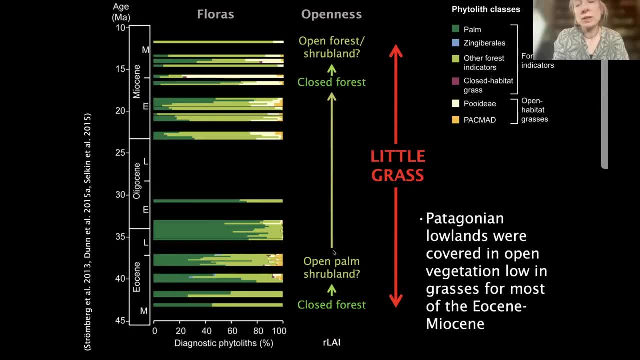 something we don't have on earth today, because palm tend, palms tend to grow in in wetter climates and then it's not until here, like i said, in the middle myosin, that we start seeing some close forest and then again an opening and and during. 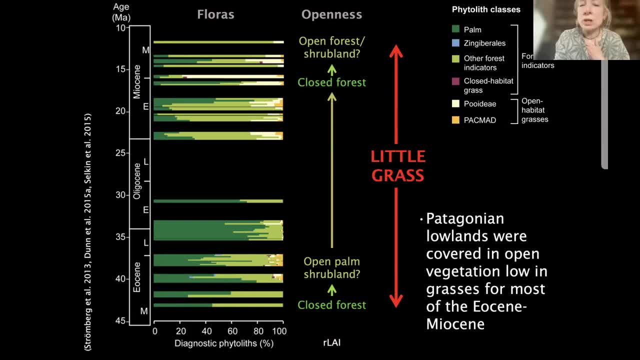 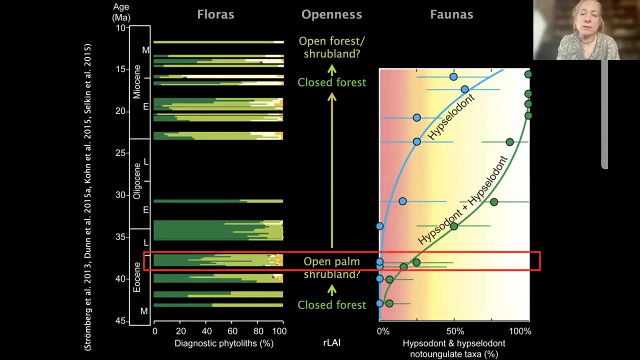 this whole time. like i said before, we tend to generally have very little grass, so patagonian were covered in this open vegetation low in grasses for most of the east scene through the myosin and, and if we correlate this with the evolution of hypsodonti and hypsilodonti. 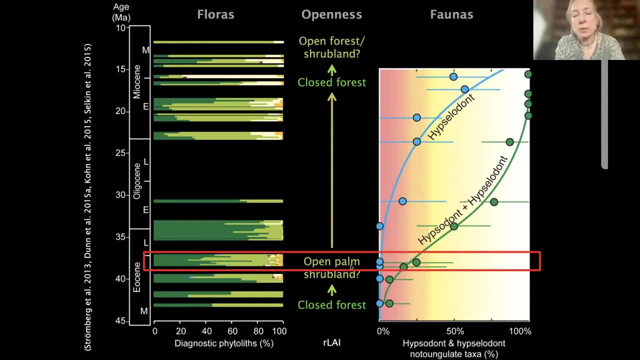 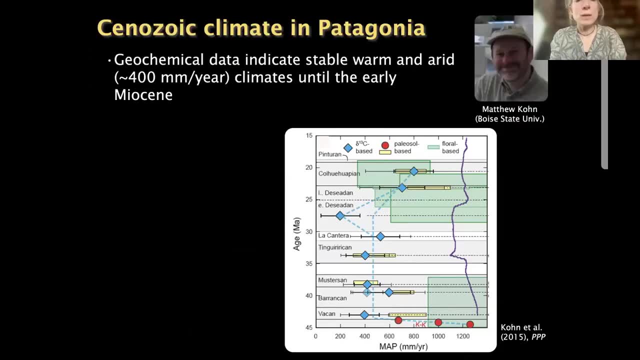 we see that there's a broad correspondence between when we see opening of the landscape and when we start seeing the these hypsodontaxa, and we also had some geochemical data from stable carbon and oxygen isotopes from our geochemist here, matt cone, and basically, to make a long story short, this is such a complicated. 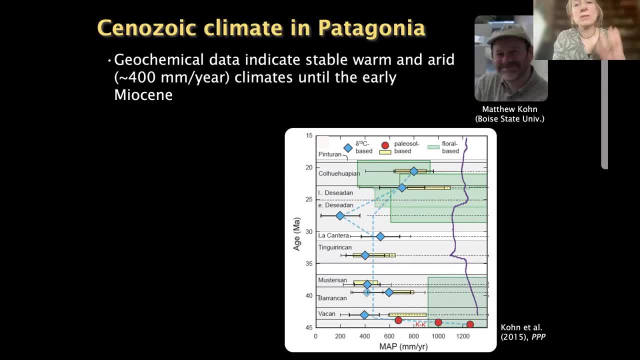 graph, don't worry about it. we found that we had stable, warm and arid climates, starting in the early to mid myosin until the early myosin when we start seeing wetter climates. so we hypothesized then that this, that the opening up of vegetation that we see into these um shrub lands in patagonia might 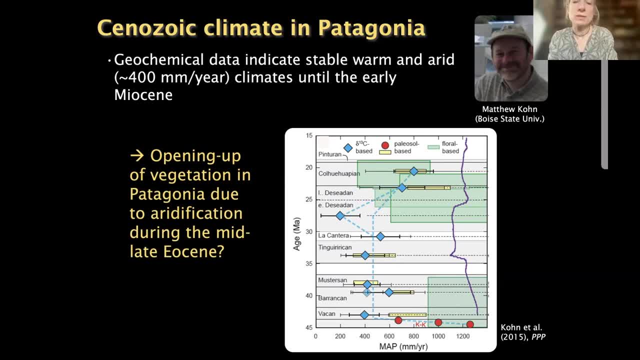 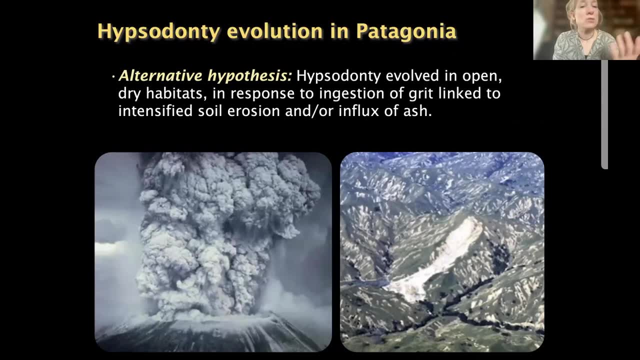 be due to this erodification during the mid to late myosin. so our alternative hypothesis then for hypsodonti is that it evolved in open, dry habitats in response to not feeding on grasses, because there were not that many, but instead ingestion of grit linked to either intense 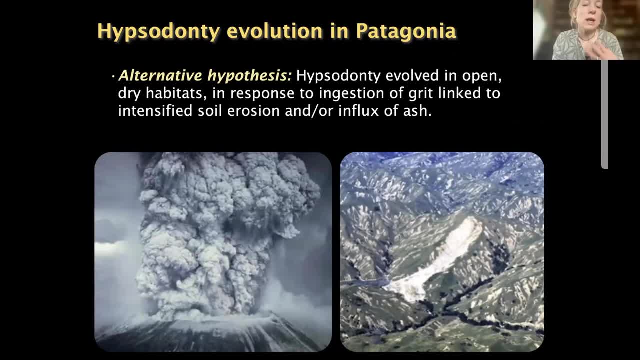 intensified soil erosion or influx of ash and, as i said, in the middle myosin is a very strong habitat and it's a very strong habitat and it's a very strong habitat and it's a very strong habitat and, as i mentioned before, the sediments that we're looking at have a lot of volcanic ash. so 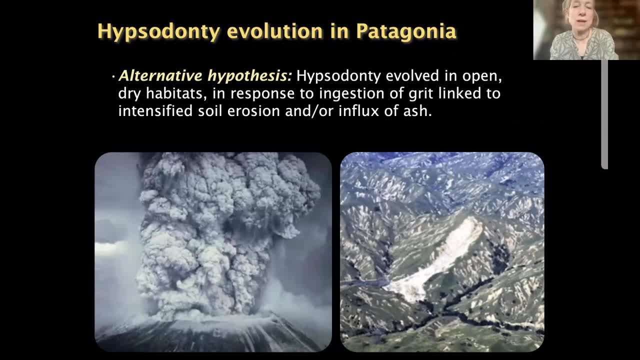 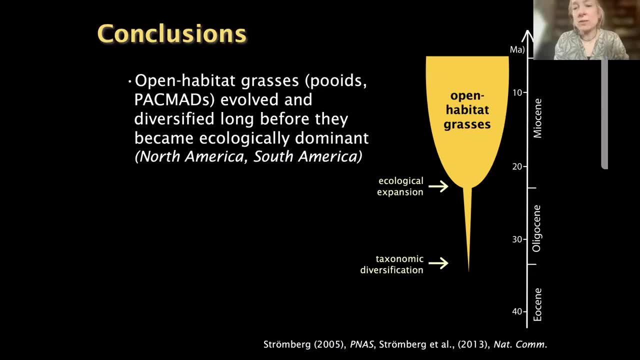 we know that there was a lot of volcanic ash in the environment during this time. okay, so to conclusions from this part here is that these: this evidence from south america is is mirroring what we see in north america, namely that open habitat grasses evolved and diversified. 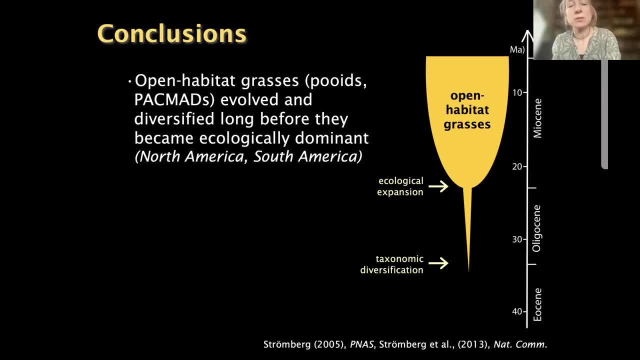 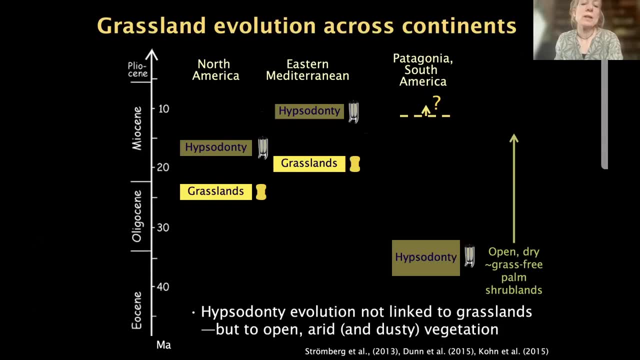 long before they became ecologically dominant, at least in these two different regions, and also that we have a lot of volcanic ash in the environment during this time. so we know that that hypsodonti evolution is not linked to grasslands, but more likely to just generally. 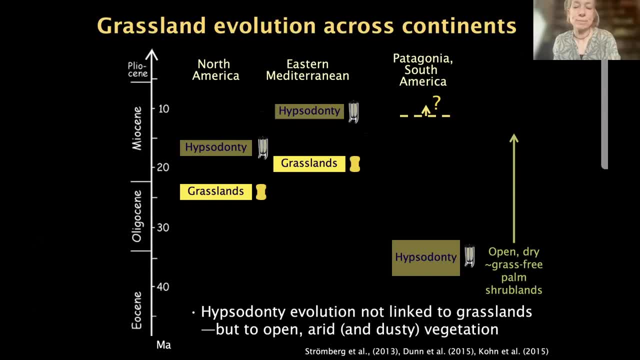 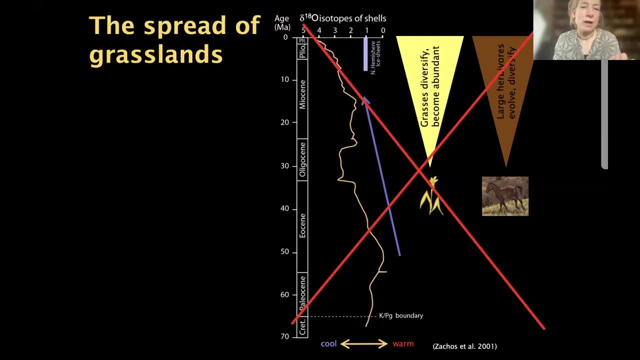 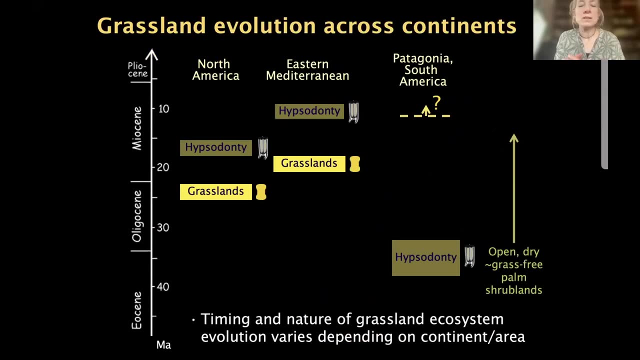 speaking open, arid, arid and dusty vegetation, and i want to say that this, this sort of simple idea of how grasslands are spreading in response to climate, and is not true, but instead we see that the timing and nature of grassland ecosystems, ecosystem evolution, varies depending on the 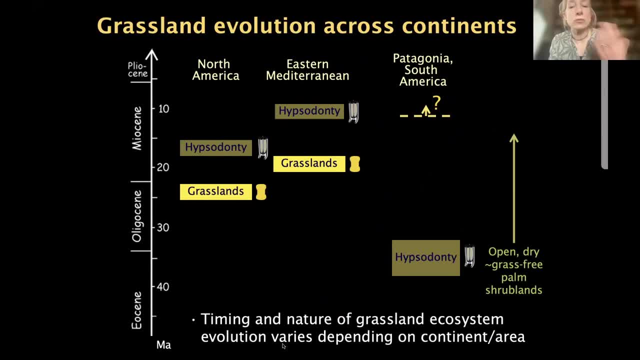 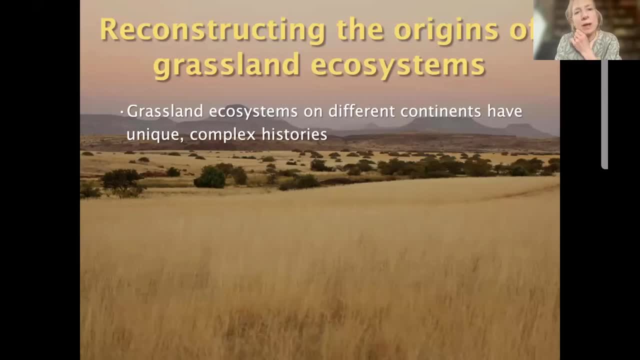 continent and area. so we see that the timing and nature of grassland ecosystems, ecosystem evolution, we really need to look more closely to fully understand, uh, the drivers here, um, okay, so in in conclusion, uh, i want to just re re state here that grassland ecosystems on different continents have 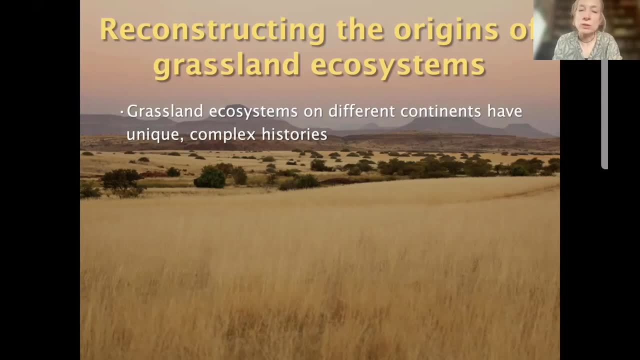 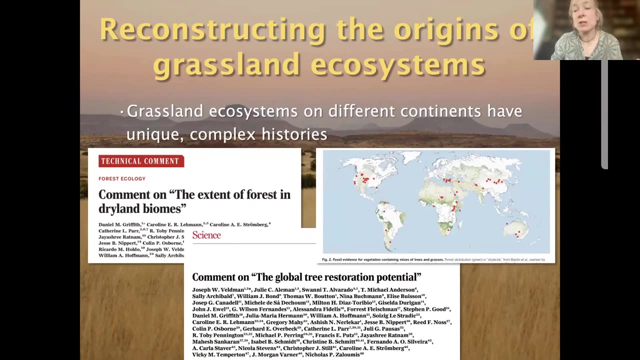 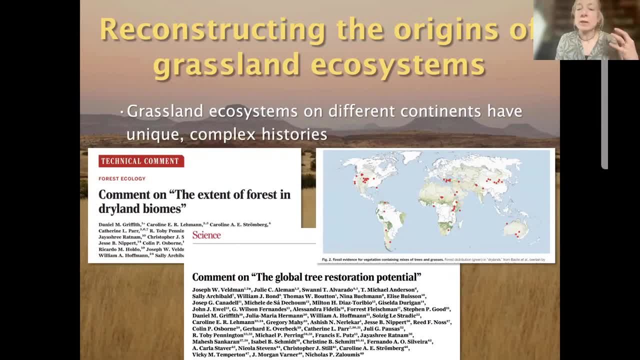 basically plant trees everywhere and and implicit in that- is viewing grasslands as a basically disturbed forest, so not as unique ecosystems with a long evolutionary history. but the work i just presented negates that. it rejects that idea that that grasslands is a very recent thing, but in fact shows that they are are ecosystems with a long history, and that that 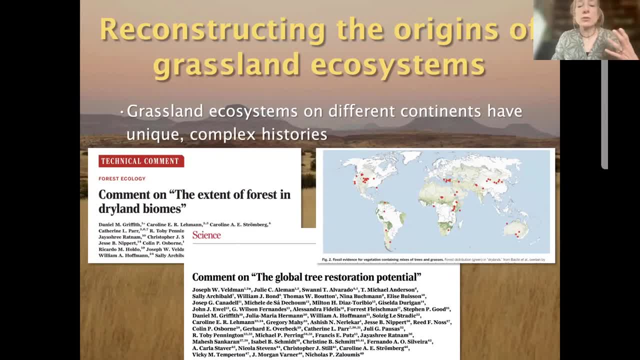 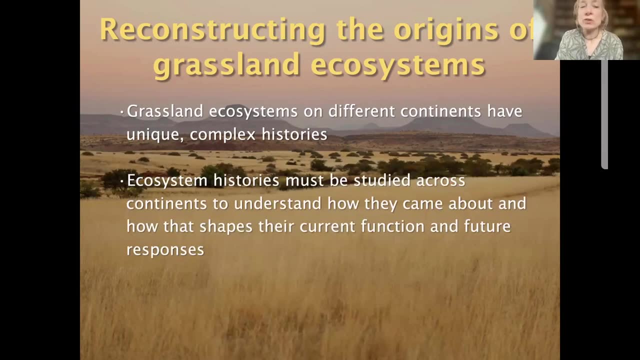 history is something that's important because it has led to the evolution of grasslands and the evolution of unique faunas and, and you know, interactions with climate and all that that i i talked about previously, um, and so we need to continue again study these, uh, ecosystem histories. 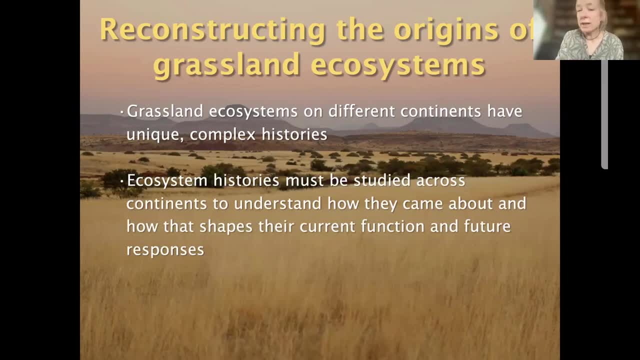 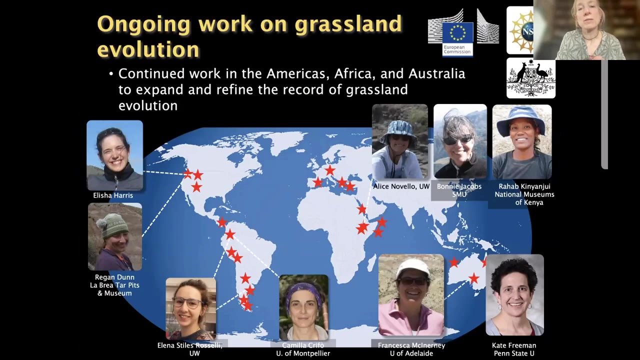 across continents to understand better how they came about, why they came about and how those, those factors shape their current function and and future responses to climate change. so we're continuing to do that and i just want to highlight some ongoing work on grassland evolution. well, just to say that we are continuing to work in in different parts of 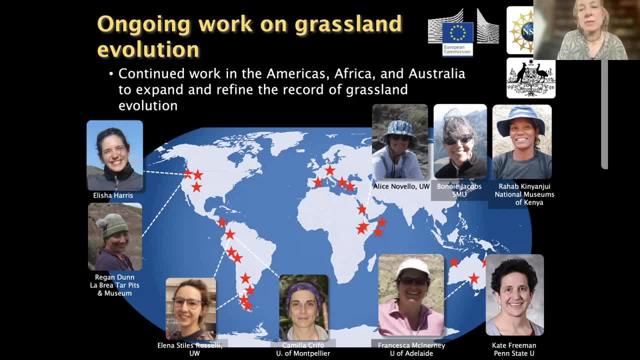 the world to um expand and refine the record of grassland evolution. uh, in the next few weeks hopefully we'll publish some work from eastern africa that i didn't have a chance to talk about. but yes, we need to continue this work to refine and expand the record of grassland evolution. 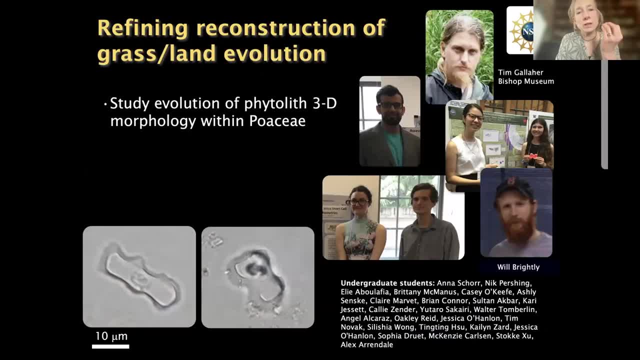 another thing that we're doing is trying to refine phytolith as a paleoecological tool. so right now we can. we can use phytolith to talk about broad groups of grasses within the grass family, but we need to get more specific to to be able to better understand, better reconstruct how. 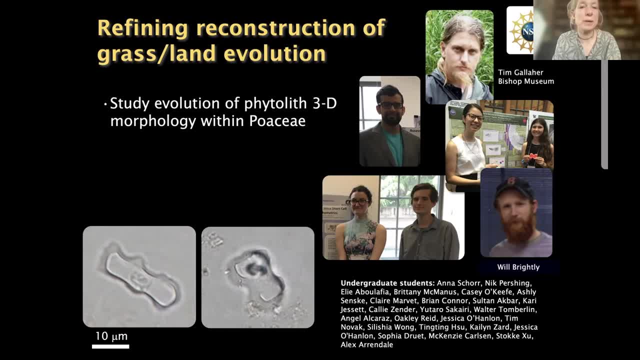 grasses have diversified and and the ecology of of past grasslands. so to do that, and my former postdoc, now collaborator, um tim gallagher at the bishop museum in hawaii, and a whole slew of undergrads and some grass students have been working on this work and they're working on. 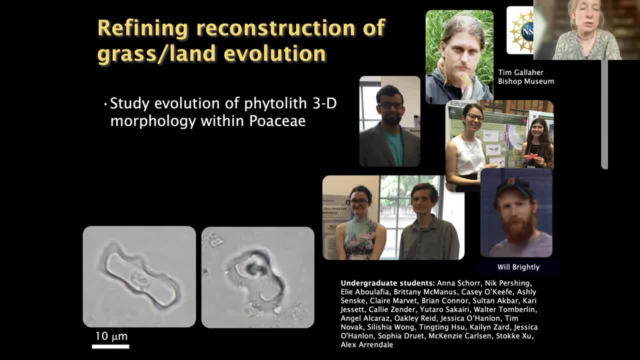 to study the evolution of a phytolith three-dimensional morphology within grasses and we're really hoping to come up with a detailed key, if you will, for fossil phytoliths across poesy. so just to highlight some some of that work. and we have quantified three-dimensional shape like i: 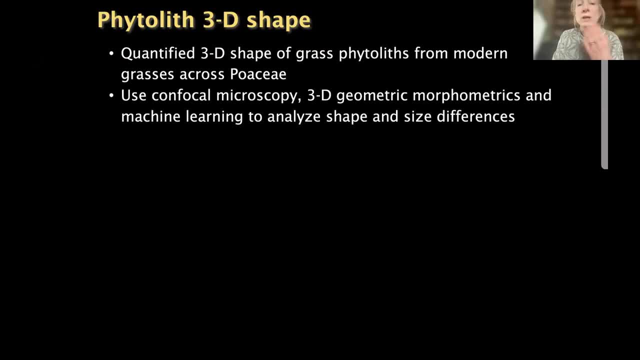 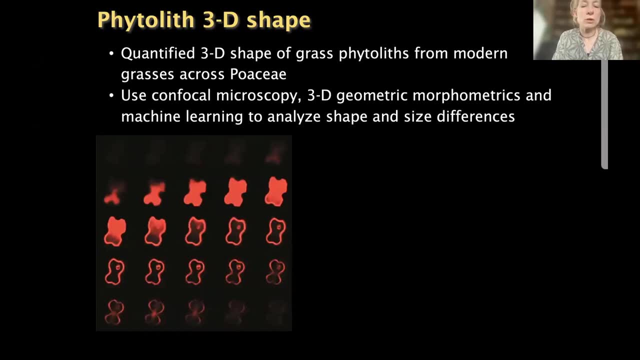 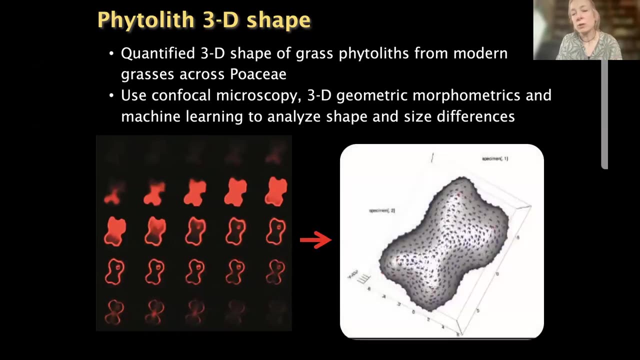 said of grass phytoliths from from modern grasses across poesy, and to do that we use confocal microscopy, which gives you basically pictures slicing through a phytolith, and then we can use different programs to stitch that together to a 3d model. we can then basically measure that. 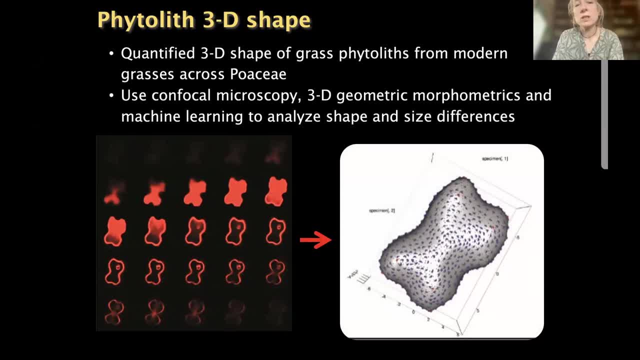 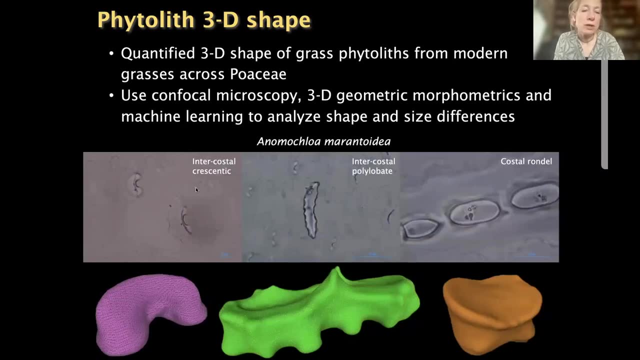 morphology, using something called 3d geometric morphometrics and machine learning to analyze the shape and size differences between different grasses and link that to the group within grasses that they belong to. so to phylogeny- and this is just showing some examples of grass: phytolith in. 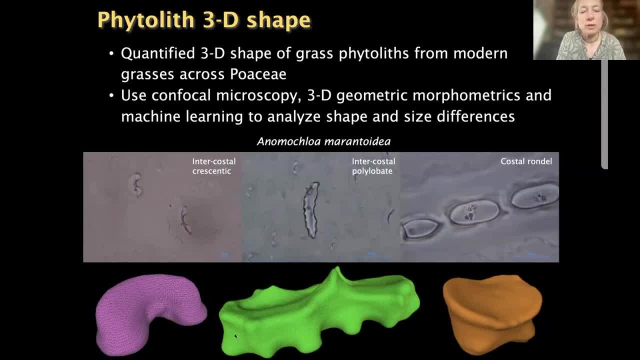 in situ, so in the grass phytolith in situ, and then we can use different programs to stitch that together, and then we can use different models of grass phytolith in situ, and then we can use different models of grass phytolith in situ, and this is what the 3d models look like, and and so we've been able to do this. this is showing a paper. 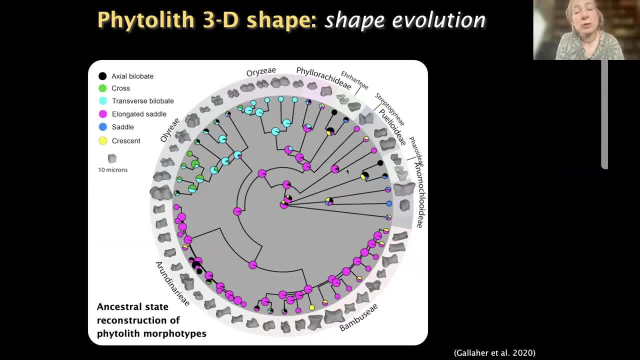 that we published a couple years ago, looking at some of the early divergent grasses and forest grasses, and so bamboos and and rices and things like that, and this is showing these 3d shapes how they map onto a here, a circular phylogeny family tree and and these, um, these pie charts. 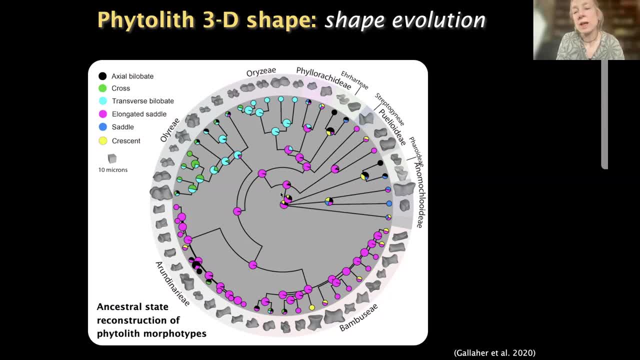 here are showing the likelihood of a circular phylogeny family tree, and, and these um these are showing the likelihood of a circular phylogeny family tree, and and these um these pie charts, nodes, and so what we found is that phytolith shape and size varies with phylogeny and the poesy. 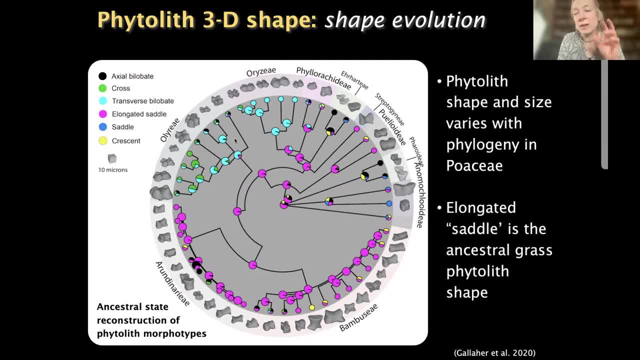 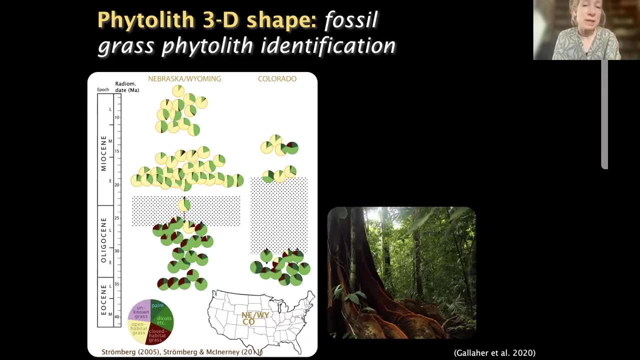 and also we could, we're able to reconstruct the ancestral grass phytolith shape as one of these elongated so-called saddles. we've also- and this is kind of the primarily primary purpose of this is to try to identify and place taxonomically fossil grass phytoliths. 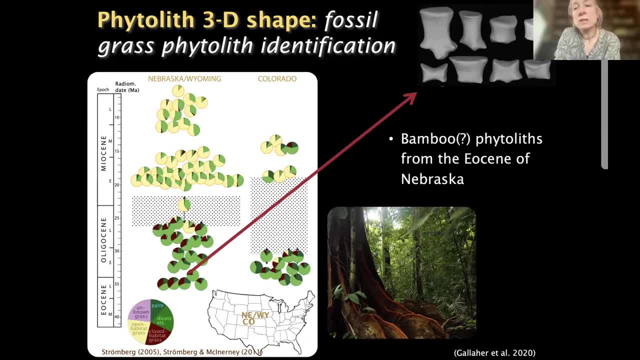 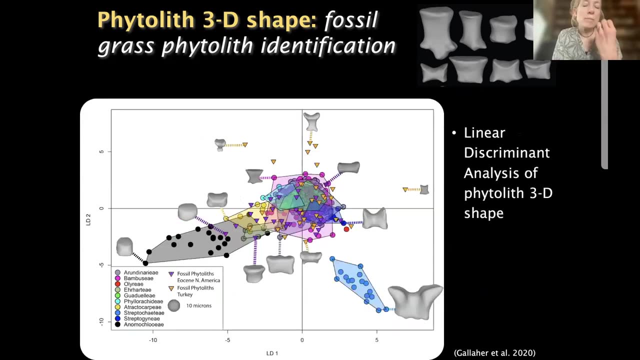 So, as a test case, we took some of these Eocene phytoliths from Nebraska that I had previously determined or hypothesized were from bamboos, and we used our modern data set combined with the fossil data set and we subjected them to different statistical 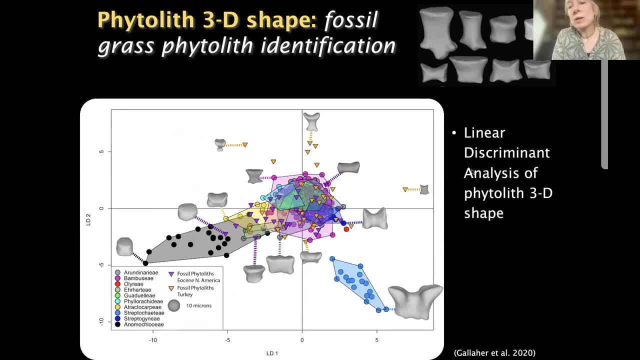 or ordination methods and machine learning, something called linear discriminant analysis. Basically, it is trying to see use statistics to figure out which group of grasses these fossil phytoliths belong to, and what we found was that these phytoliths were indeed most. 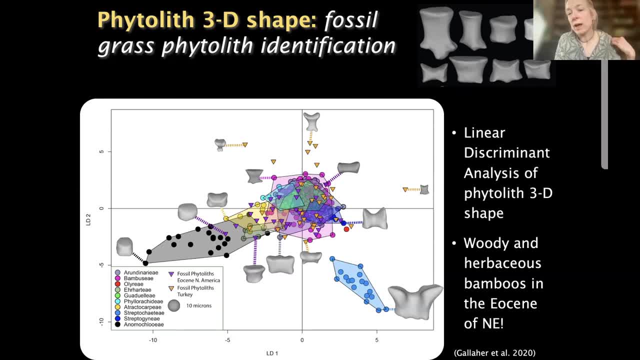 likely woody and herbaceous bamboos that we have there in the Eocene of Nebraska. So basically confirming what we previously thought, but also refining what we previously thought, so showing that there was some diversity in the phytoliths That we found back then. 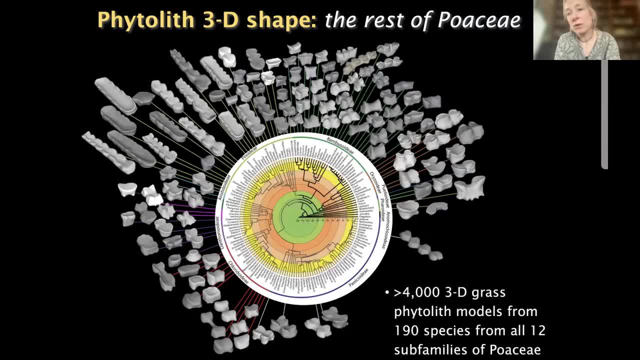 And now we're continuing to look at the rest of the grass family. We have over 4,000 3D grass phytolith models from almost 200 species from across Poesie and we're working analyzing data from Poetie right now and also working with a whole bunch. 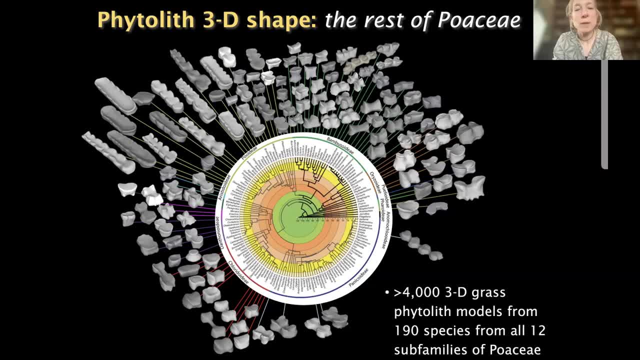 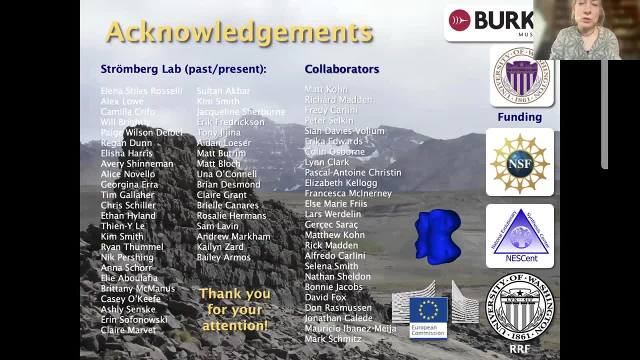 of undergrads again to assemble all the rest of the data for the Pac-Mad clade. So stay tuned. And with that I just want to say thank you so much. Thank you so much for your attention and I'm happy to take questions. 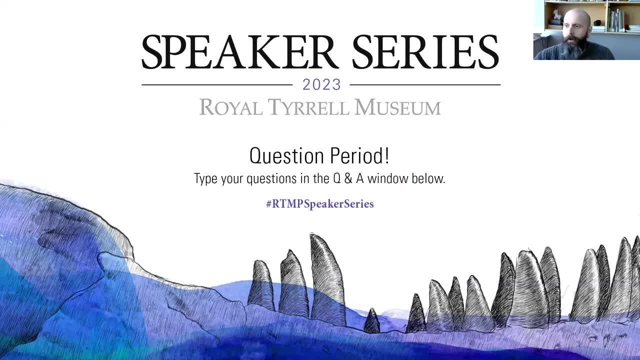 Thank you for that wonderful talk, Dr Stromberg, and we do have a lot of questions, but I'm going to use my moderator privilege to ask you the first question, and it's going to be a simple one. So a lot of early paleoart included grasses with dinosaurs and for a long time afterwards. 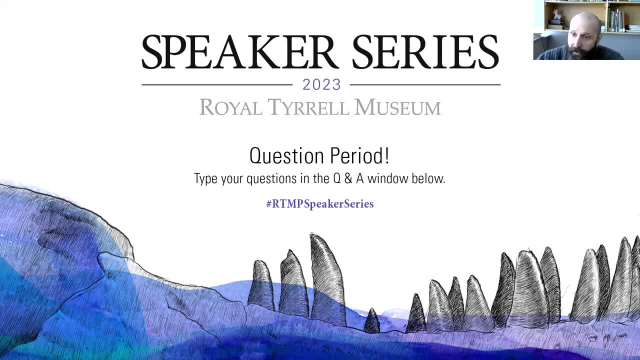 when we understood the fossil history, It was determined that the grasses were in error. but with the evidence of the titanosaurs eating grasses, would you suggest that grasses should be, with moderation, reintroduced into Cretaceous paleoart? 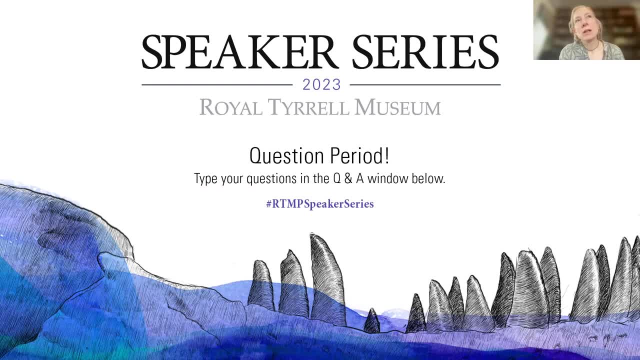 Not. I would say not unless it has been established in a particular place that they were locally abundant, or even You know more than regionally abundant. I don't think there's any evidence that they were regionally abundant anywhere during that. 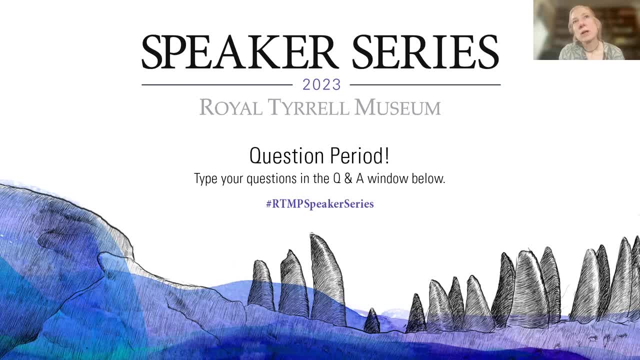 time The you know I said that grass fossils in general are quite rare, and that is true. but we do have what we think are grass pollen. you know, throughout the Xenozoic and you know, in the Miocene, in the more recent, in the more recent times, they are very abundant. 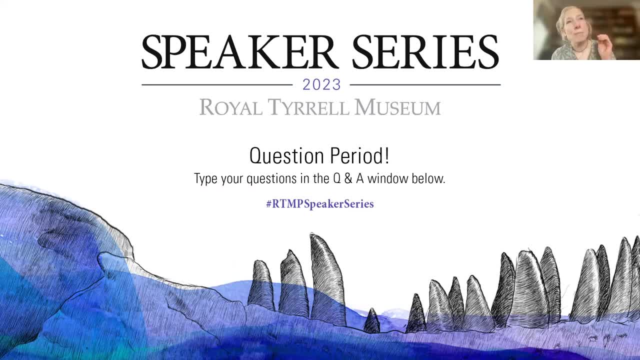 in some sense. So I think if there were abundant grasses in the environment we would have seen them in the in the pollen record. there would have been some indication there. It's possible. some of the more recent work we've done in India seems to indicate that. 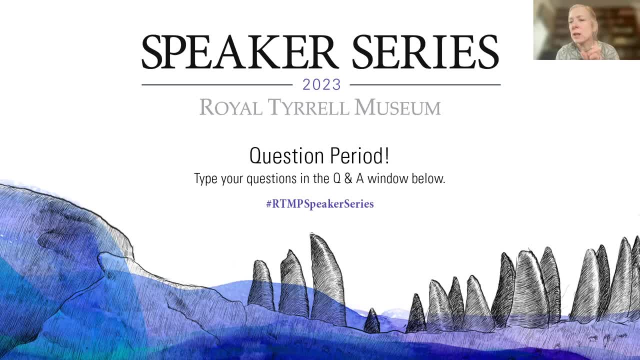 they may have been more abundant right at the beginning of the Paleocene locally, but I would not. I would not assume that they were abundant just because they were had evolved that time. Great Thanks, All right. So our first question from from our attendees has the transition from C3 to C4 and CAM pathways. 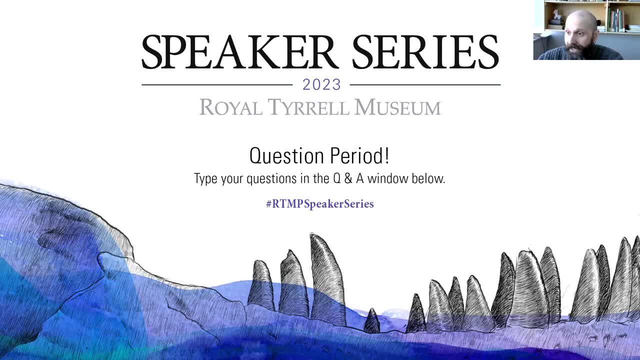 resulted in the widespread advent of grasslands? And if yes, can the increased productivity of the C4 pathway and a lack of the C2 pathway contributed to this Great question? So I didn't talk at all. I meant to not even mention. 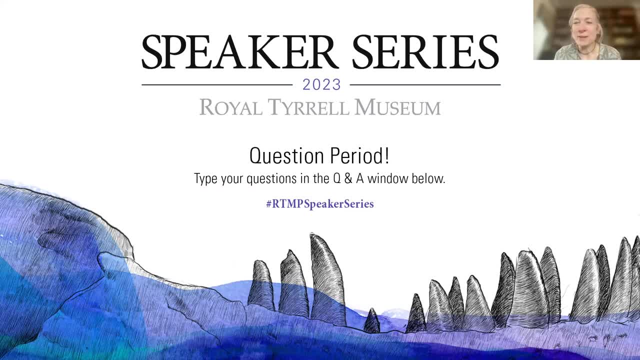 There are different photosynthetic pathways, but I forgot to get rid of the C3 there, but it's a great question. So within, for those of you who don't know- within the Pac-Man clay, these tropical grasses, we see the advent of this C4 photosynthesis, maybe as many as 30 times independently. 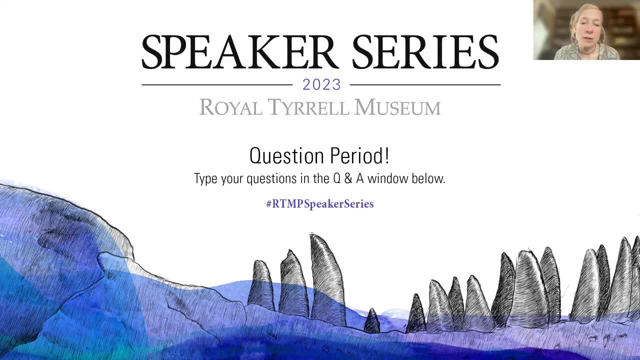 And C4 photosynthesis is very advantageous in hot and dry climates, with summer rain in particular, and at low CO2, low CO2 levels And so So so it's often been thought that you know C4, okay, So there's that. 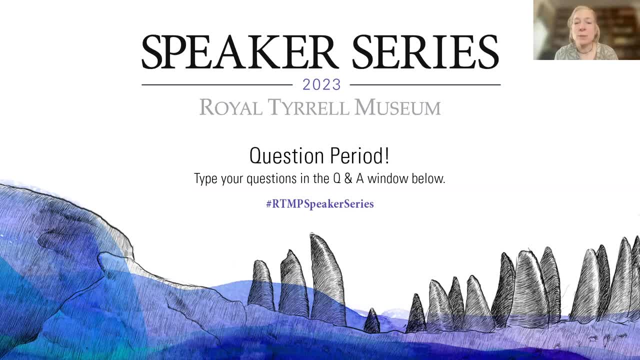 Then also in the fossil record, using geochemistry, using stable carbon isotopes, we can see when C4 grasses become abundant, because C4 grasses have have a different isotopic signature compared to C3 vegetation. So C3 is the ancestral photosynthetic pathway that most plants have. 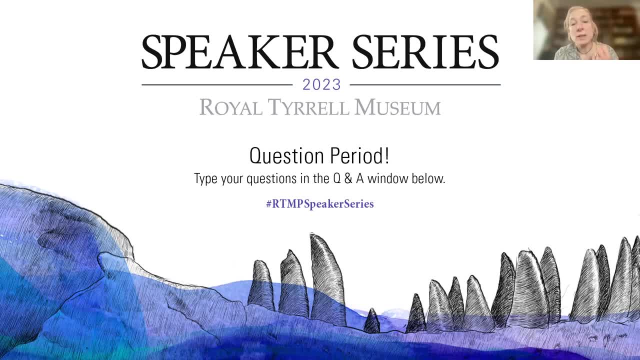 And so people, people often assumed that the evolution of grasslands was synonymous with the spread of C4 grasses. but now we know, based on phytoliths, and I should also say implied also by hypsodontae, but definitely shown based on phytoliths- that prior to C4 grasslands in many regions, we 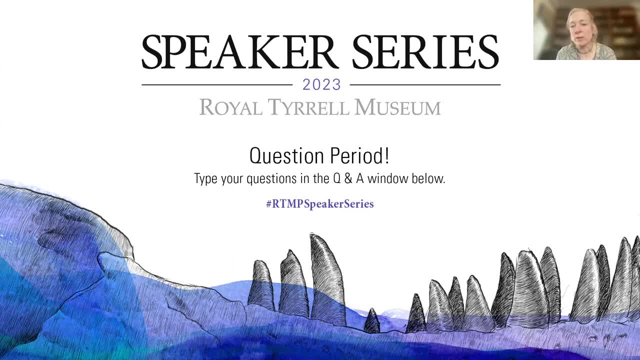 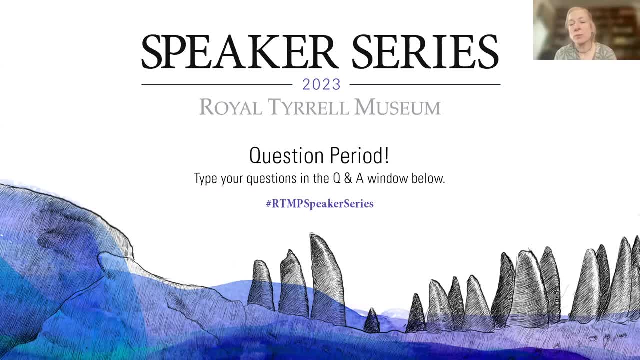 grassy, And one of the things I showed you was the evolution of grasslands. there are grassy biomes by, say, 22 million years at the latest, And then it's not until five to 6 million years ago that we see the spread of C4 grasses. 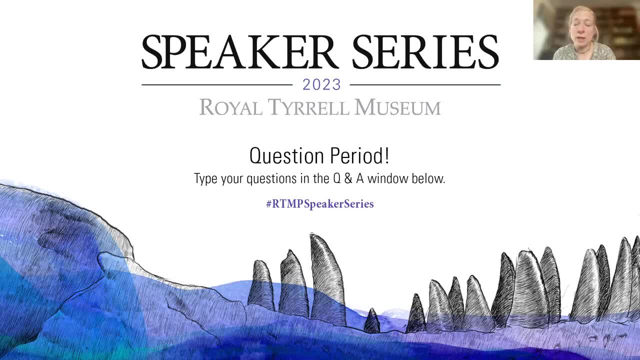 in North America. So there's a. there's a lag there where you first had C3 grass dominated habitats and then some C4 grass dominated habitats In other, in other continents. there's less of a lag, but there's often. some indication- pollen or phytoliths- that there was C3 grassy habitats appearing first. Not everywhere necessarily, but in some regions, So they're not necessarily synonymous. Great thanks, Yeah, I think that covered it. Is there a functional reason for the difference? 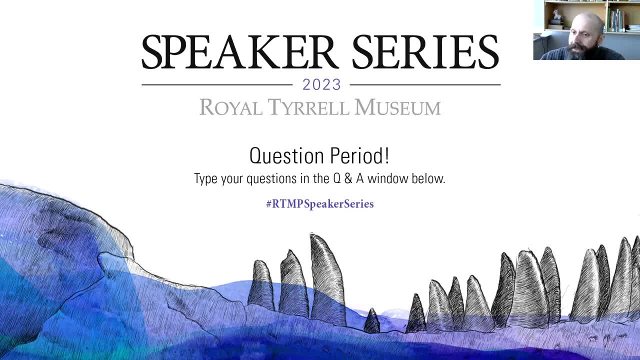 in phytolith shapes between different plant groups or families. Well, great question. So, if we think outside of grasses, oftentimes those phytoliths are a direct reflection of the types of cells, because they're basically infillings of those cells. 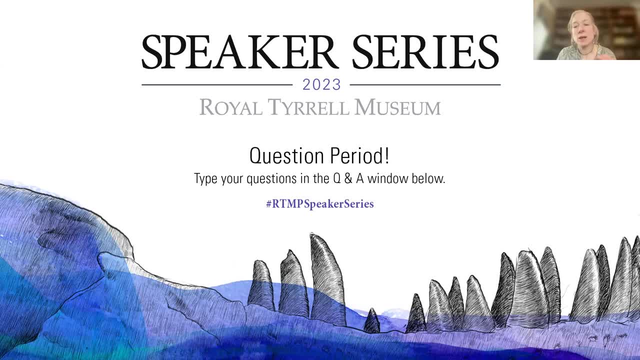 And that's why they're less diagnostic outside of grasses And also that kind of kind of the function is just basically tied to the function of the cell. So you can have in the epidermis, you can have stomata, so the pores, they can be salicified, You can have the vascular. 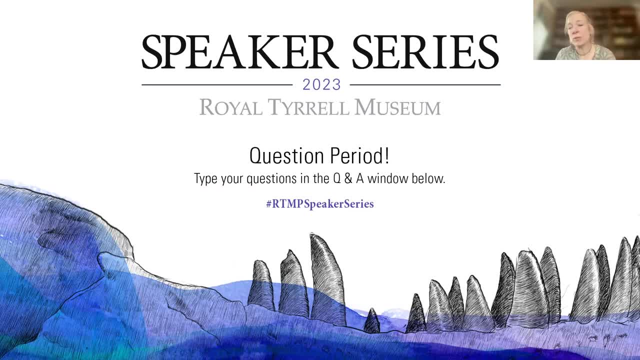 tissue being salicified. You can have regular epidermal cells, You can have hairs being salicified, So those are just. you know, there's no function outside of just what: the cell, the function of the cell. So within grasses we see shapes that don't seem directly tied to the shape of the cell. 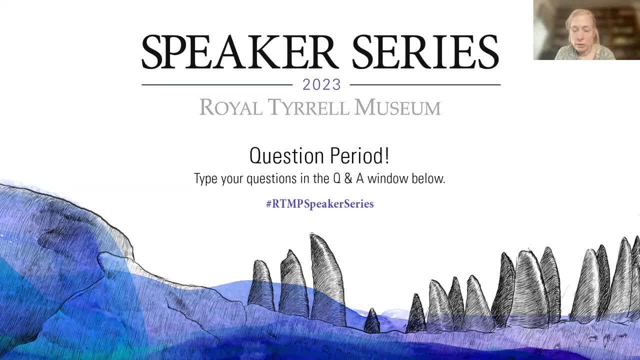 They're sort of independent of the shape of the cell, And that's where people have talked about potentially different functions relating to the shape. So there's some that are very elongated, some that are short or like, yeah, bilobate shape and things like that. There's no great. 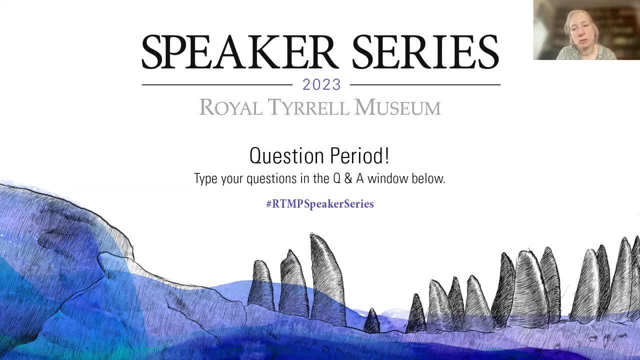 sort of strong hypothesis I would say at this point. about the shape. The most interesting, compelling thing I heard was when I talked to a structural geologist who suggested that the phytoliths that are long and sort of like have sinuous margins or like wavy margins, that maybe they are similar to. 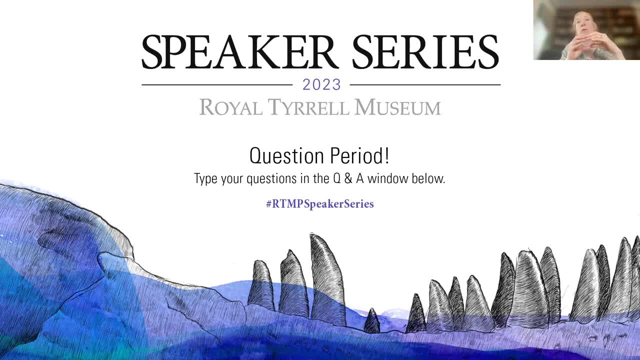 how minerals behave in metamorphic rocks when there's like a lot of tension. They tend to be sort of, I forget, budino or something like that, what it's called, And so he suggested that maybe they have that shape to strengthen the grass leaf when there's a lot of wind or other sort of forces moving the leaves. 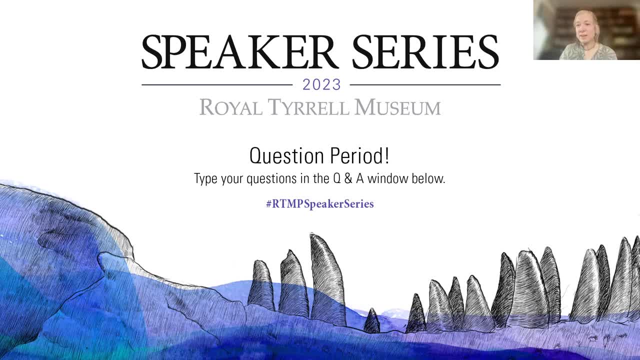 And that is fascinating, fascinating suggestion that has not been tested, But other than that, yeah, we don't know. So for most plants outside of grasses, the phytoliths are simply when silica rich water is moving through the plant. 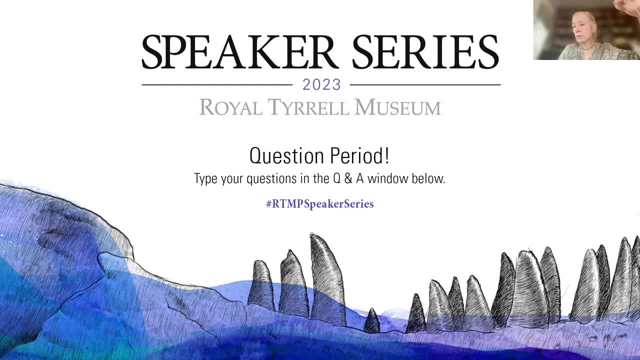 And so, yeah, no direct function of those phytoliths. Great. So there's a follow up question to that one and you've already answered it partially. So the follow up question was: are the phytoliths purely an anti-herbivore measure? 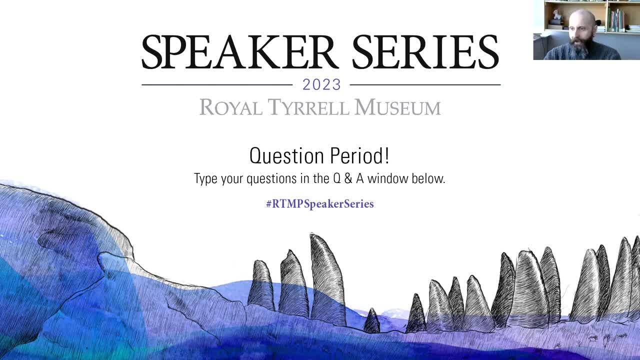 Or do they serve other purposes? So you've already touched on that. But the sort of extension of that is: does their abundance in plant tissues or their shape tell you anything about the predation stresses that the plants are being subjected to by local herbivores? 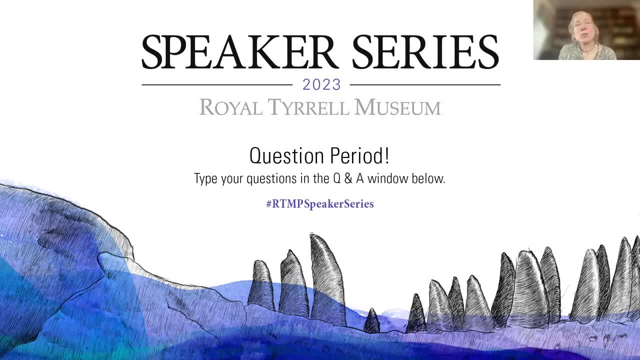 Also a great question and something that we've done some work on, And so we did some work where we try to map onto a phylogeny the abundance, like the relative abundance, or the concentration of silica and tissues both across land plants as a whole. 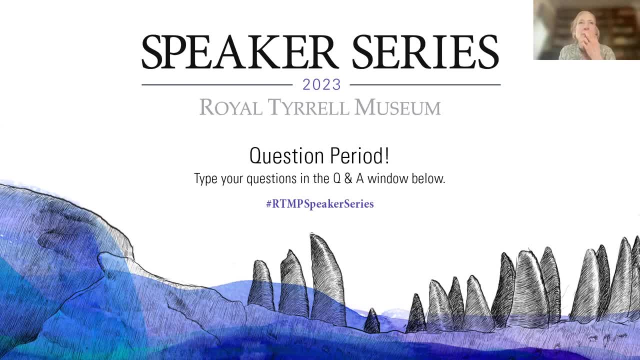 and then focusing in on grasses. Indeed, silica has been proposed as an anti-herbivore defense, And so you would expect to see either silica being increasingly deposited within a group of plants that's subjected to, that's co-evolving with herbivores, say. 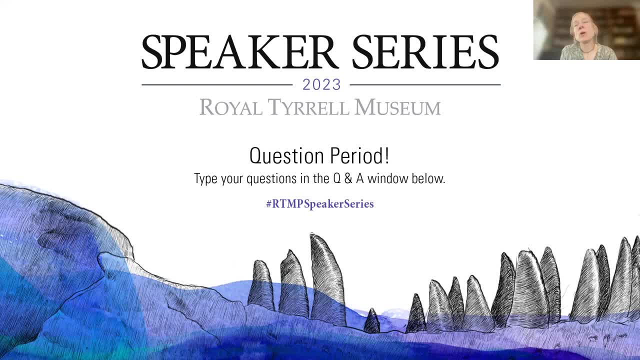 so grasses would be an example of that. Or during certain time periods, like, say, when we see the advent of these tooth batteries in some dinosaurs, that they maybe were feeding on abrasive things. Yeah, And so far we have not been able to see any patterns. 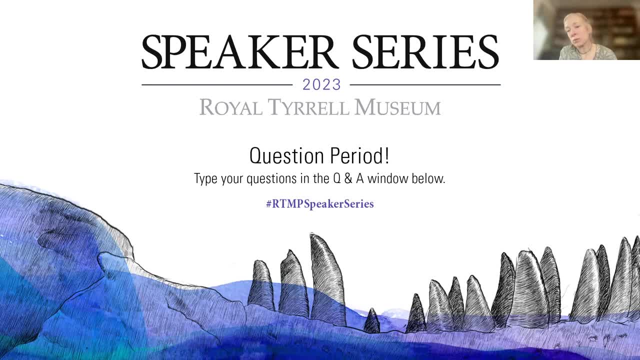 of silica deposition in plants that support those hypotheses. If we look broadly on plants, I think we just don't have enough data and enough precision in when Silica evolved. So silica deposition evolved probably was present or possible with early land plants onward. 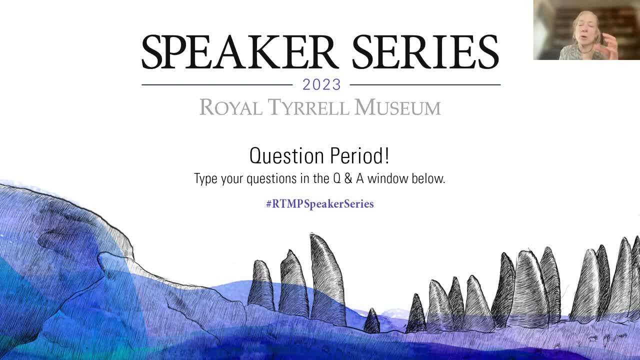 but we'd see it sort of becoming more abundantly used within different plant groups at different time periods. So it's not that all plants are just doing it a lot or a little, but there's sort of certain groups within, say, flowering plants or within conifers or whatever. 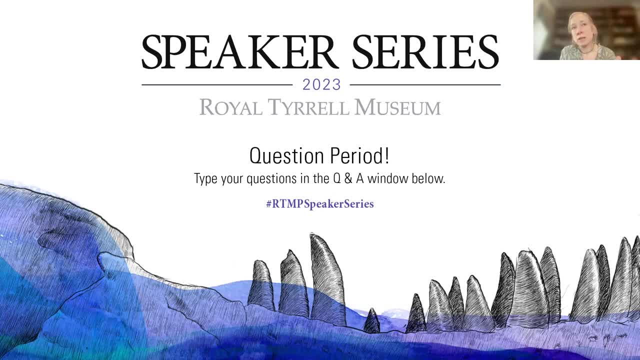 that are depositing more silica, But so far we don't see any great patterns there. If we look within grasses, we also don't see patterns of increased silica deposition, for example in open habitat grasses, which we think we're interacting with herbivores. 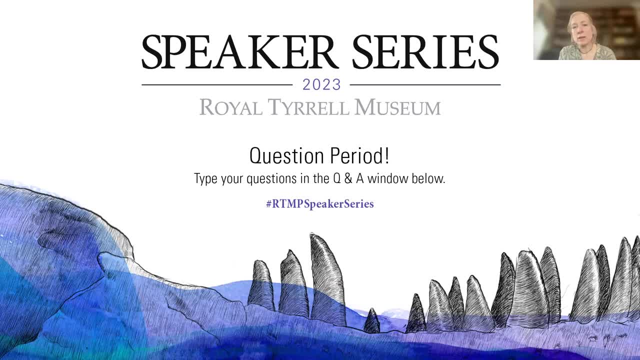 in a more sort of meaningful way than a forest grass. Forest grasses are just not abundant enough to sustain a lot of herbivores, So it's not. yeah, we wouldn't expect to see that, But we don't see those patterns. 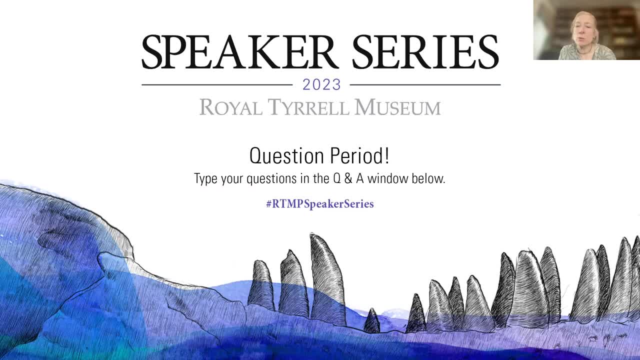 We see instead that silica deposition seems to be more linked to the climate. So in a climate with a lot of evapotranspiration, so a lot of water is being moved through the plant because it's dry and a lot of evaporation. that's where we see more, higher levels of silica. 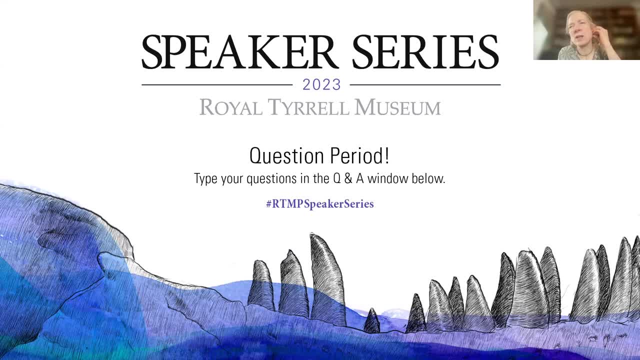 So it seems more, you know not necessarily that there's, there was selection from that for that, but maybe it's something that's happening, you know, in the plant, in each individual plant, that they're basically sort of passively taking up. 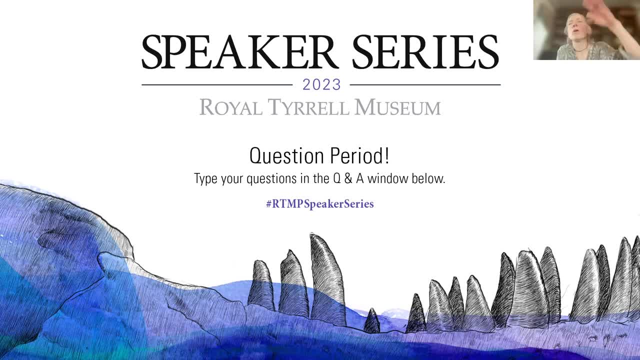 a lot of water, sorry, a lot of silica, because a lot of water is moving through the plant body. Sorry, that was maybe a little bit confusing. The short answer is it: you know, I, we still think that phytoliths are an anti-herbivory defense. 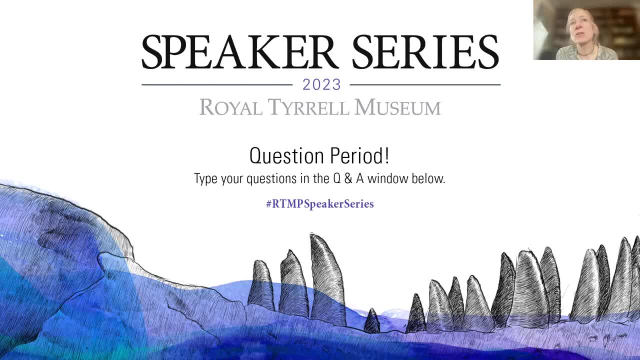 but we don't think that it was an anti-herbivory defense to large ungulates, more likely to insects, And that is a lot harder to test because we don't have a good fossil record of insects. So yeah, that's something that needs to be looked at. 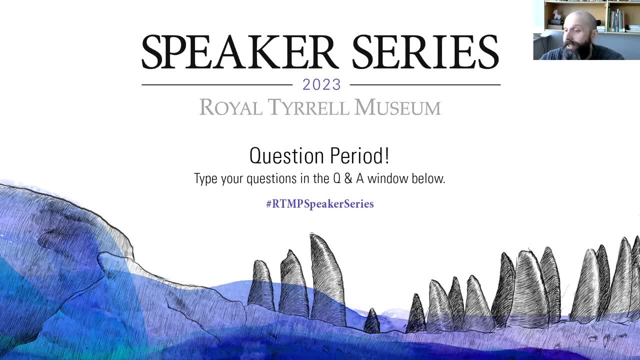 Great, Okay. So the next question: have you or has anyone carried out a study of phytoliths to understand herbivore diversity in regions like China or Russia? Hmm Well, Russia, I don't think. so, I don't think. I mean, certainly we haven't. 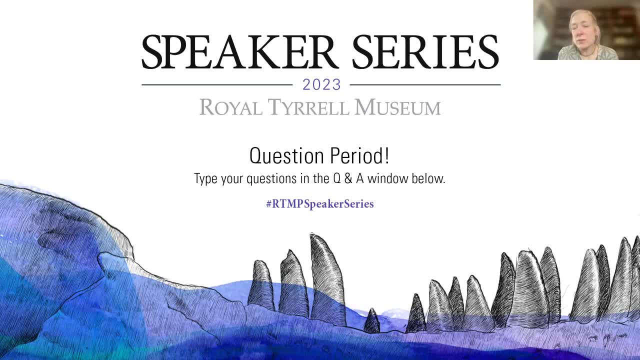 and I don't think there's anyone working on the timescales, sort of like, you know, deep time the way we are In China. I have actually tried to find phytoliths in many, many sediments and have been unsuccessful, except in one place. 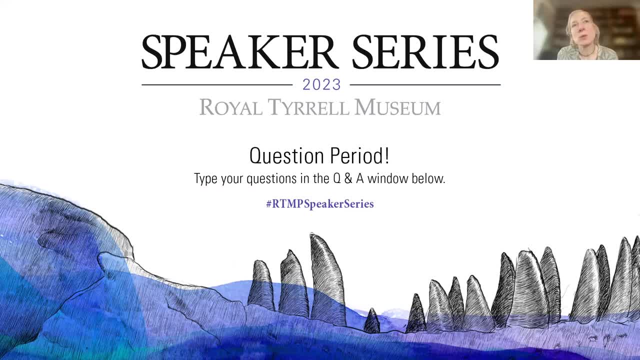 but it was just one lake And so can't really address that question with just one place And I think there are some, I think there was. I reviewed a paper once that was looking in. I think it was Mongolia, Inner Mongolia or Tibet. one of the three where they had a record of phytoliths, But I don't know whether it got published Anyway. so the short answer is there is that there is work ongoing looking at that, But I don't think that that paper directly compared it to herbivores. 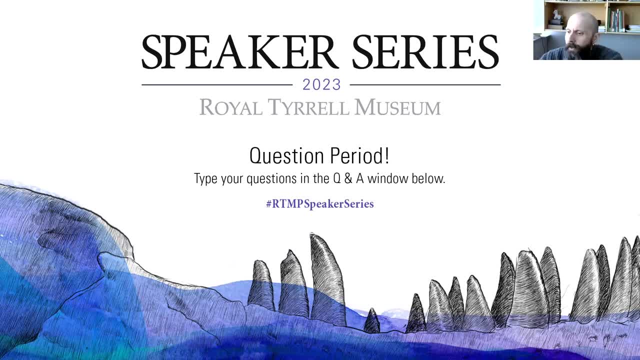 And yeah, Okay, great. Do you see any relationships between phytoliths in the fossil record and the incidence of wildfires? Hmm, This is a question I'm hoping to answer in collaboration with folks at well, Alison Carp and Kate Freeman, who are our geochemists working on. 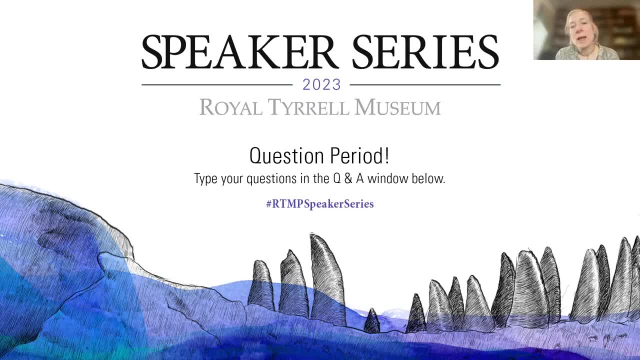 different ways to look at fire in the fossil record, And the short answer is that we haven't. we don't have a record where we have both phytoliths and those kinds of fire indicators. That said, we are making them. for example, 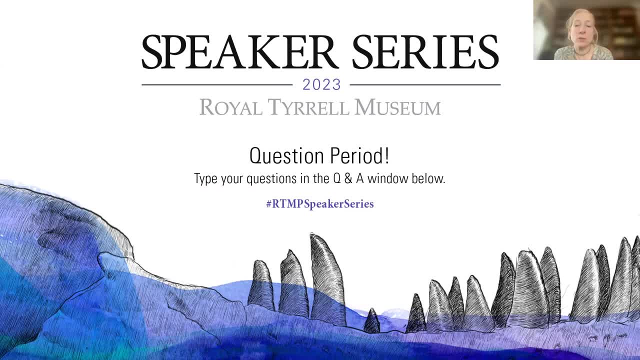 I'm working in Australia and there we can make those comparisons, And we we just haven't even really began the the phytoliths counting yet, for that There is also we have, because phytoliths are affected by fire. 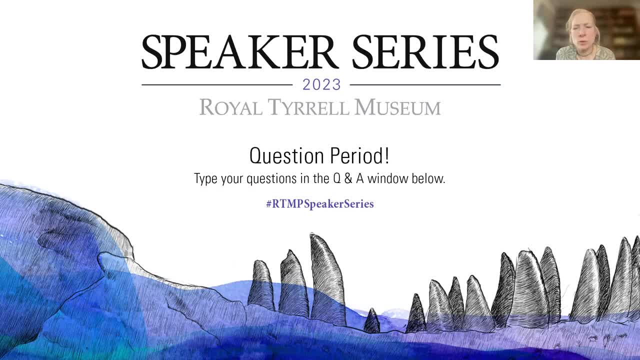 So they they get black and slightly deformed. So we have used it in Patagonia to look at fire across the Eocene-Oligocene boundary, where we saw that there was a change in the fire regime, or we inferred that there was. 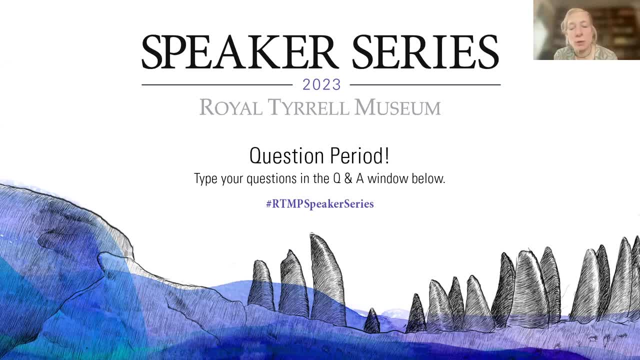 a change in the fire regime, looking at phytoliths and some other geochemical proxies. so, um, we don't, we don't know yet. uh, we just have haven't reconstructed the record from australia, for example, to say what the relationship is there. uh, however, i will say that the record from from 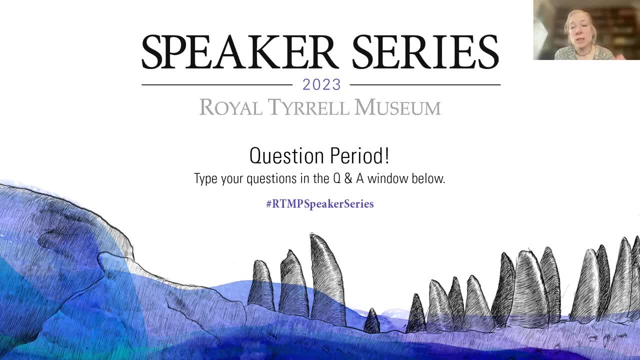 australia, looking at pollen, and these fire indicators indicate that the fire regime there, which is very strong, was established before grasses and even and long before c4 grasses. so there there's probably not a strong correlation. but in other regions i expect there are, for example, in, in, in in india, pakistan. i think there's a reason to think that, but yeah, great. 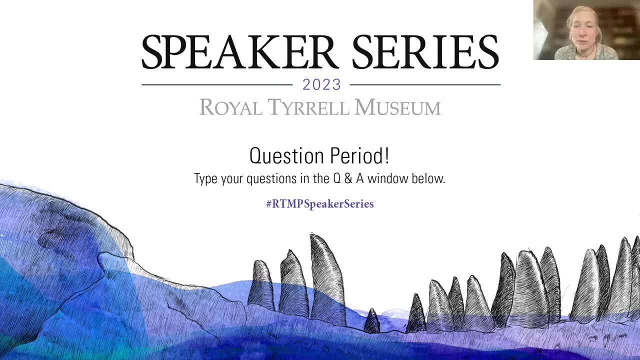 uh, do you have time for a few more? yeah, yeah, sure, yeah, sorry that i'm a long winded. no, uh, can you comment on the biogeography and the distribution of extinct members of poesy in the cenozoic, and can that information at all be used? 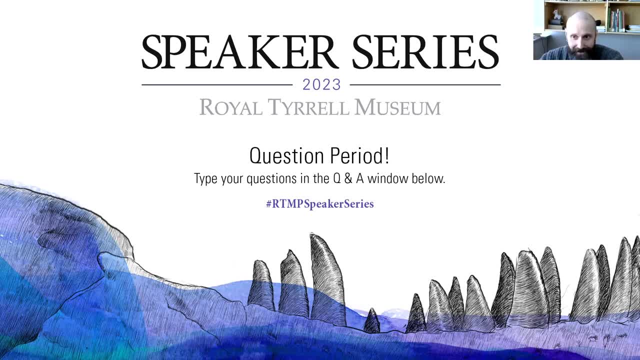 for the future of agricultural practices. so i, the short answer is that i think, generally speaking, uh, we, we will be able to say something. uh, like, i was talking about understanding a little bit about um sort of the ecologies of of different taxa, the, the how, how, the, the distribution of of 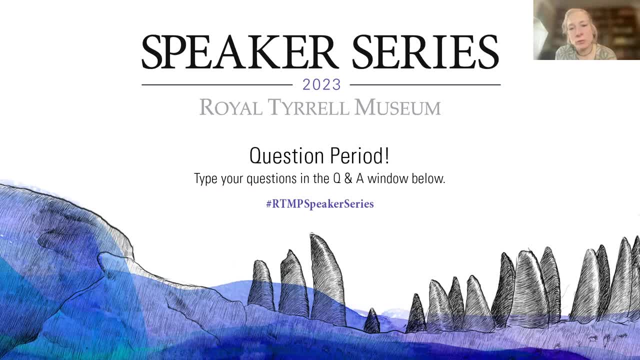 different taxa with certain ecologies have changed through time, can maybe tell us about the the breadth of those ecologies? so right now we have grasses, certain grass groups living in different habitats and in different climate zones and whatnot, and so we are. we then assume that that is, that is their climate regime, that they are are most adapted. 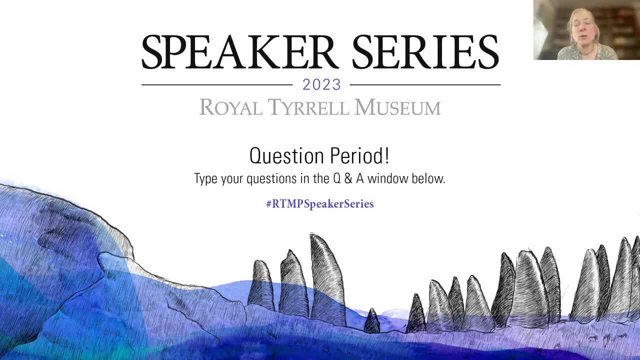 to, and and that's the kind of habitat they are most adapted to. but in the fossil record, if we find that we find these lineages or these groups of grasses in different climates and habitat types, that might tell us that, uh, they, they're their fundamental niche, if you will like so. 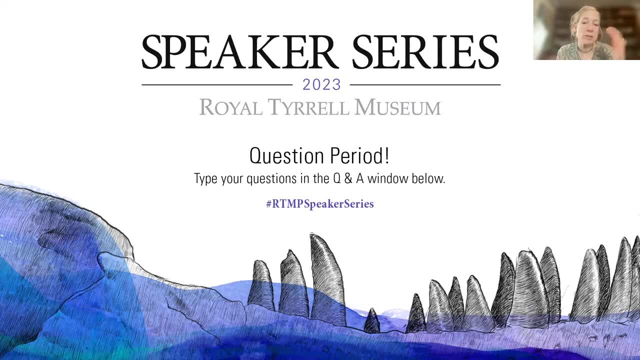 where they can live is actually much broader than what we see today, then that is helpful, i think, for for being able to analyze what's going to happen, uh, with, with crops, for example. of course crops are, are very altered from their um, from their ancestors, um, in in like genome duplication and all kinds of selection happening, but the, the. 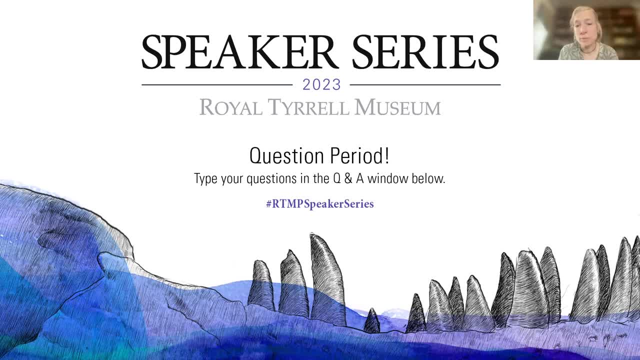 fundamental things, so like c4 photosynthesis in corn, for example. we don't know exactly why c4 grasses became, uh exploded onto the scene very late in the miocene, as opposed to earlier in the miocene, or or even a legacy nor eocene when c4 photosynthesis evolved, and so we're trying to 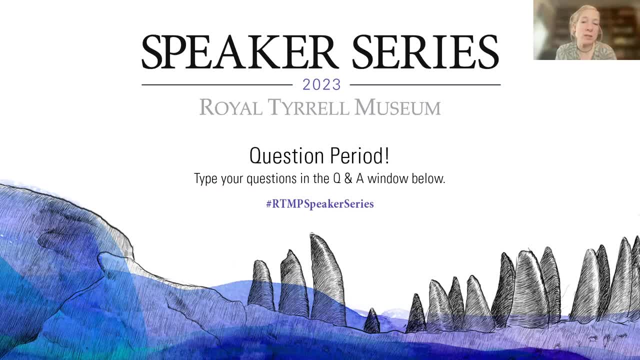 figure out what were the factors that made it advantageous to be a c4 plant. if we can determine those factors, we know, we know more about uh what to expect um in terms of where c4 grasses can grow productively, and so that will be directly informative for um agriculture. i think great, uh, we'll do, we'll do one. 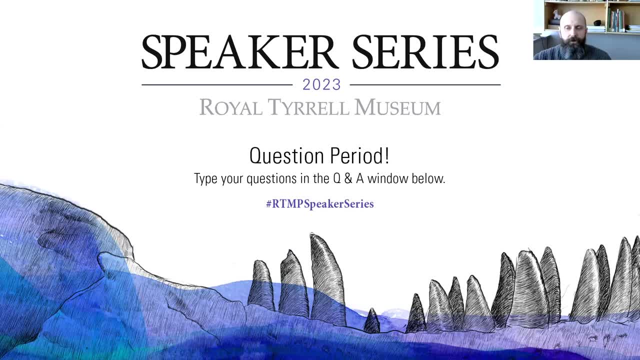 more and then we'll let you go. um, do you have any ideas or have thought about creating a theoretical morphoscape using phytoliths, based on mathematical frameworks similar to those done on foraminifera? um, i, i? i think the answer is yes, in a sense that that's a little bit what we're trying to do. 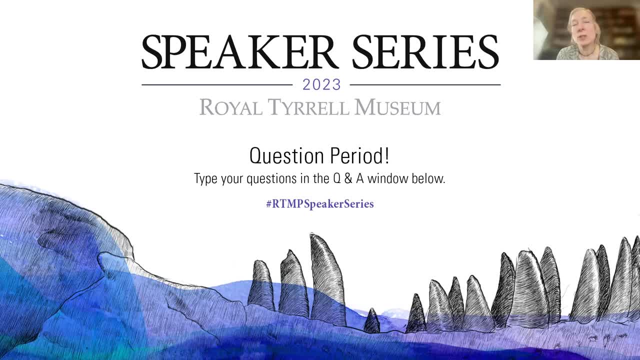 with with this 3d work that i mentioned. i don't know exactly what um sort of what the morphoscape for forums is. i don't know like, is it sort of looking at evolutionary adaptive peaks or something like that, or or sort of, uh, just looking at how the